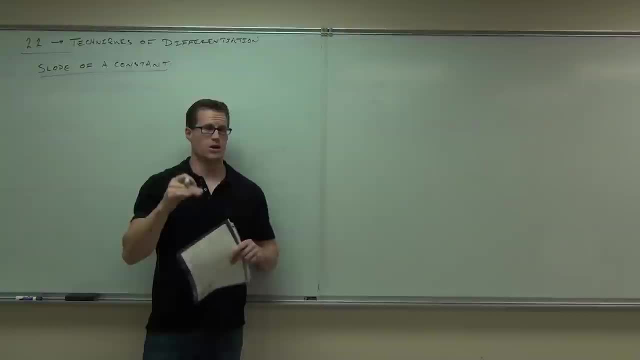 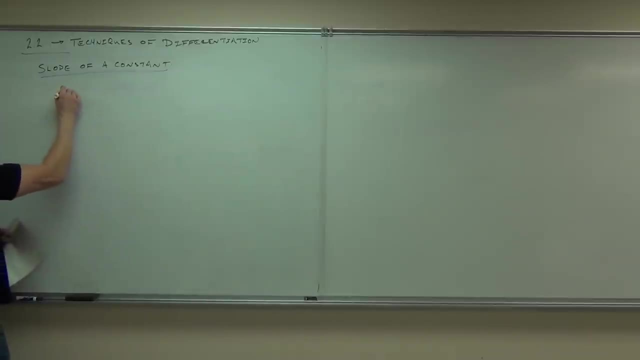 Do you get a horizontal or a vertical line? Which one? If you graph a constant: y equals 5, what do you get? It's not vertical, right, That would be. x equals a horizontal line, at whatever your constant happens to be. 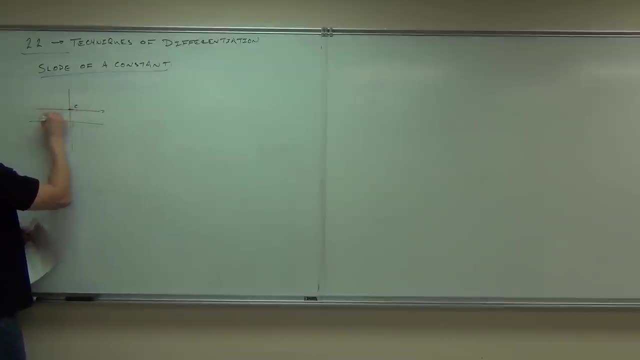 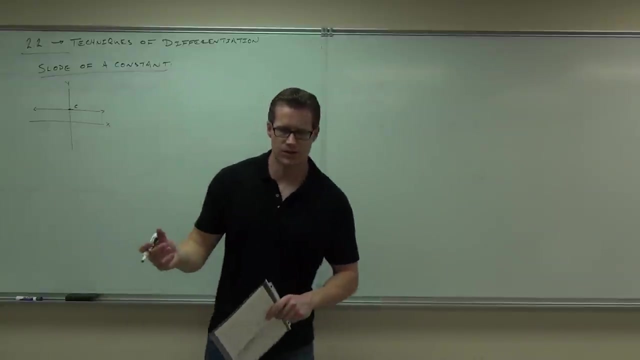 So that's a constant line. Tell me something. Supposing I had drawn this perfectly, what's the slope of my line there? Zero, Sure, because we know the slope of any horizontal line would be zero right, And the slope of a constant is, in fact, if it's not rising or falling. 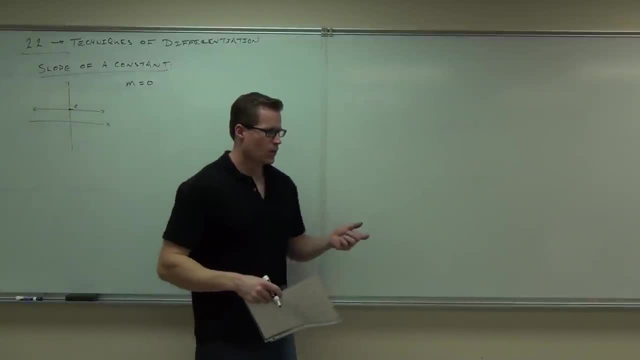 All right, cool. Well, wait a second, though. What does derivative stand for? Slope of curve? Slope of curve? In our case, our curve is a horizontal line. It's still considered a curve, even though, ironically, it doesn't curve. 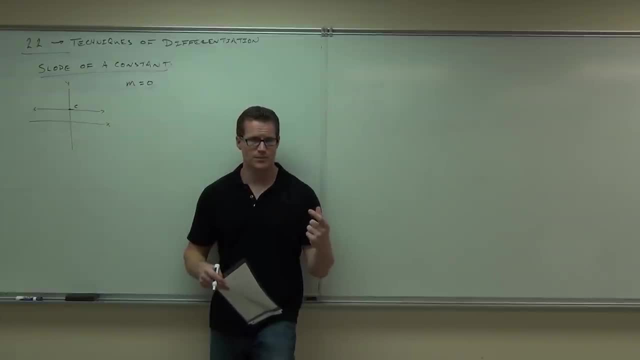 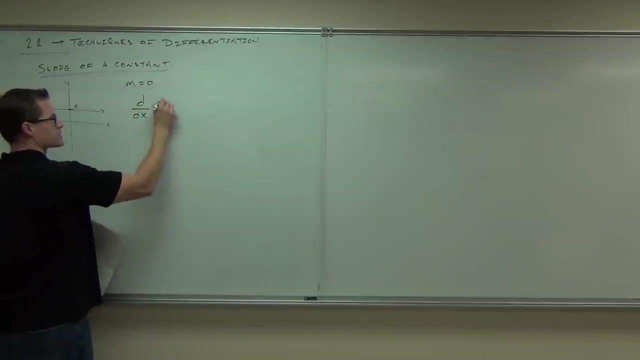 Still, though, if derivative means slope, you believe me that derivative means slope, right? If derivative means slope of a function- and the slope of our function is always zero, no matter what- then the derivative is always zero. Okay, of a constant. I've been completely general. 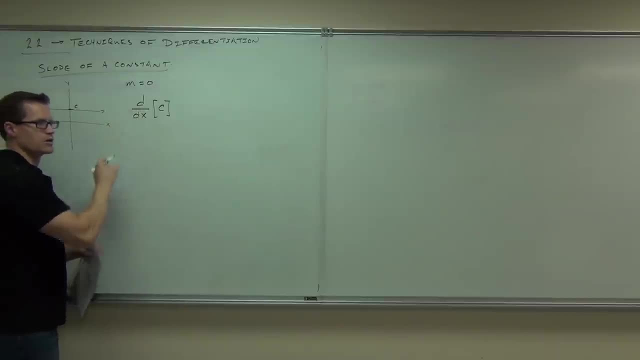 about this constant. I don't know what it is. It could be negative, positive, whatever. What's the derivative of a constant? Basically, it's asking this question: Don't forget what a derivative means. Derivative means slope. What's the slope of a constant line? 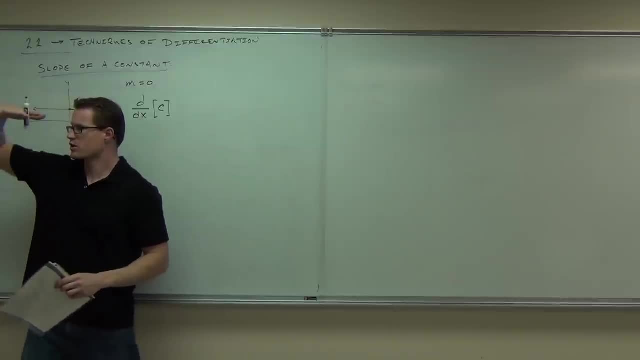 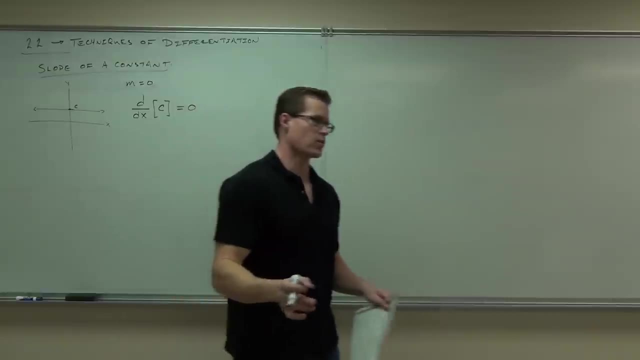 Zero, Zero, sure. What's the slope of a horizontal line? Zero? The derivative of any constant is zero, no matter what, That's kind of nice. Do you believe that? Do you buy into the reasoning why horizontal lines have no? 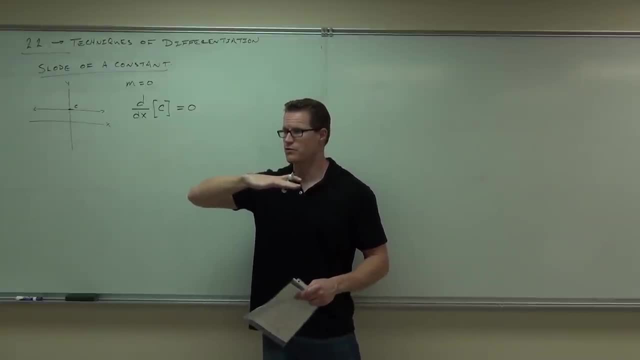 slope or they have a slope of zero. I should say They have a slope of zero. Therefore, the derivative of a horizontal line must give you zero. Derivative is slope. Slope of horizontal lines are zero Constants give you horizontal lines. so the derivative 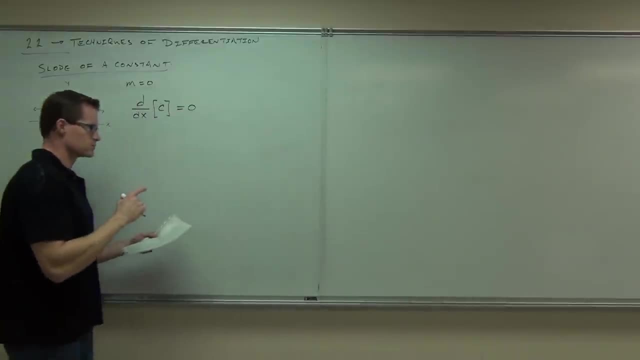 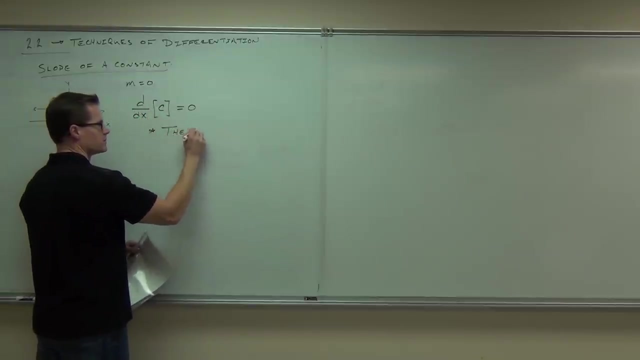 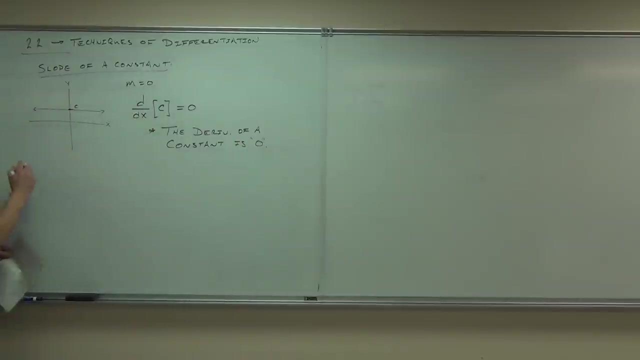 of a constant is zero. That's kind of nice. So in English this says: the derivative of a constant is zero. Okay, basic examples, just to make sure that you get it. Okay, what's the derivative of? what's the derivative of three? 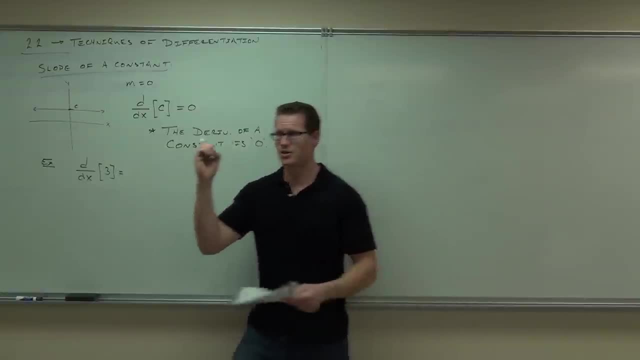 Three is a constant. What's the derivative of a constant? No work at all. That's fantastic. I love it. No more limit, right, If you have a constant, the derivative of a constant is zero. See, the derivative is just zero. 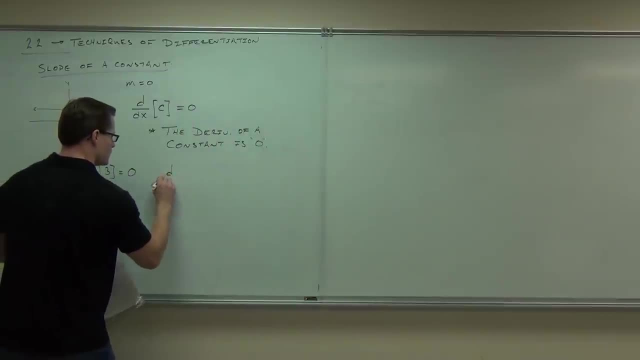 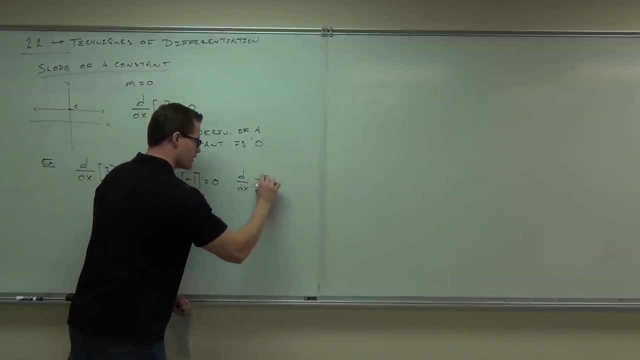 That's easier. What's the derivative of? derivative of negative one: everybody. what is that Zero? No thought at all. Derivative of a constant is zero. What's the derivative of pi? Is pi a constant? Pi is just a number. 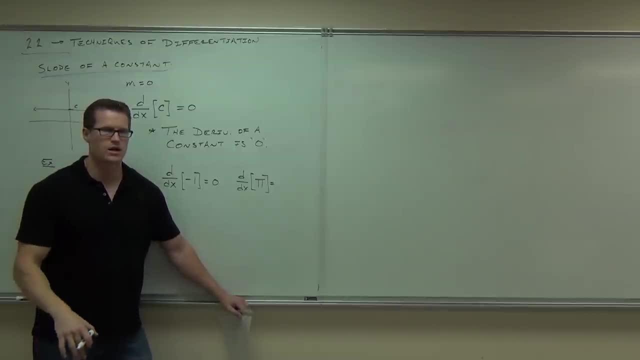 It is 3.14159 and forever, whatever that is, But it doesn't matter that it doesn't end. It's still a constant number, isn't it? It doesn't change. The derivative of any constant is zero, So this is zero. 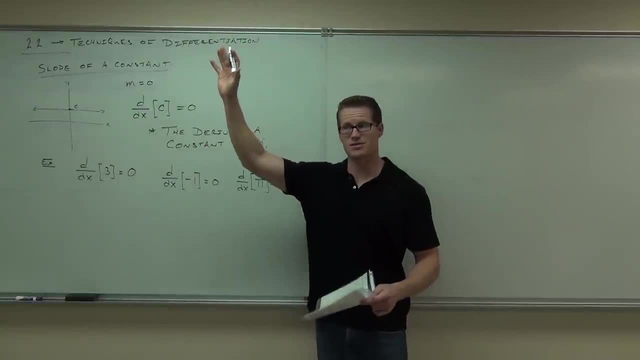 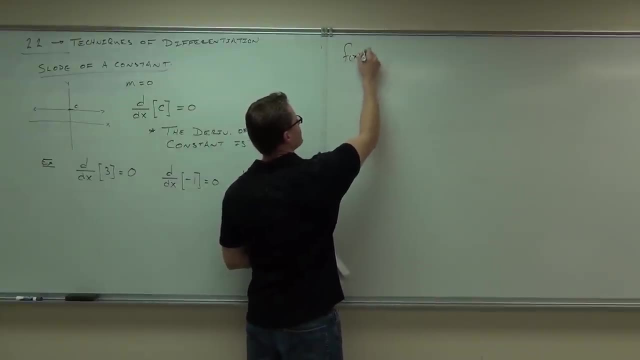 How many people feel okay with the derivative of a constant as zero? Good, That's kind of nice, right. We didn't even have to use limits over there. Unfortunately for us, when we come up with something that does have a variable in it, there was a formula. 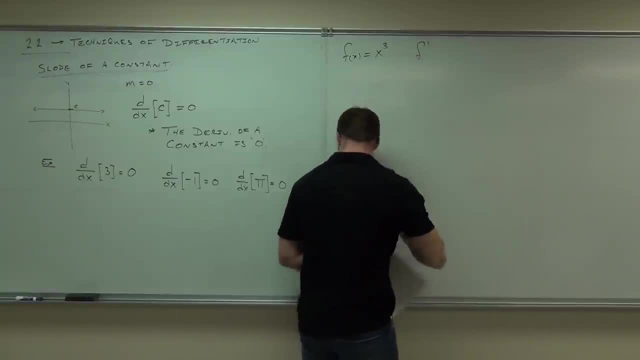 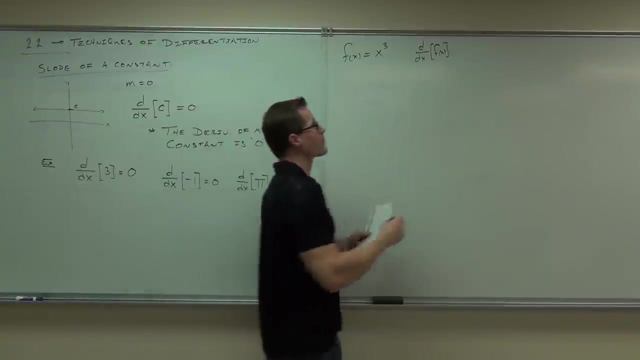 that we were able to use. We knew that the first derivative- or I'll use, just so you get familiar with it, The derivative of f with respect to x- that's what that is- was what. What did it start with? 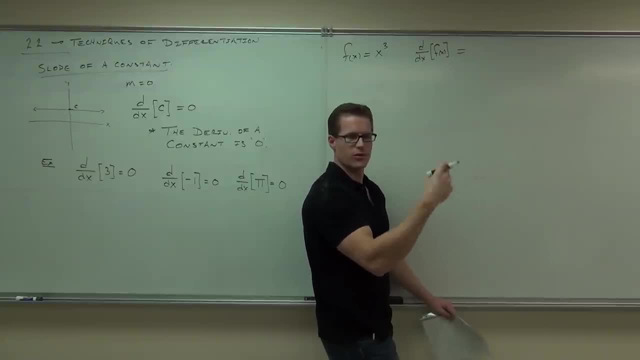 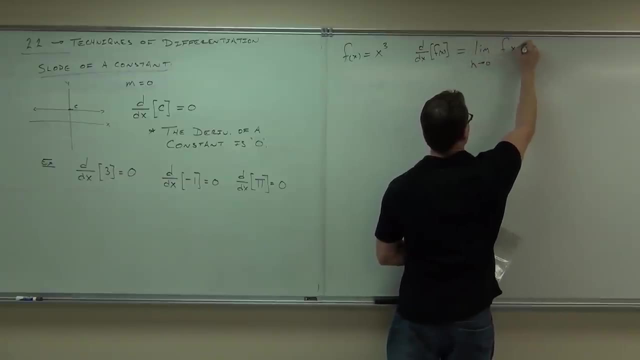 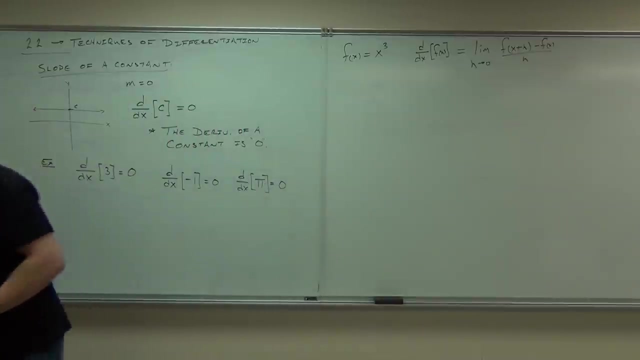 The formula to find a derivative. Oh, before that, Limit, Limit Need a limit As h crunches zero. Cool, Minus f minus h, Love it. Okay, That's how you find the derivative True. We've practiced a lot of time on this. 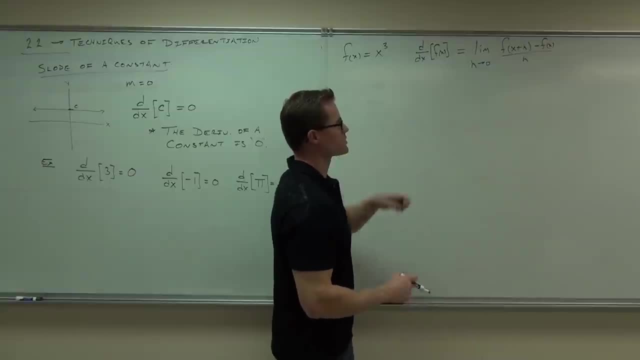 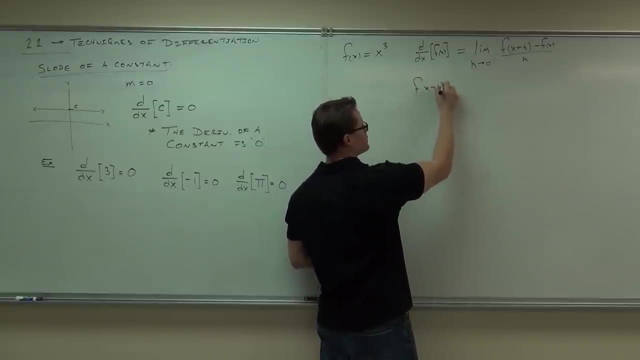 This is one of the examples we've got to do. is this one? I want you to see what happens with this. okay, So we're going to work this through right now. I've asked you to find f plus h. I'm sorry. 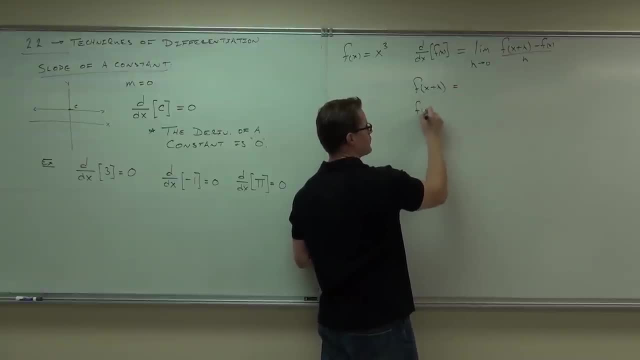 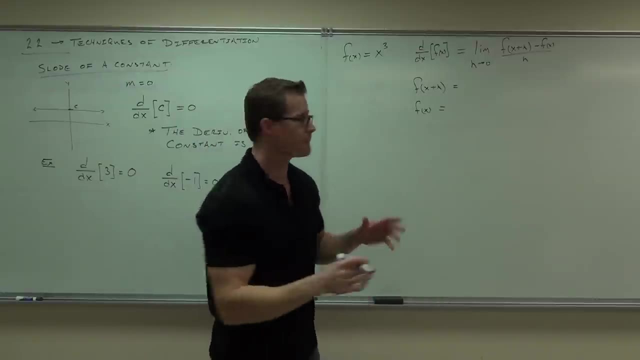 f of x plus h first, and f of x- Find them independently. Then we plug them in and we figure out what this is going to be. What is f of x plus h? What's that going to give us? in this case? f of h cubed. 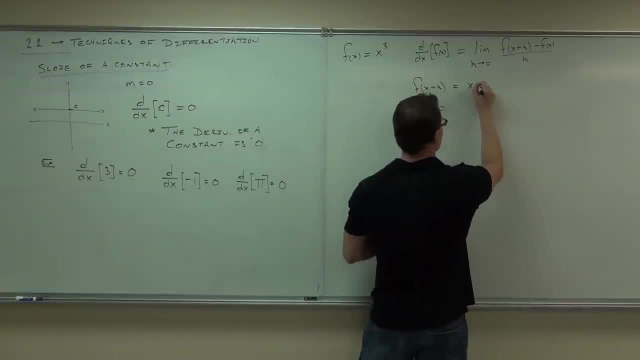 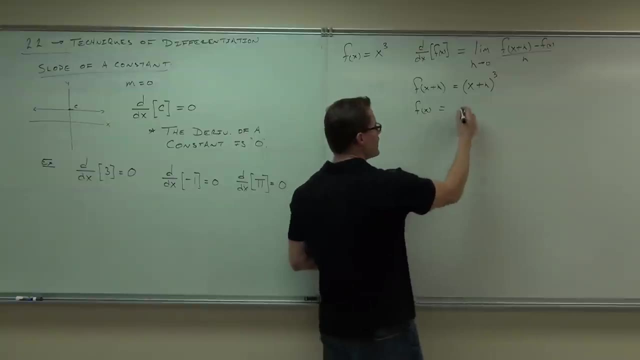 Very good, It's just a composition. We're just substituting that in. Have you gotten pretty good at that so far? Yeah, Just don't separate the x plus h, You'll be fine. f of x is just x cubed. 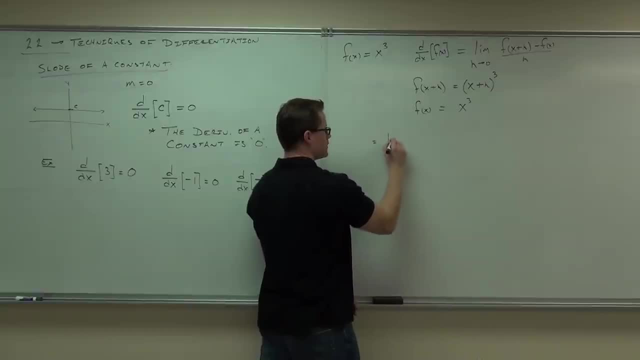 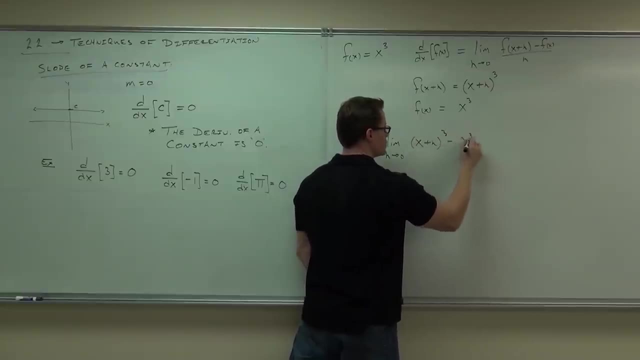 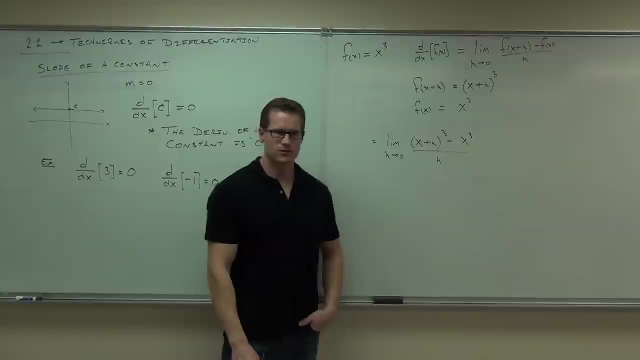 So we know our first derivative is going to be limit: h goes to zero. x plus h. cubed minus x. cubed all over h. Still all right so far. What do we do now? Yeah, we've gone through this a lot. 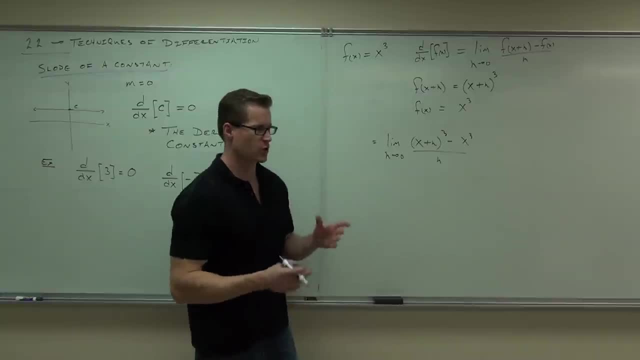 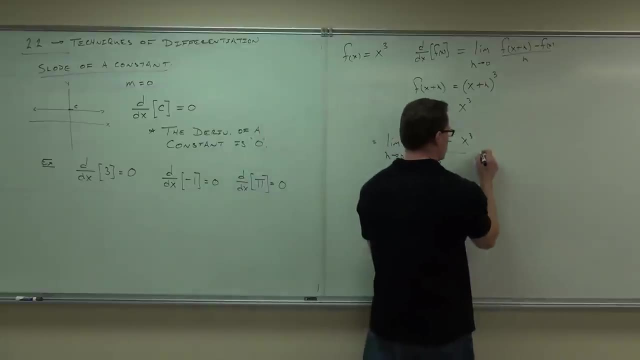 Now it's basically just algebra: You distribute, you combine some like terms. Hopefully you're able to factor an h out, and your whole goal here is to cross h's out. True, That's your whole goal. So in our case we'd go all right. well, this is limit. h goes to zero. 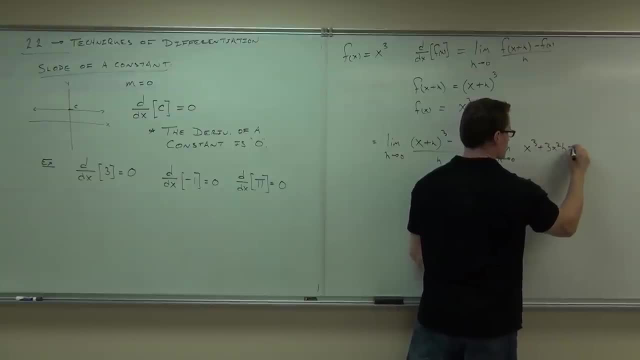 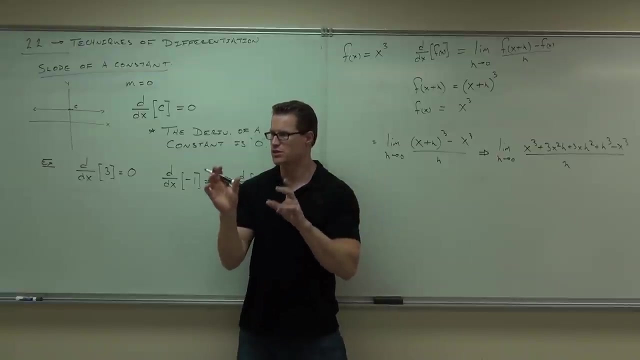 We've got x cubed plus 3x squared h plus 3xh squared minus. I'm sorry, plus h cubed. I did that kind of fast but you would just distribute that all out: X plus h. times x plus h. times x plus h. 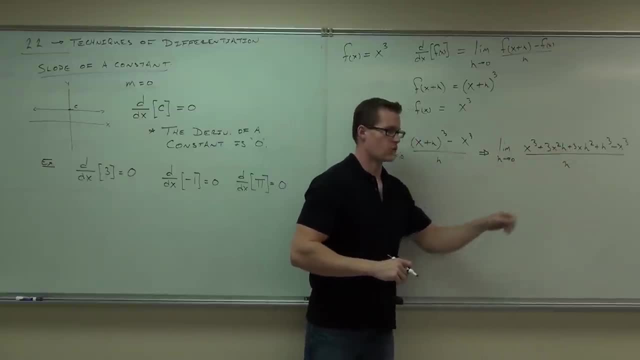 Distribute, combine like terms and I guarantee that's what you're going to get right there. If you want a quicker way to do that, you come see me. I'll show you Pascal's triangle and how to do binomial expansion. 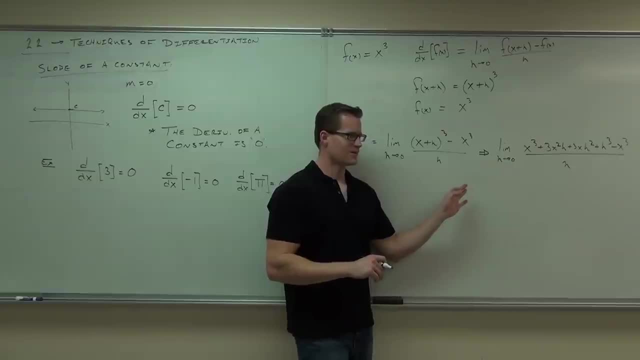 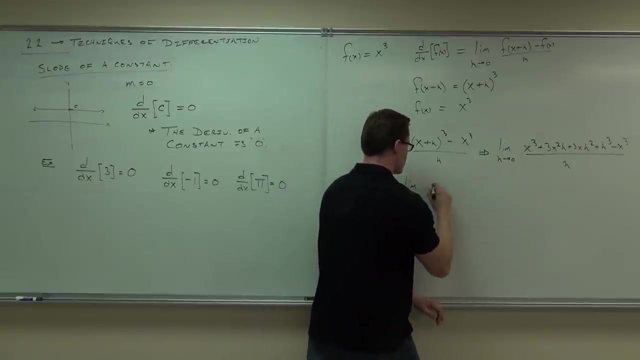 It's not hard. So far, so good. Does everything except for the h terms cross out? In that case, that's just this one and this one. So we get limit h goes to zero. 3x squared h plus 3x h squared plus h. cubed over h. 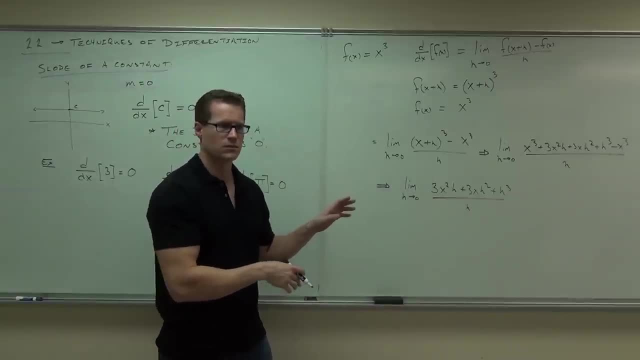 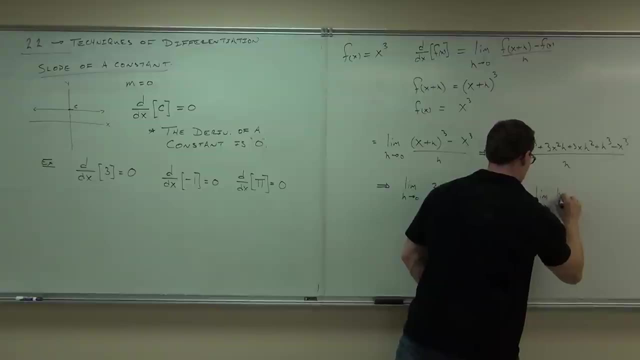 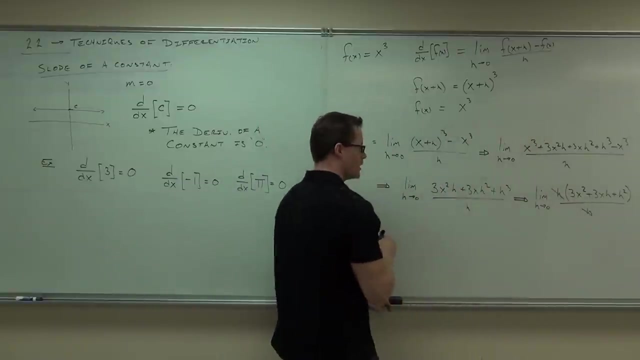 What would I do now to finish off this problem? Back around and cancel the h's out? Perfect, You're still with me, right? If you've done work like this before just some algebra cross the h's out. let the h go to zero. 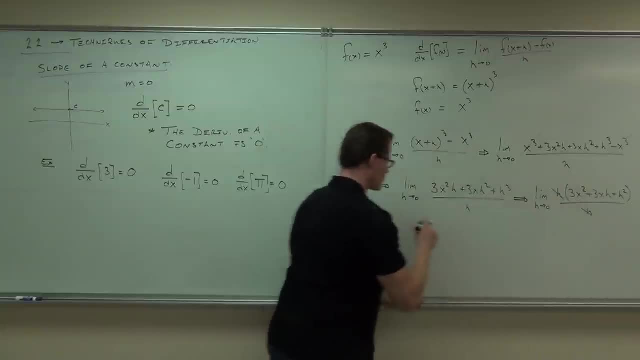 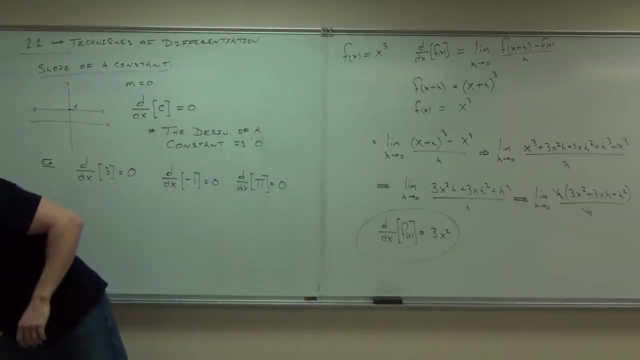 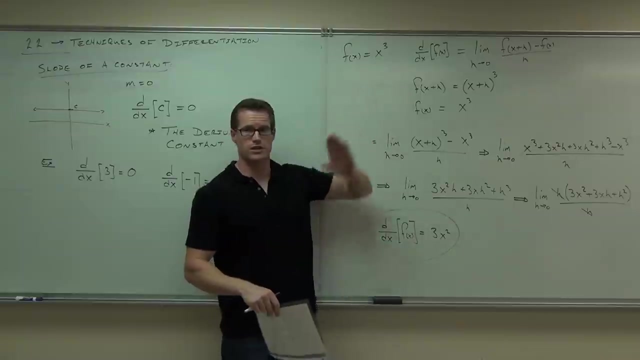 because now you've gotten rid of that denominator. and what are you going to get out of this whole beautiful thing? Three out of x squared. Three x squared right. Beautiful, What did I just find? The formula of the slope, Yeah, so this gives the slope of this function, this s curve at any point, right? 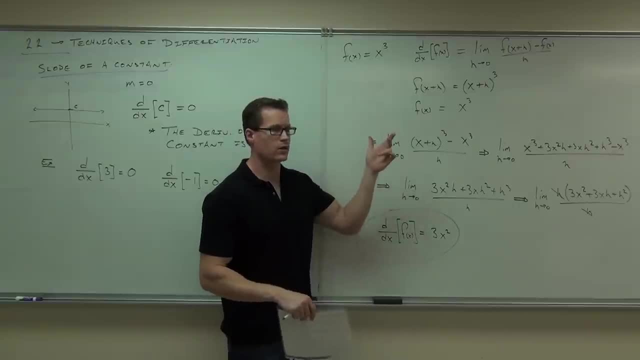 If I had to give you a point like 1, 1, or I give you a point like 2, 8, you could plug in the 2 or the x value. you could evaluate it. find me the actual slope and find me the equation. 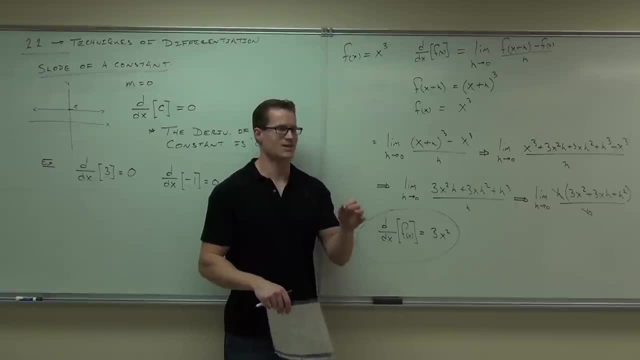 of the tangent line of that specific point, Could you not? I hope you're like: yes, I can do that right now. That's where you should be at this point. Here's the thing. This is going to be from someone who hasn't taken calculus before. 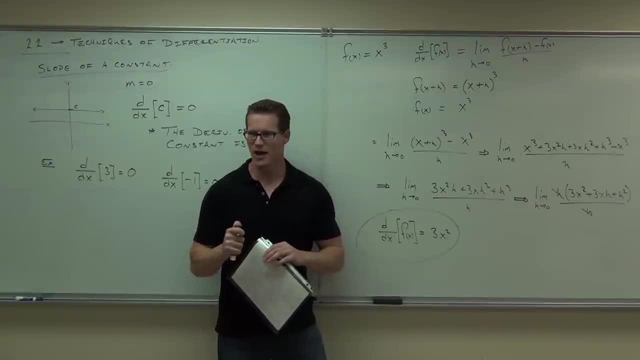 I want an answer, Do you see, because I know some of you have. so, those of you who don't love me that much, but those of you who have not had calculus before, you're going to love me, You're going to love me. 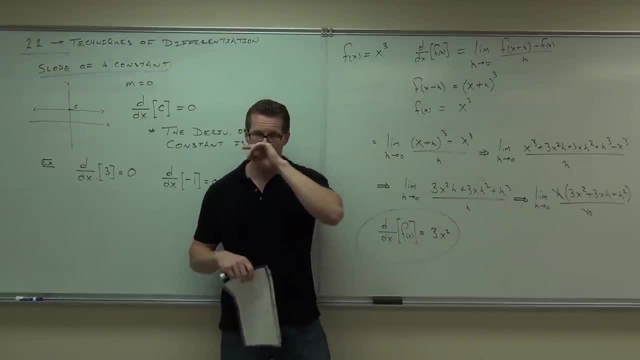 Does this suck? Yes, This sucks. I want you to think: Is there a way that you can go from here to here without garbage? Do you see a pattern? Do you see the pattern on Someone who hasn't had to take calculus before? 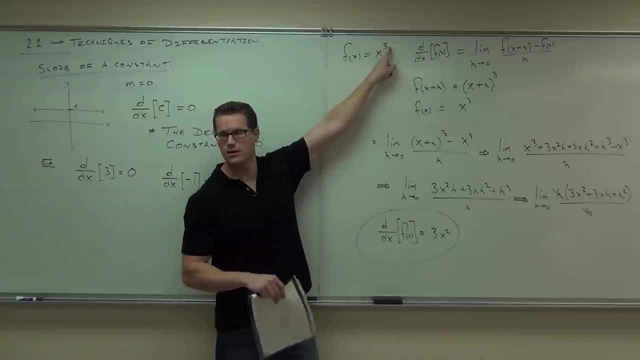 Where does this number go? What happens to this number? So, from this to this, all that happened was this number went out into the front right And one got taken away from that number. Do you believe me? Guess what Works all the time? 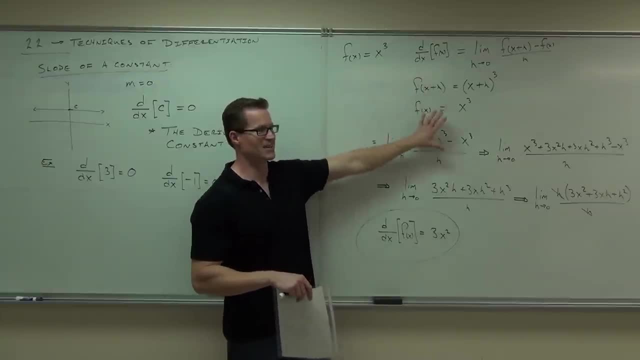 All the time. Do you ever have to do this again? Why do you think I teach you this one before I teach you this one? Because if you want to ever do this, yeah, you don't have to. This is the formula for a derivative. 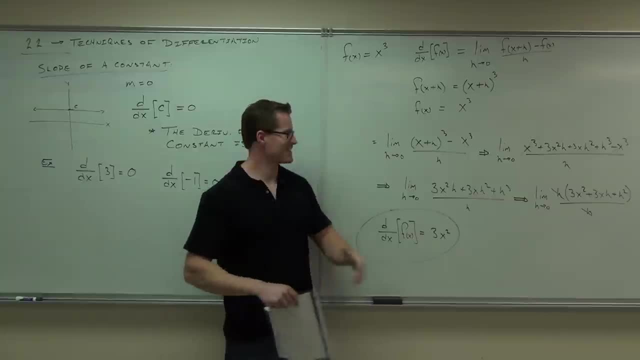 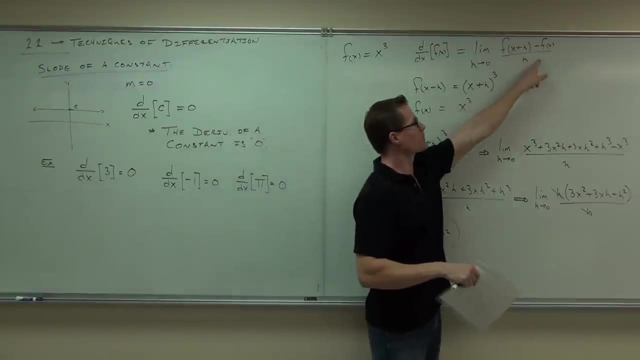 What we're going to learn now are shortcuts. This is horrible. Why is there even a formula when you can just do that? Because this is what we're doing. This is the slope, and this is the only way that you can let the points. 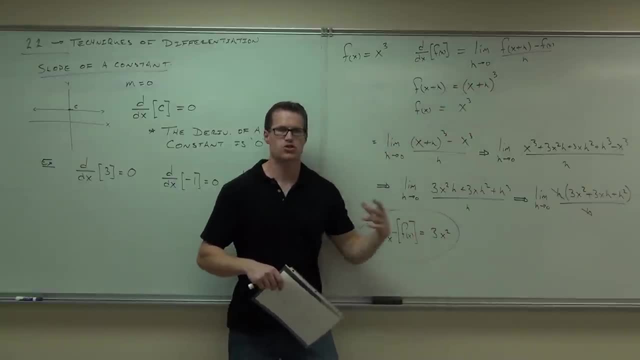 the distance between them go to zero. This is it. This right here is a shortcut that works every time. So what's the actual calculus? This is the actual formula. This is the actual calculus. That's it right. This is the stuff that works. 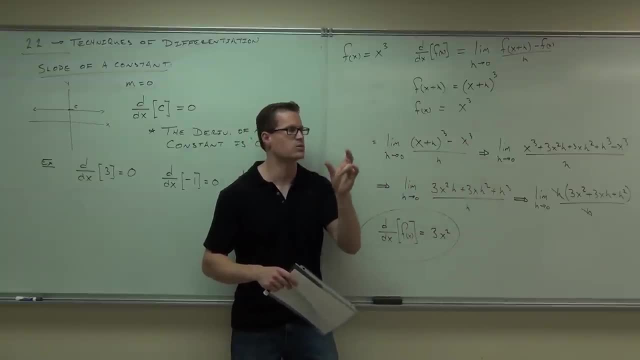 The limit is the fundamental of the calculus. That's how you let it happen. Now, techniques of differentiation says great. we understand that. What's the way we can put this in practice and actually do the derivatives all the time? This stuff right. 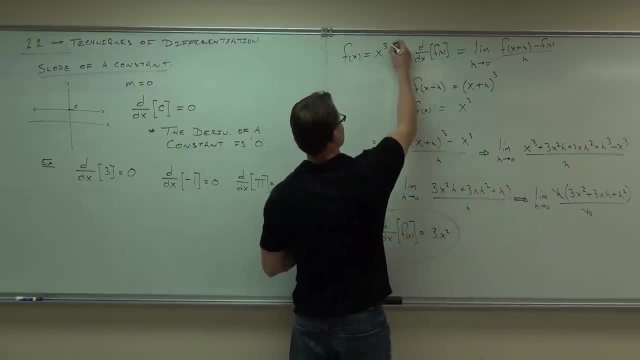 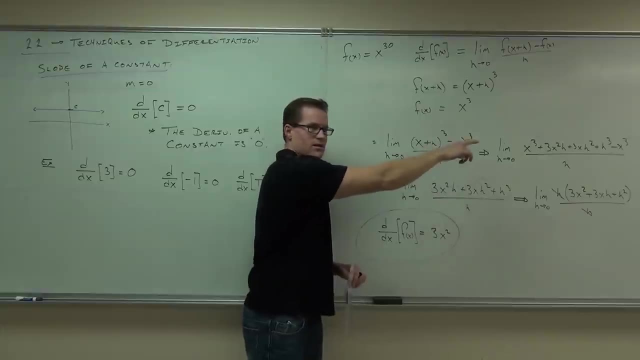 Because here's the thing You're going to want to do- that That has to be a 30.. You want to do that? No, I don't either, But the thing that's going to happen is: it's a polynomial right. 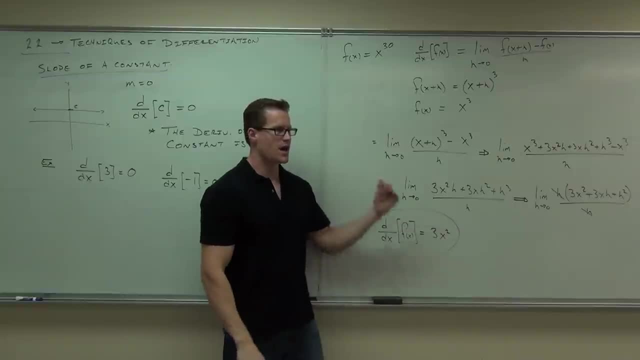 It's a very basic polynomial. What's going to happen is, if you do binomial expansion, every single term in here- think about this, you can think about it- Every term in here is going to have an H, except for the very first one. 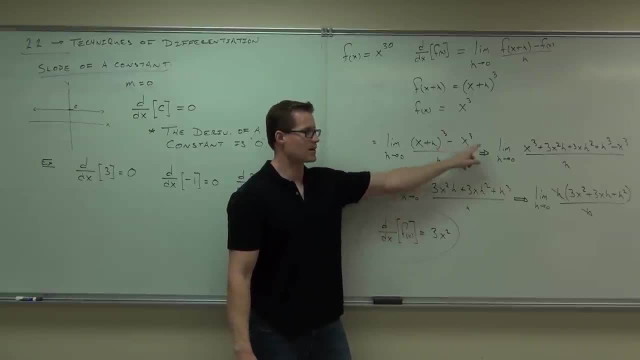 True, The very first one is not, And you're subtracting exactly that function from it. So that's going to be gone. Everything else has an H. The very next term will have only a single H, That's binomial expansion. 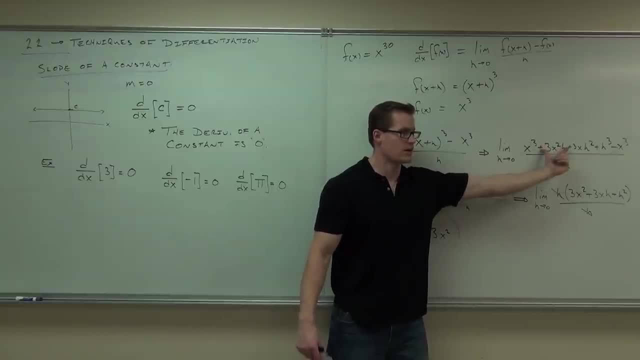 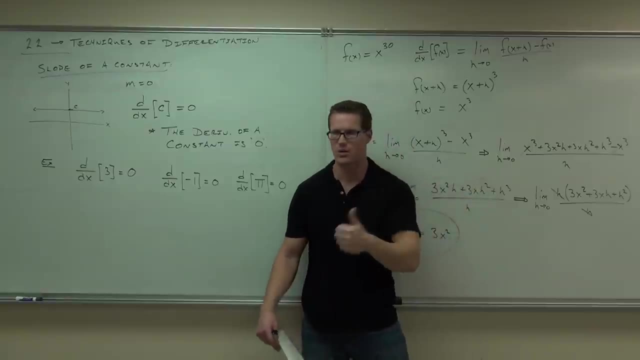 When you factor that H out, you're only left with this thing: Binomial expansion says how you get this is that goes there and that becomes one less. That's why this works. That is the power rule for derivatives. So what's calculus? 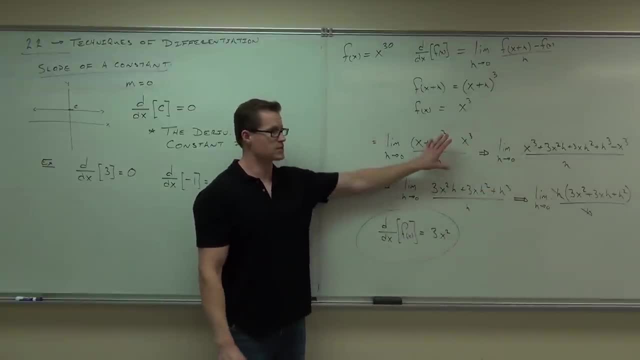 This is calculus. What's the easy way to do it? That's the easy way to do it. You have to know this, because that's what this class is all about. all right, You're finding slopes, and that's how you do it. 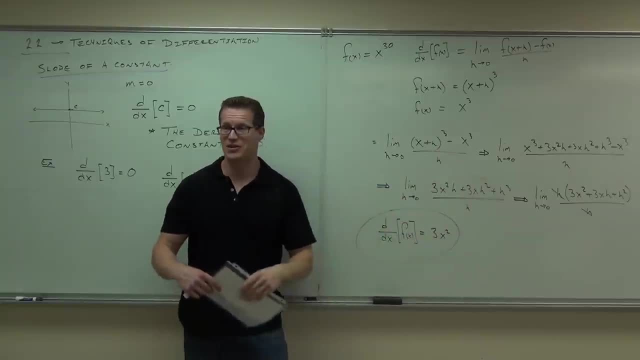 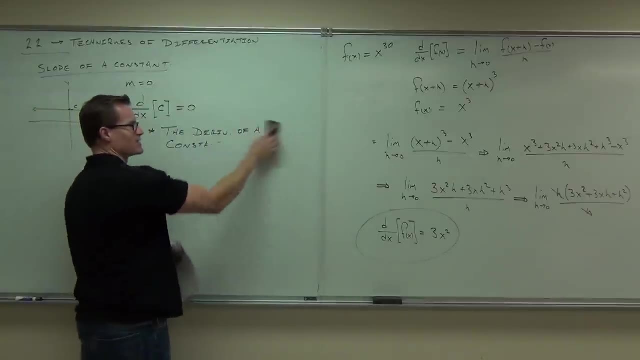 In practical application, though, you just kind of cheat a little bit. You ready to learn how to cheat? Yes, That's what I love about this stuff. I love cheating. It's not cheating. Everyone does this. If everyone does it, it makes it okay. 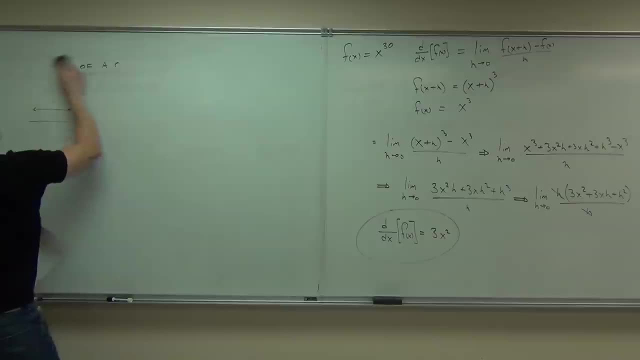 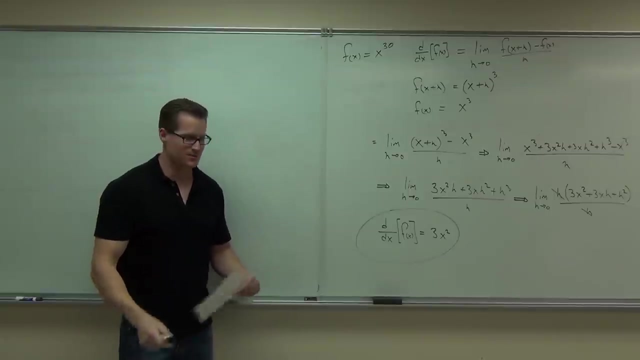 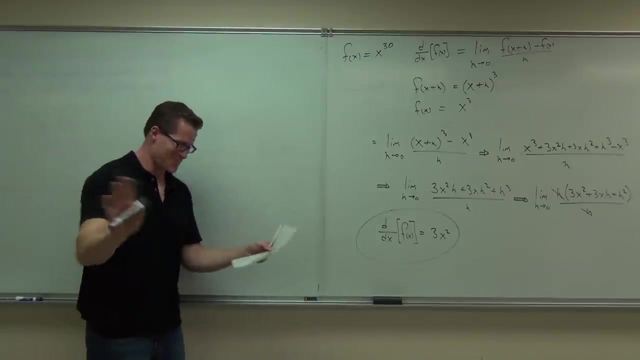 That's not true Really. So if everybody jumps off a bridge, Please do it. We have a shortage of food. I mean just kidding You two on YouTube or wherever. don't jump off bridges. That's ridiculous. It doesn't hurt sometimes. 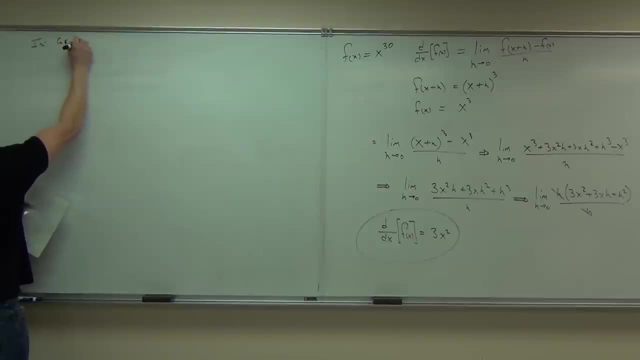 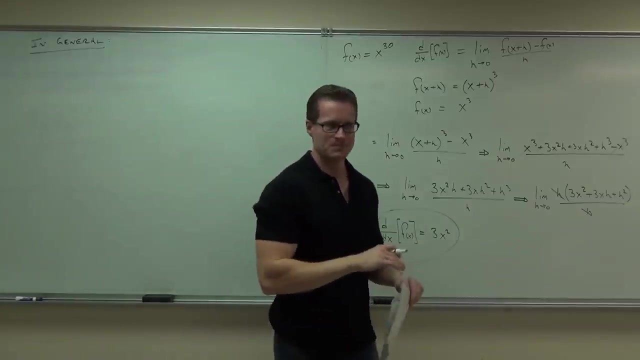 It does You just hope that sarcasm invokes you. Okay, if n is any integer, this works. We're going to find out later. if there's no qualifications on n, It can be anything, But for right now any integer works for us. 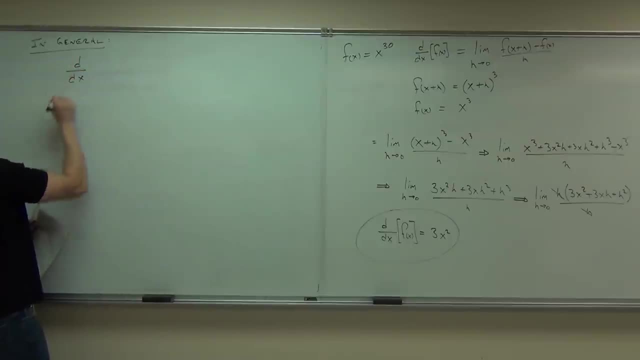 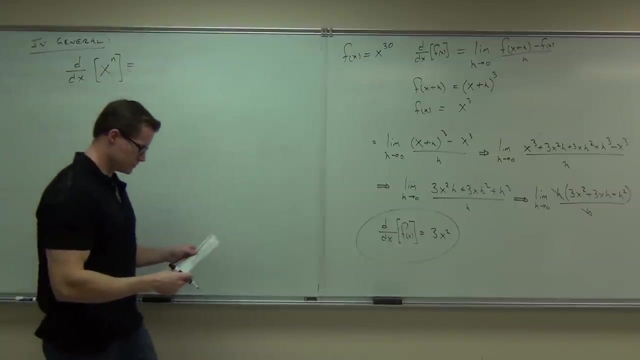 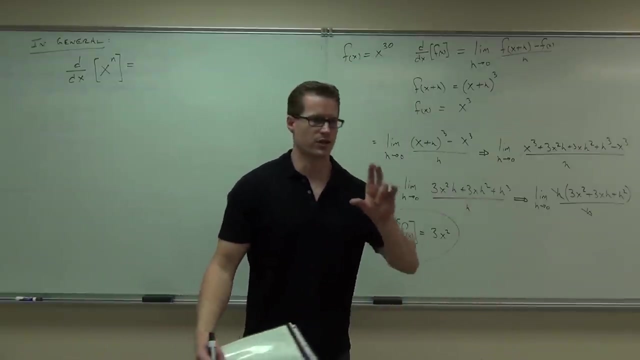 This is a true statement. The derivative of any x to any power is equal to. Notice: ddx stands for derivative. That's true, The derivative. that's how I'm going to be writing most of the derivatives in here, because it's very nice, notationally, to write it this way. 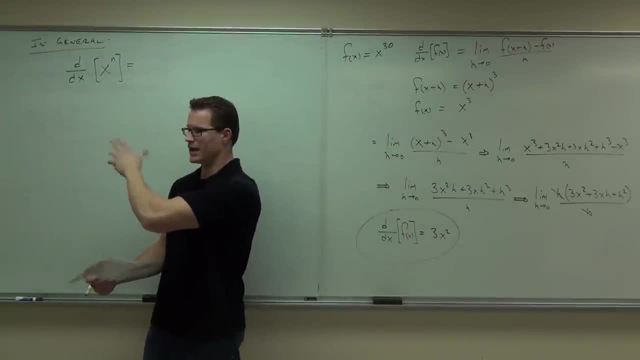 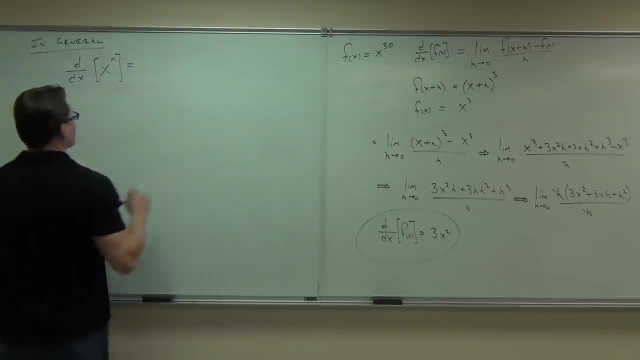 It's hard to write it with the f prime to do this. I don't like that. I like this way to say: I'm taking the derivative of whatever's in there. Do you understand? It says: take the derivative of this. What you get out of that is what happens to the. well, it wasn't a 30 anymore. 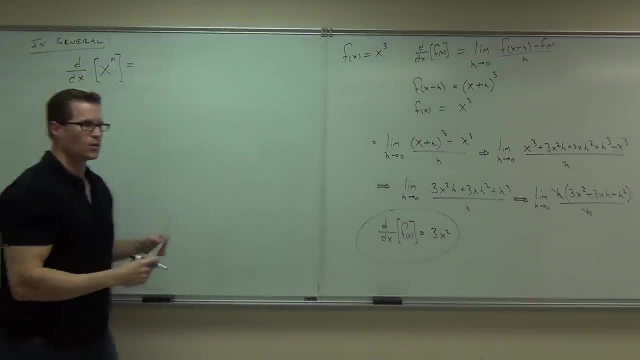 It was a 3.. What happens to the 3?? It's a symbol that represents the 3 here. What's the n going to do? You just pull it. You just pull that n out front. The x doesn't change. 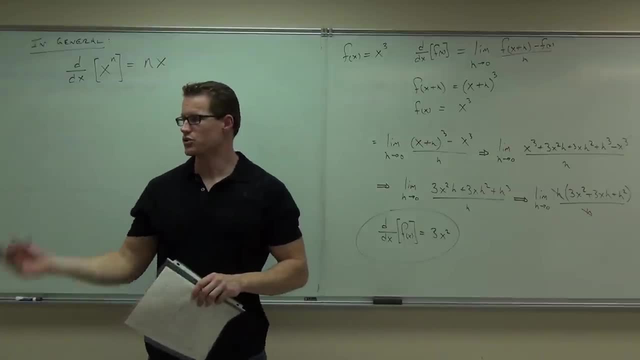 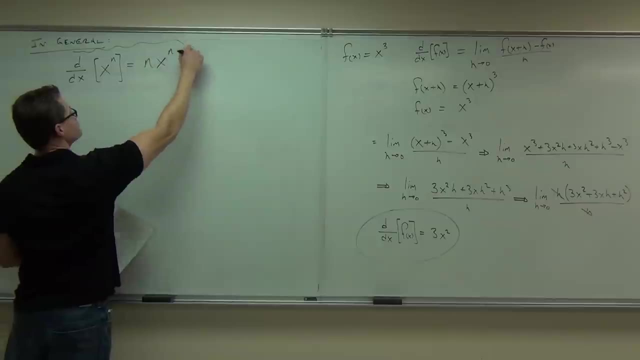 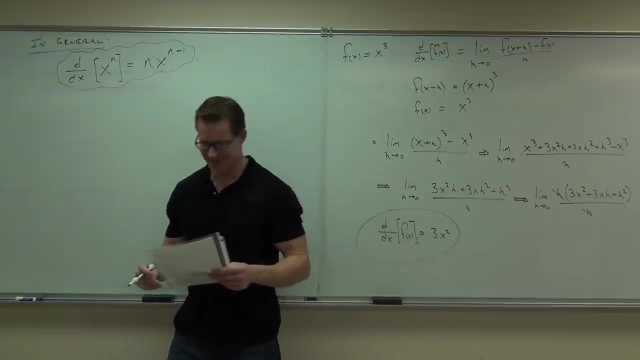 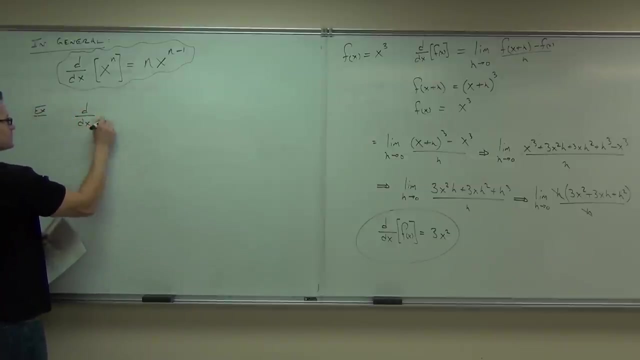 But what happens to the variable Sure? you subtract 1 from it, That's n minus 1.. Do you love me? Told you you'd love me, Maybe not. Not yet You're going to. So can you do? we've actually done that derivative before, if you remember. 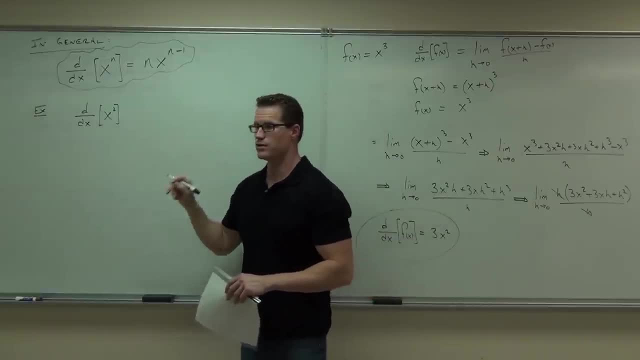 We've done it twice, We've done it the long way, both with limits. Can you do that derivative? What's the derivative of x squared? That's what this question asks. Derivative of x squared: what do you do? What happens to the 2? again? 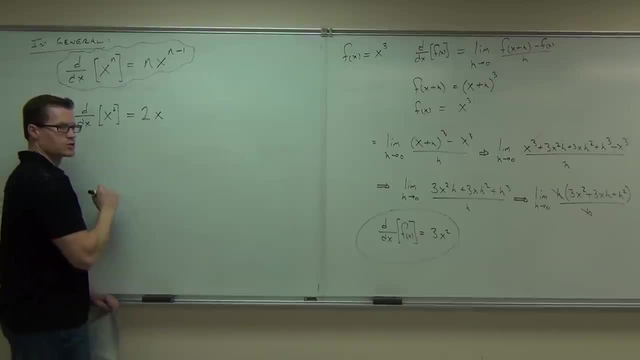 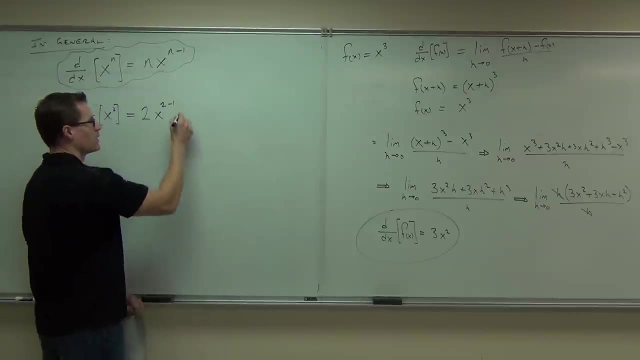 It fits this format. So 2 goes here, x to the how much, Because you're going to do 2 minus 1.. Now, I'm rarely going to show you that math. We're just going to assume you can subtract 1 on your own and get 2x to the first power. 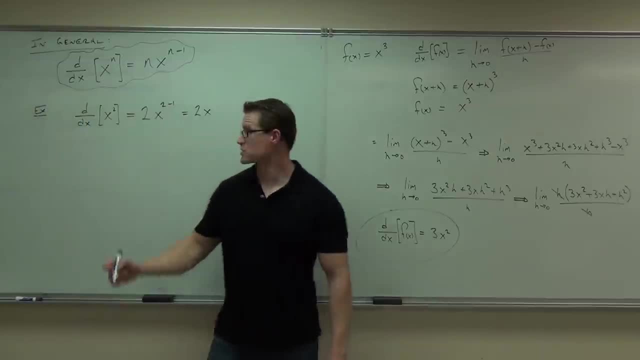 We're just going to do that: 2 minus 2x. Hey, that's kind of cool, because you've just found the slope of that curve in less than 2 seconds without doing any limits or anything like that, right? So I could ask you this question and now the same exact question I gave you on your test. 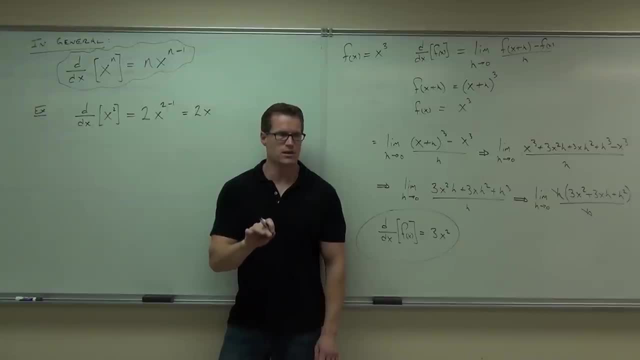 and you could do it in like a minute, maybe less, Because I say: find me the equation of the tangent line through this curve at the point 2 comma 4.. Can you do it? Yeah, at 2 comma 4, here's your slope, right. 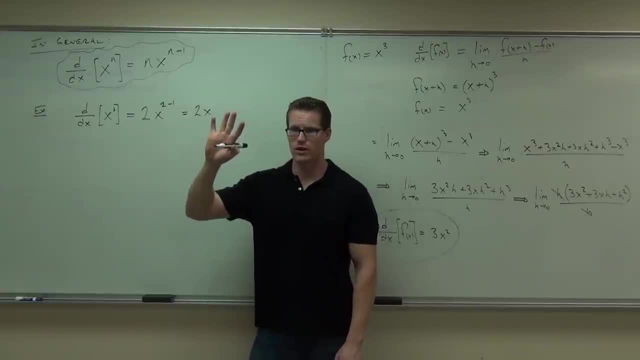 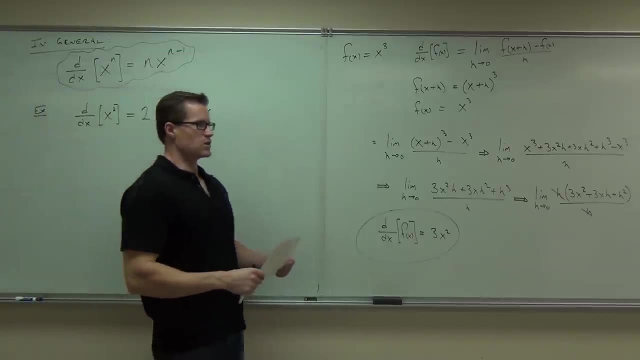 Plug in 2, you get a slope of 4.. Now you have a point and you have a slope. It's very quick. So, on the test, are you ever going to tell us to do that? Yeah, probably once, to make sure you can do it. 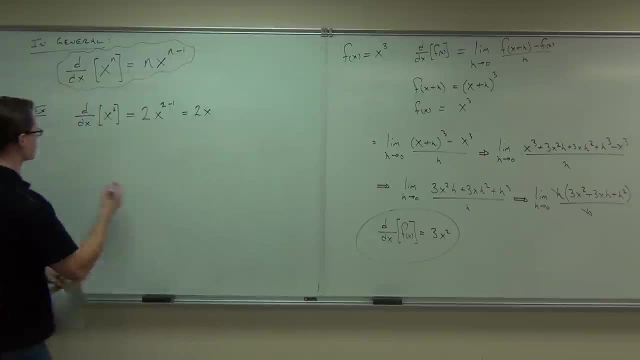 Yeah, but after that, no, it takes way too long, especially for things like this. I mean, honestly, that's just ridiculous, Even though it's very simple. that's ridiculous when it comes to this stuff. You don't want to expand that. 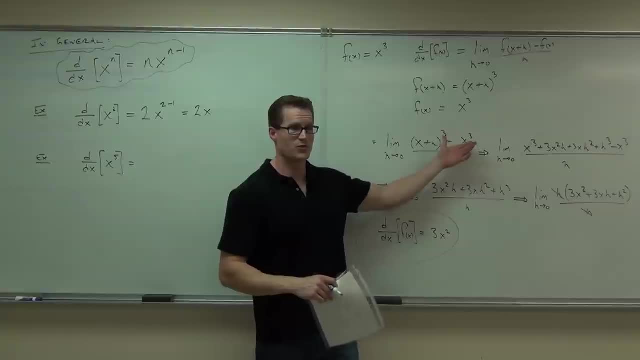 You don't want to do that. I'm guessing a whole lot of you are probably not going to come to me for it. You don't want to find out about expansion anymore, since you don't have to do those for crazy big numbers. 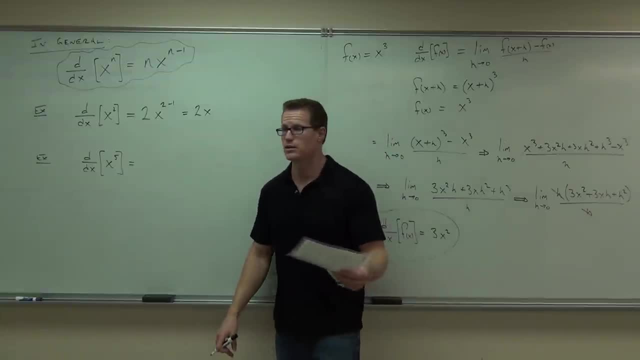 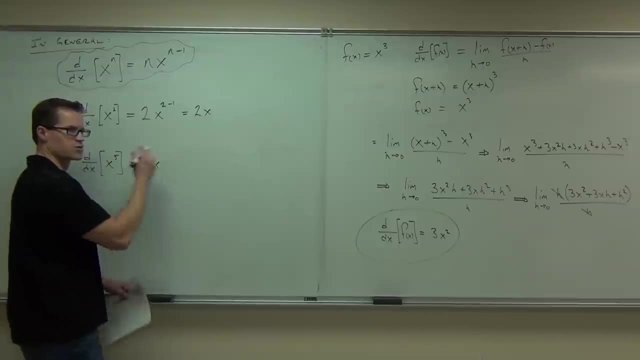 Can you take the derivative of x to the 5th? How much is it To the 1.. Good, We bring down the 5. X to the subtract 1 from that exponent you get to the 4th power. 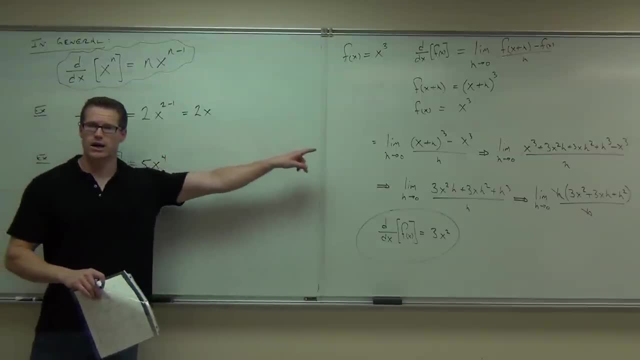 That's the derivative: Very nice, very quick. If you did it this way, would it work out? Yes, absolutely. It's just going to take you a whole long time. 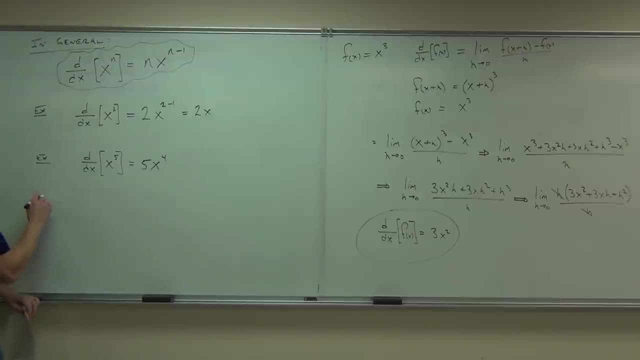 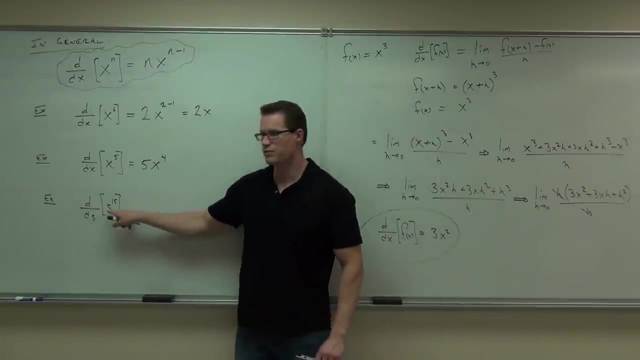 Here's one you definitely don't want to do. Dds of s to the 15th. Notice one thing on the notation. Do you notice how this has to change with the variable that I have? 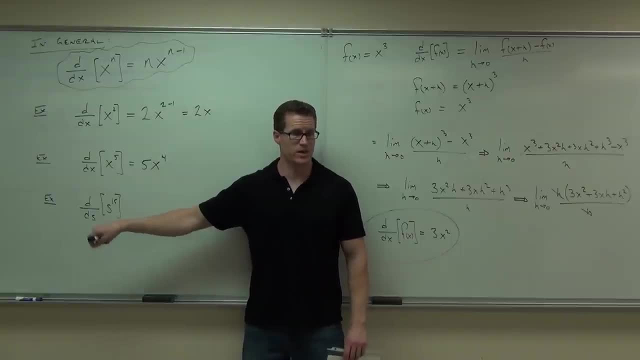 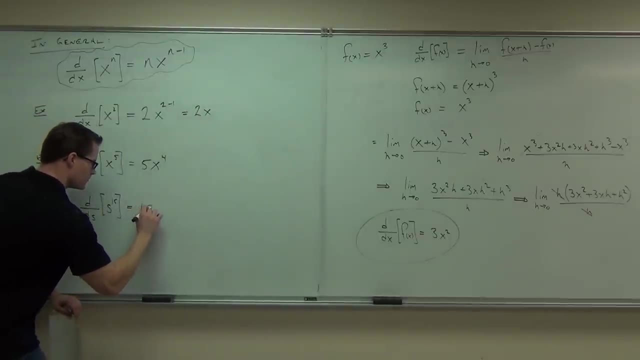 So it's not ddx anymore, it's dds derivative with respect to s, and then I'll give you the variable. so s to the 15th, What's this one? Sure, very quick, very, very fast. 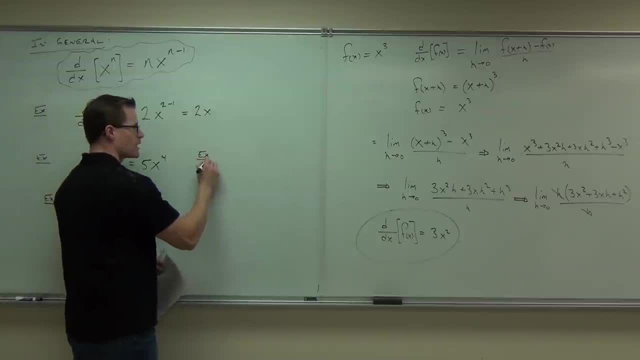 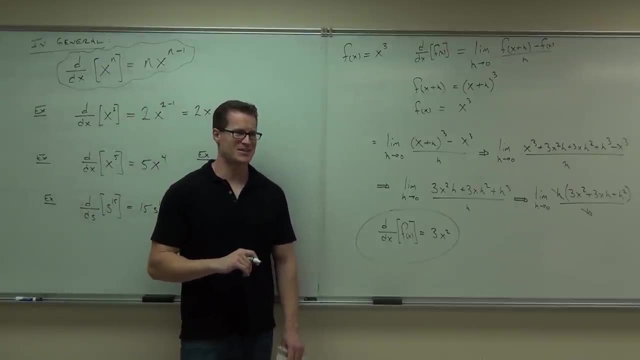 Now there are a couple of things that we should be able to do as well. What would happen if I gave you? did the shiny just wear off the calculus? Did it make it less cool, somehow that it's easier, Or did it make it like awesome, this is so not bad. 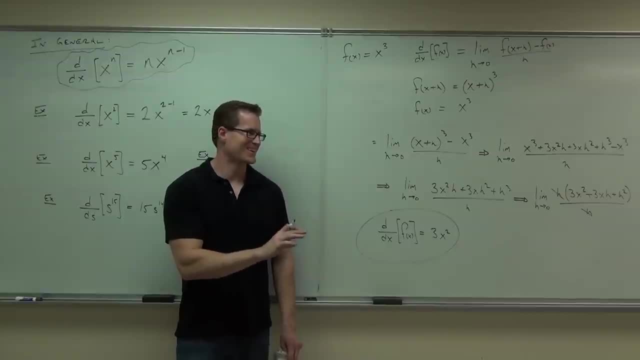 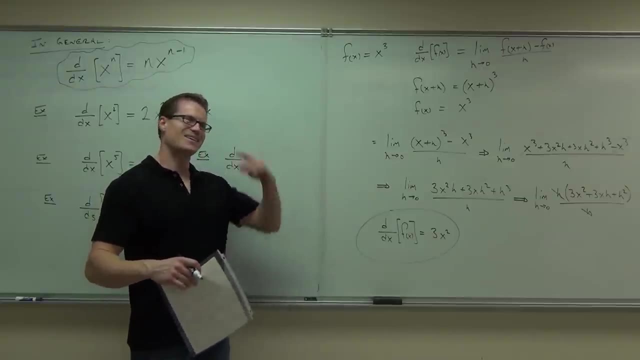 It's going to get worse. I mean, it's going to get worse. This is the common form of the storm. Yeah, this is like the eye of the hurricane. all right, You made it through the outskirts and then you're like, ah, it's sunny, I like this. 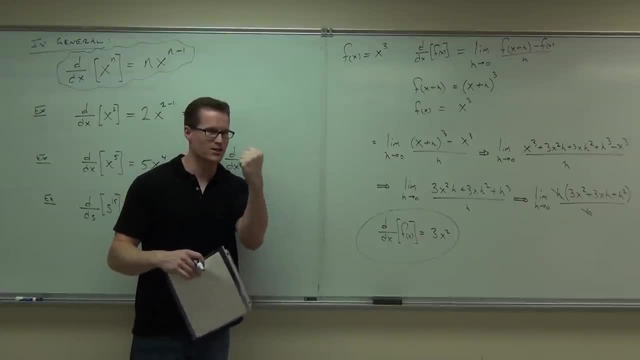 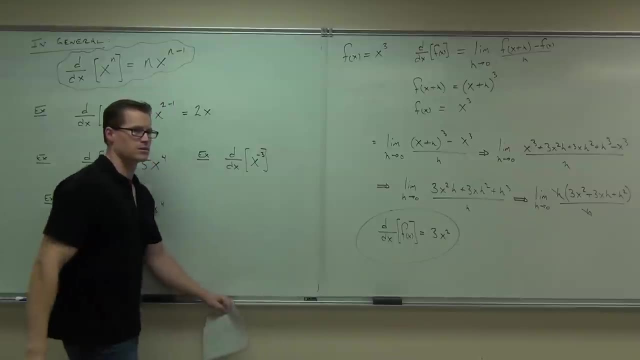 A little mist maybe to cool you off, and then I'll pound you again, But for right now, take a breath. Can you do it with negatives? Yeah, Of course. yes, absolutely you can. What do you do with the negative? 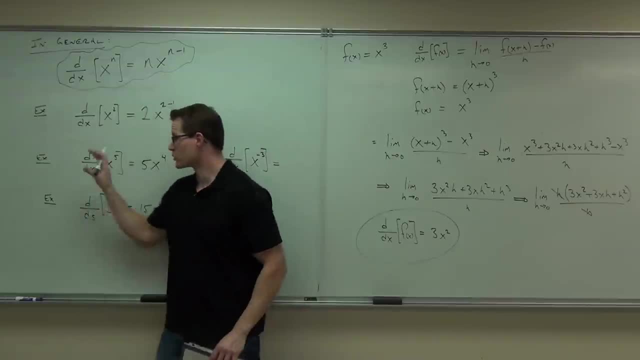 What's it going to become? What's the derivative of x to the? by the way, this is showing you work. all right, You don't have to show me any more work than this. What's the derivative of x to the negative? third, 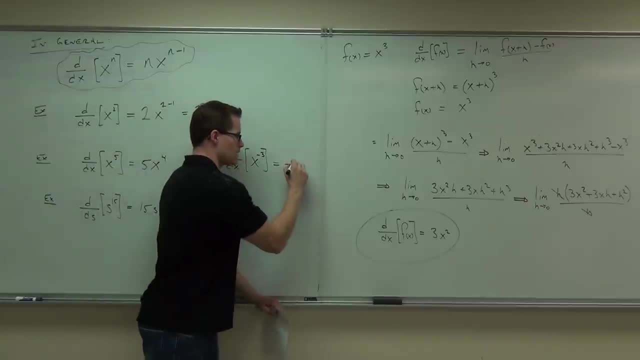 What happens to the negative three? So you still have to do that. negative three, X to the Negative four. Wait, wait, not. negative two, Negative two. Negative three minus one. yeah, that's negative four. So this is negative three, x to the negative four. 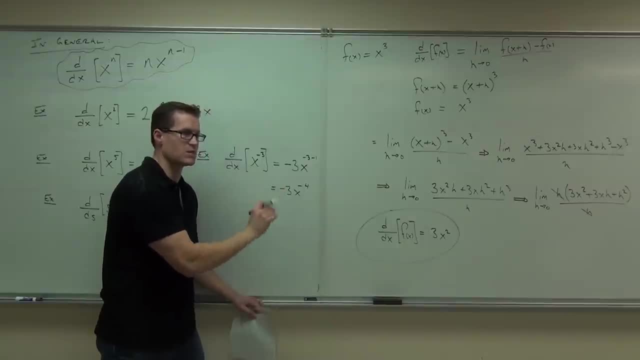 You'd be surprised how many people mess that up. all right, Watch your signs very carefully. If you're subtracting, make sure you actually are subtracting. We'll do a couple more. How about this? Do you want us to write it like that, or do you want us to export it to the denominator? 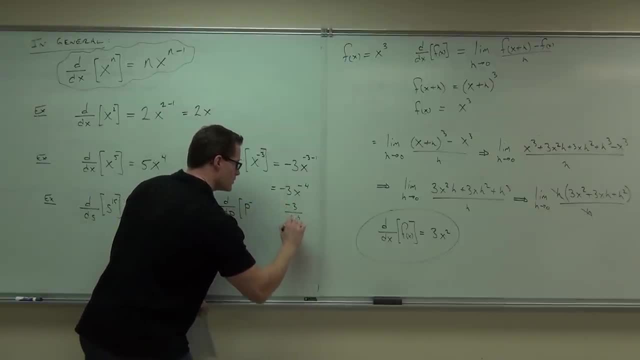 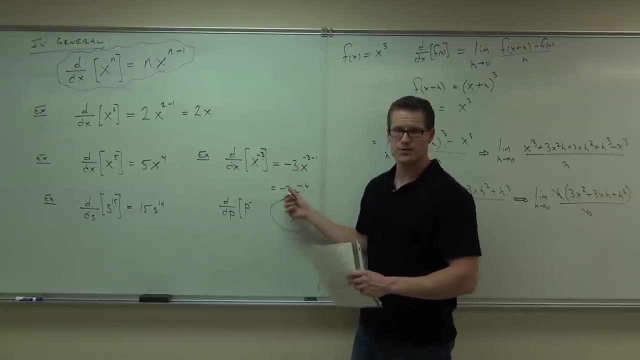 Oh, you can do this as well. Generally, I'll tell you: if I've given it to you this way, leave it this way, That's fine. If I've given it to you as the other way, give it to me the other way, okay. 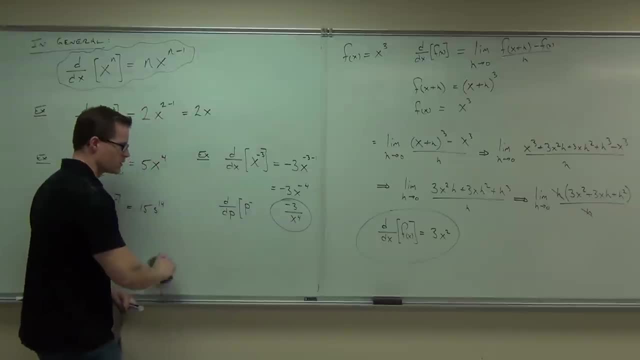 That's the general rule. If you want to write it like this all the time, that's fine as well. How about that one? What's that going to be? Negative two comes down. Negative two comes down. great P to the what. 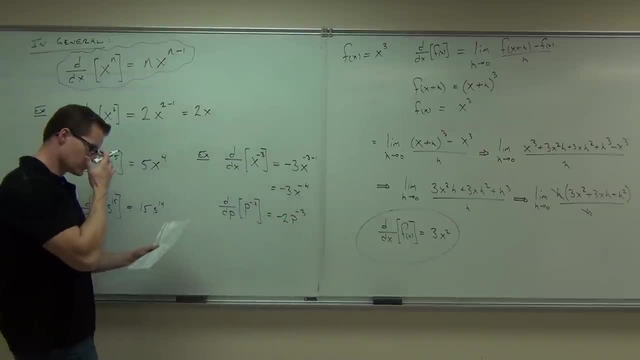 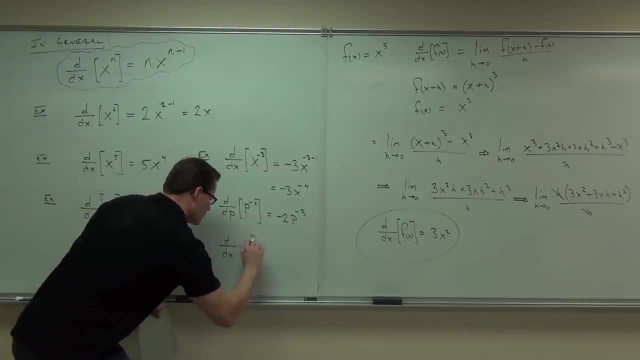 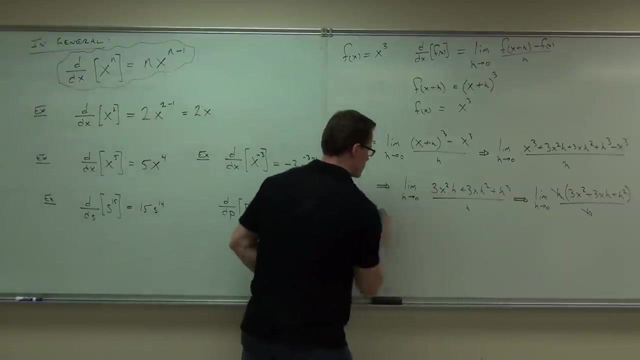 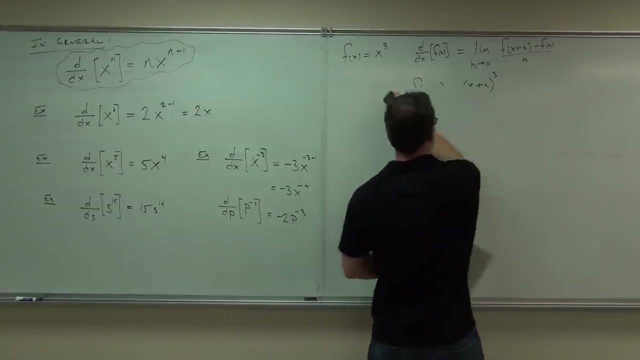 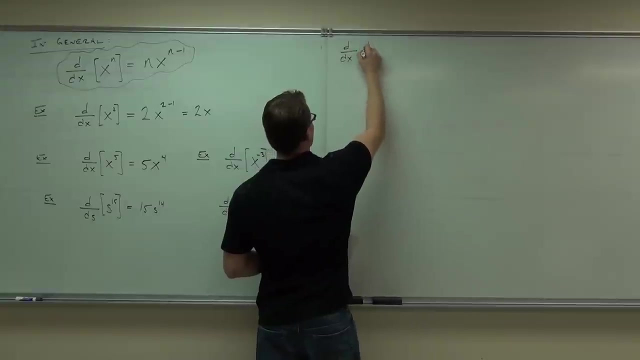 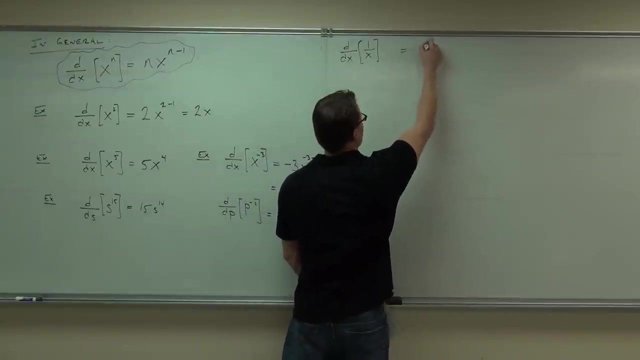 P to the three. okay, You know what. I'm going to move this one over there so you can see it better. This is kind of an important one actually, Thank you. What about ddx? one over x? Is it one over x? sorry, one over. what do you do with that? 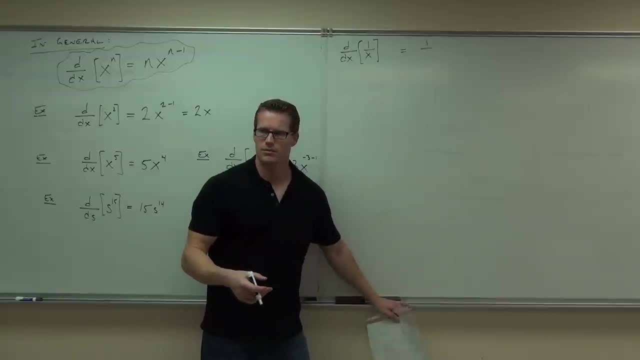 Is it one over one? You just take the derivative of x. can you do that? Move the x-prime in front of x, which is one up to the top. Aha, Make it a negative x-prime. So we have to move this so that it fits that format. 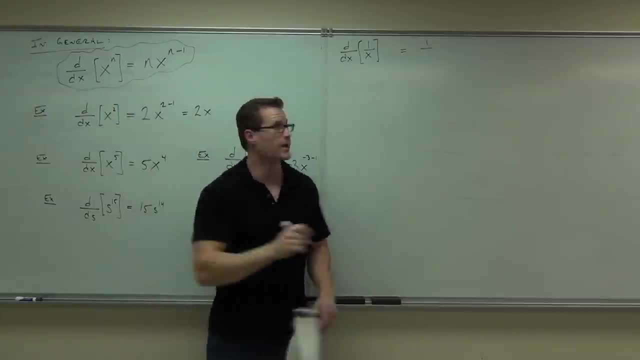 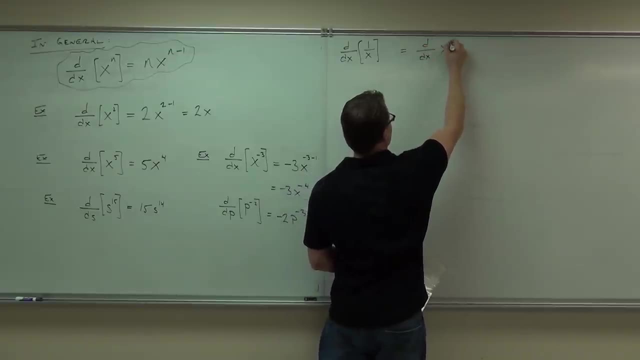 Are you with me? Right now it doesn't, So somehow you've got to change it to make it fit that. Now, if we do that, sure, now it becomes a negative one. Now you can take the derivative, because it fits our x to the n format. 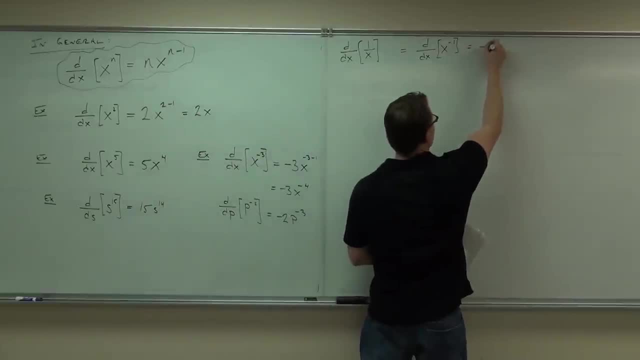 We'll bring down the negative one X to the. what Two? Negative two? Two or negative two, Negative two: You're subtracting one from a negative two And then, because I gave it this way, change it back. We're going to have negative one. 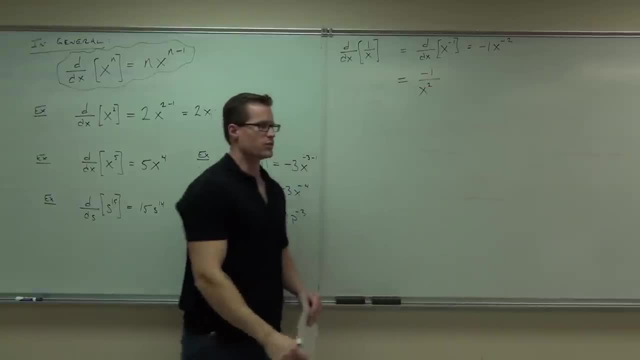 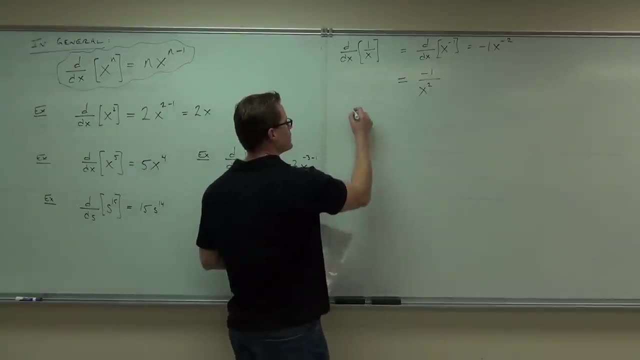 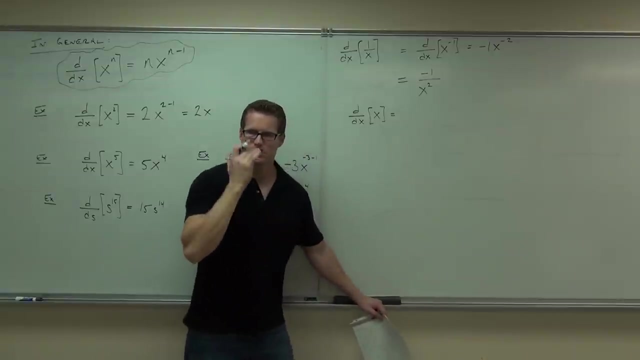 Negative one over x squared. That's the derivative. You okay with this so far. By the way, what's the derivative of just x? One? Some people said x equals one More than one. What's the exponent right now? One? 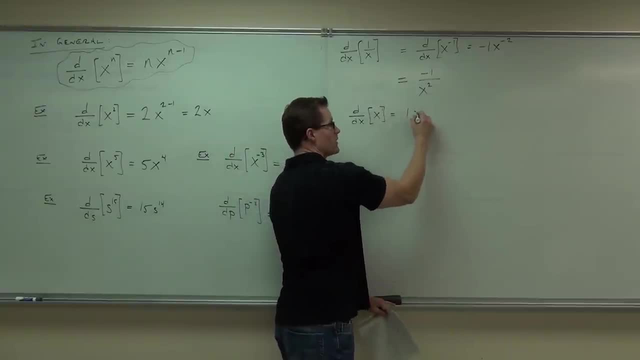 It is one right. So what would happen here is you'd bring down the one. You'd have x to the one minus one, Wouldn't you What's x to the one minus one? So you'd have one times x to the zero. 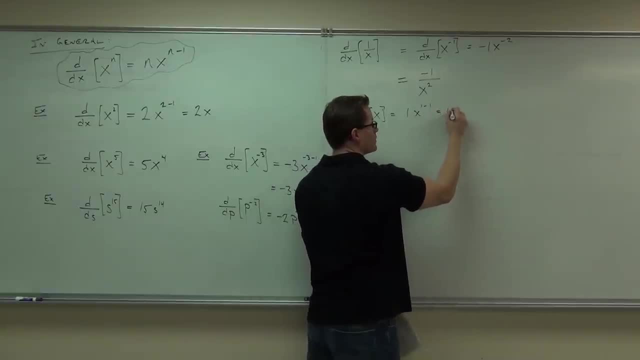 What's x? to the zero One. So this is one times one or one. The derivative of x is one. In fact, if you think about this, think, Think for a second Understand. that's the most basic of all linear equations. yes, 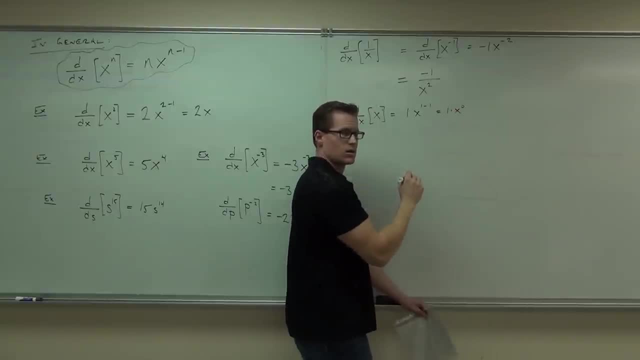 Where we have a non-horizontal, It's x to the first power. What's the slope of this line? One Derivative means slope, doesn't it? So the derivative means slope. So the derivative means slope. The derivative means slope. 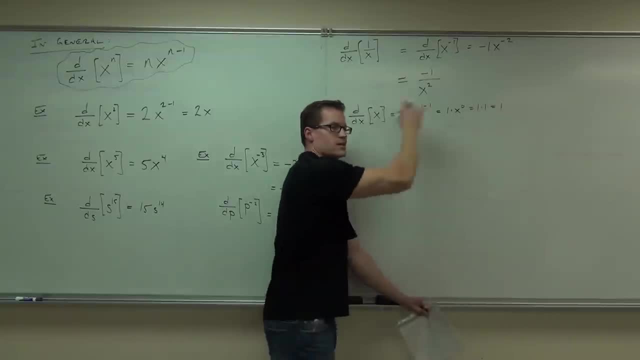 What's the slope of this line? One, The derivative means slope. So x to the one minus one. What's x to the one minus one? One, The derivative of x is one. In fact, if you think about this, think. 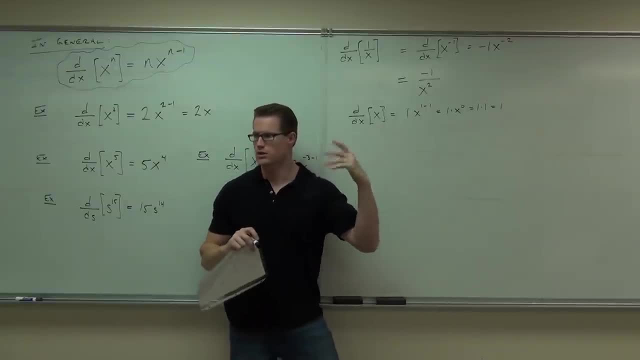 Think for a second Understand. that's the most basic of all linear equations. yes, Where we have a non-horizontal, It's x to the first power. What's the slope of this line? One Derivative means slope, doesn't it? 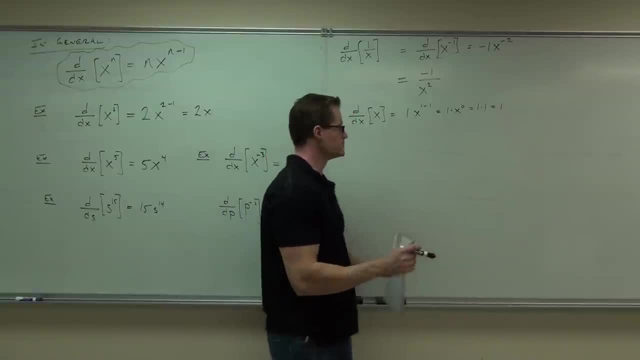 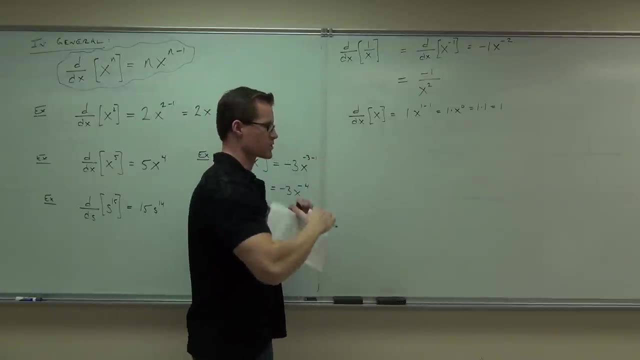 So the derivative would also be one. You can show it with the general power rule. now, How many of you feel okay with so far? All right, another little thing we can do. It's kind of cool. This opens up a whole lot of doors for us. 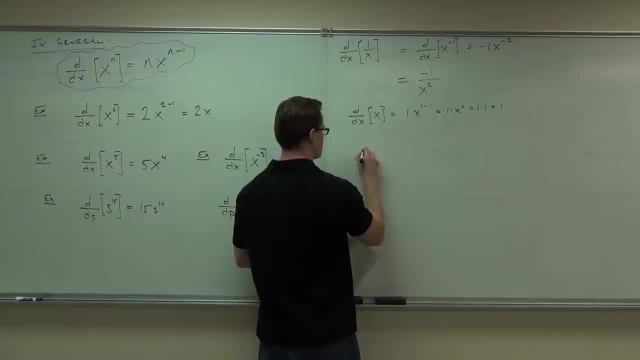 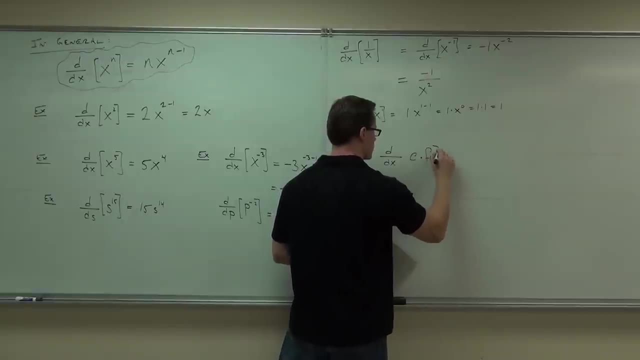 So another note: if you ever have a constant times a function- that could be anything in there- What we can do with derivatives is take that constant and move it out in front of our derivative. It doesn't apply to it. So this is the same thing as c times the derivative. 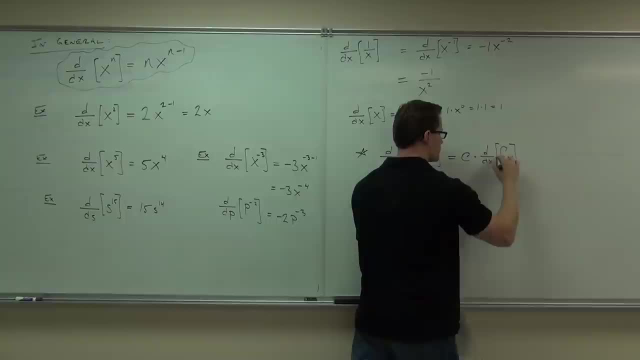 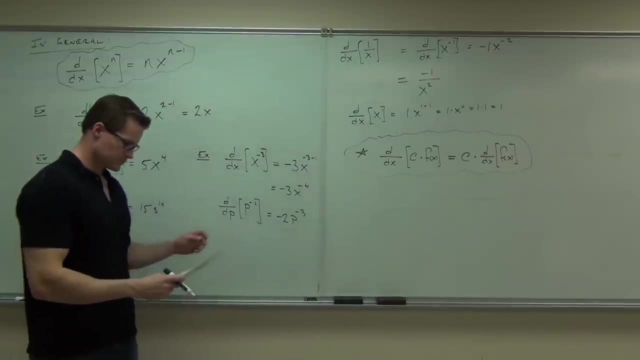 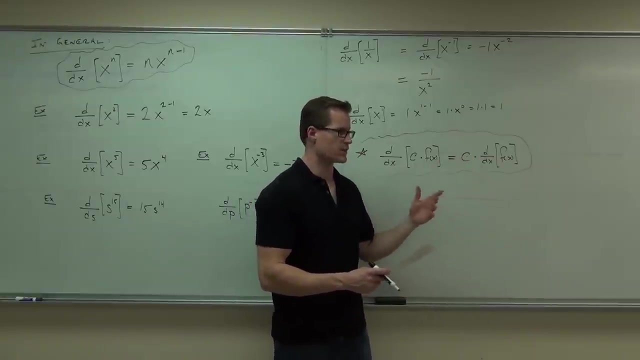 It's the same thing as c times the derivative of f of x, If c is a constant. So make sure you know that c is a constant number. It doesn't change. It's a number like 3 or negative 2 or pi. 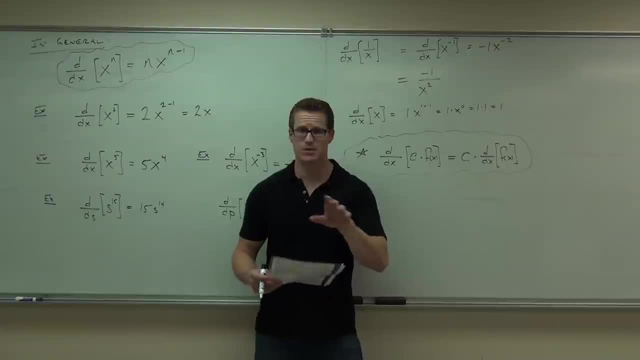 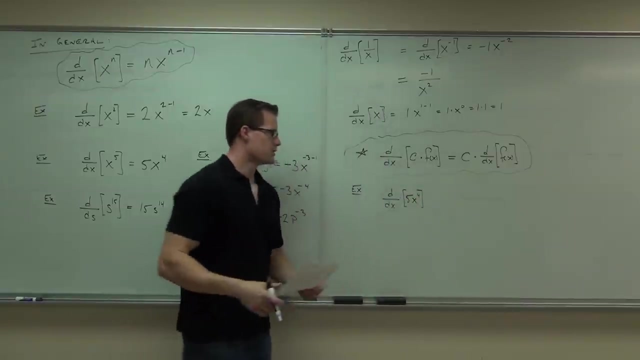 But if we have it being multiplied by that function, we can pull it outside which. I can see a couple examples of this. How about the derivative of 5x to the fourth power? Do I have a constant in there being multiplied by a function? 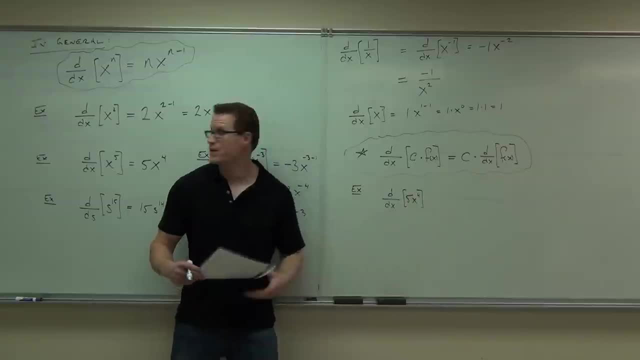 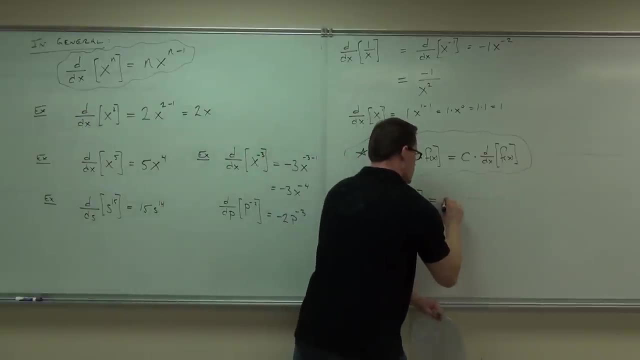 Yeah, 5 is going to be multiplied by x to the fourth. Remember, we kind of want to make it fit that thing, right, Because that's the only thing we know right now. So that's about it. So you know, you can make this 5 times the derivative. 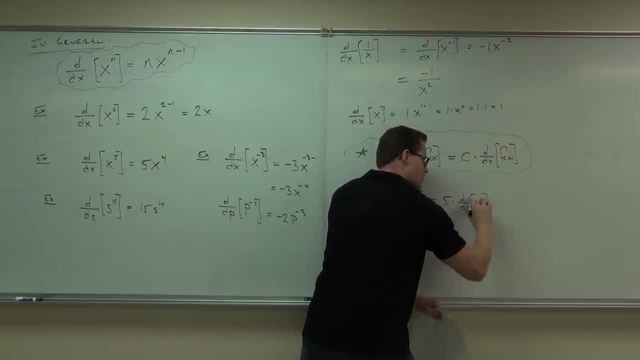 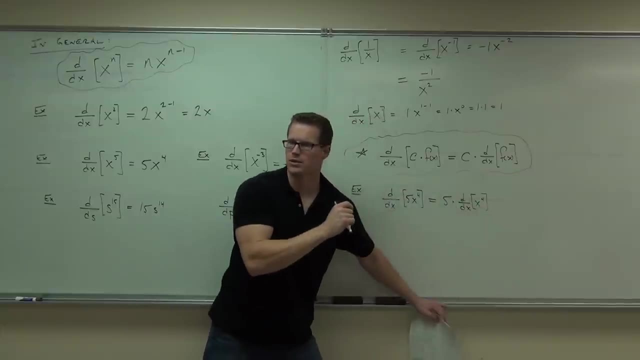 of 5x, x to the fourth. We can take that constant number and multiply it by the derivative of the function itself. So what's the derivative of x to the fourth power? please, 4x to the fourth. Don't forget about the 5.. 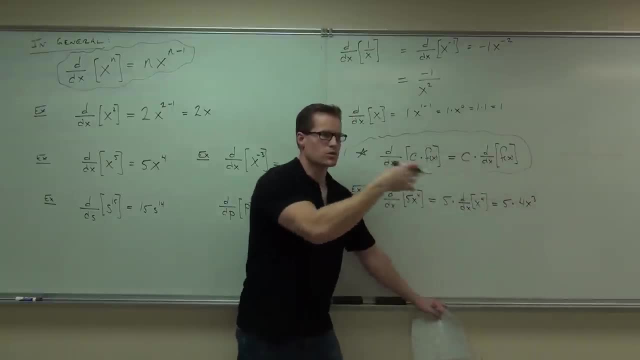 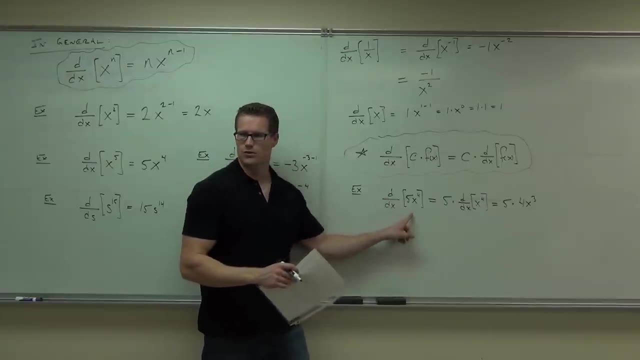 But then you have 4x, sure, to the third power. Now you can do the 5 times the 4.. How much are you going to get 20 times the third? Yeah, sure, Now look Practically, can you get 20x to the third from here. 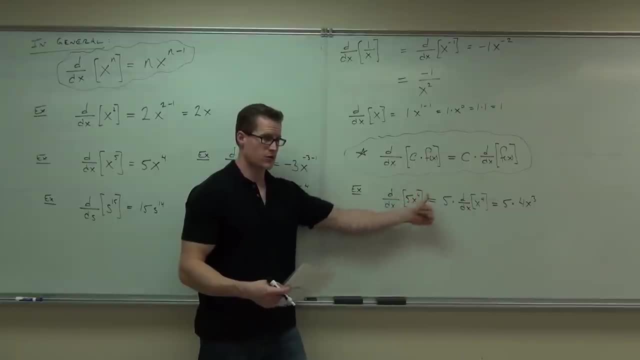 Yeah, Absolutely. You bring down the 4,, you multiply it, times the 5. You're going to get the 20, right, Yeah, Are you following me on that? Mm-hmm, I haven't outpaced you yet. 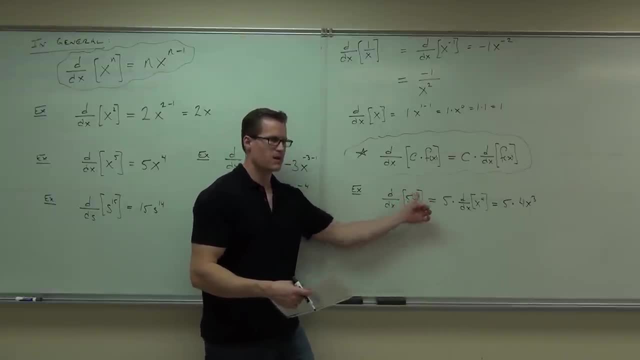 No, All right, cool. If you bring down the 4, which you know you're going to be doing, multiply it by the constant term. you're going to get the 20, and then subtract 1 from the 4.. 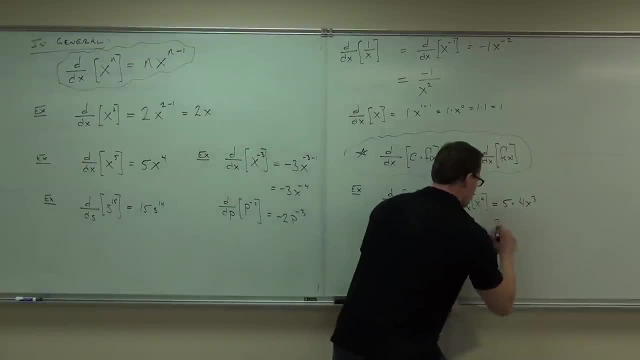 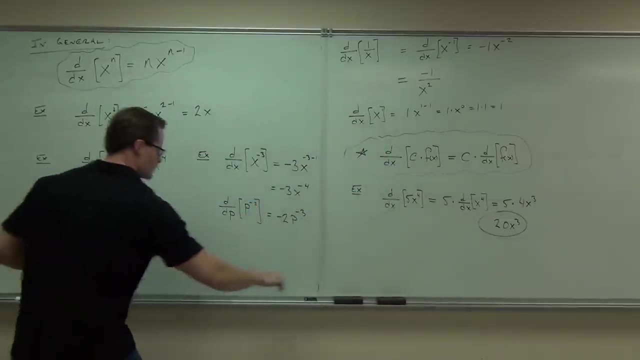 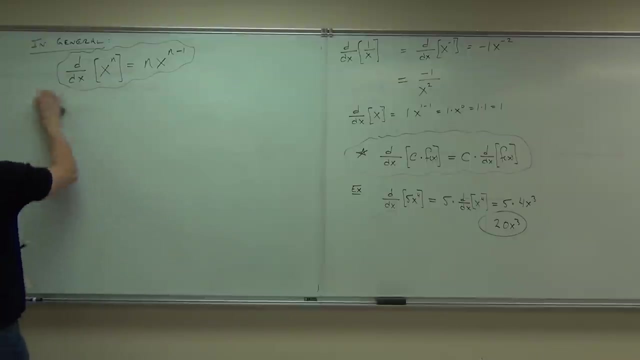 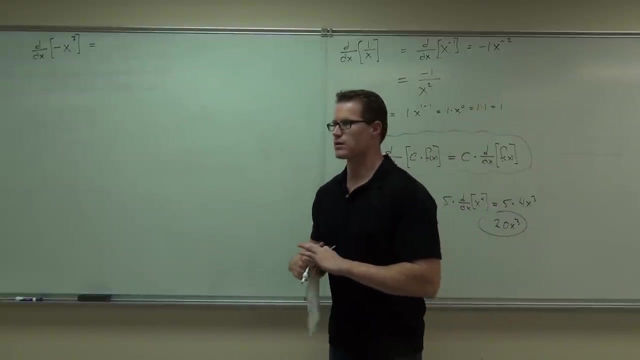 You're still going to get 20x to the third power. How about the derivative of negative x to the seventh power? What do you think? What can we do? Do we have a constant in there? Yes, So we could pull that constant out of that negative. 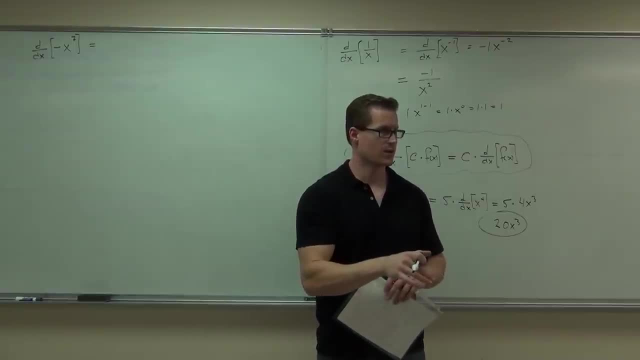 then take the derivative of x to the seventh. Can you take the derivative of x to the seventh? Yeah, All of you should be able to at this point, At this point, right, So we can do that. But basically I'm showing this to let. 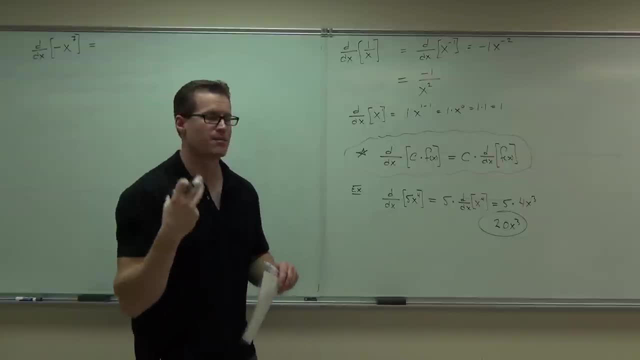 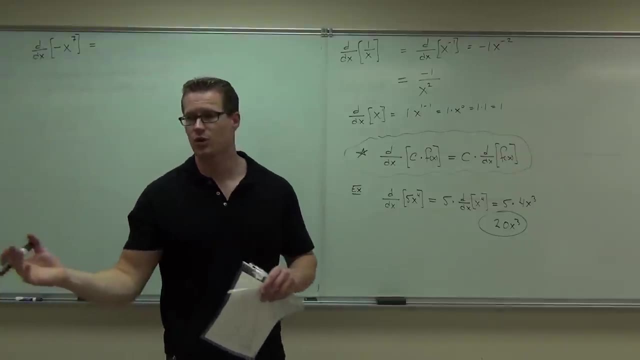 you know that if we can pull the constant outside of it, you can just multiply it by the exponent. So in our case, right here, can you tell me the answer? with just doing the derivative of negative x to the seventh, What are we going to get? 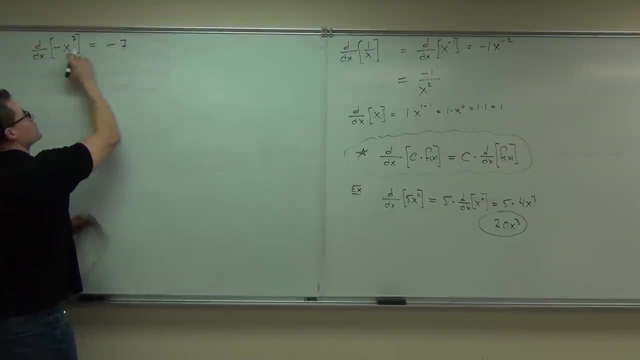 Negative 7.. Sure, You know that's a constant. You'll be multiplying it later. Negative 1, that's negative 1, times positive 7, that's negative 7,. x to the sixth power. you're done. 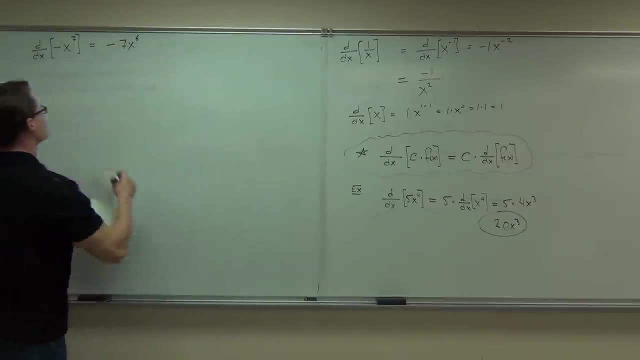 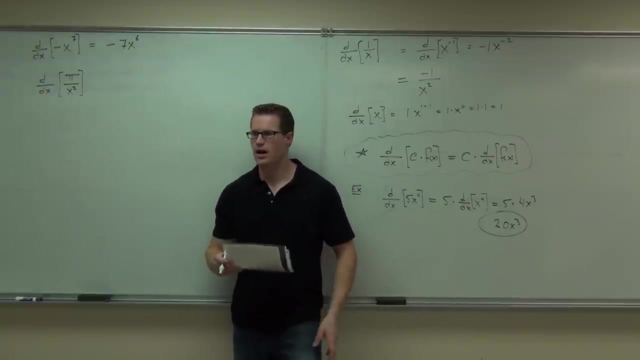 That's your derivative there. How about let's do one last one, The derivative of pi over x squared? Pi over x squared. What do you think? Is it pi over 2x? Pi over 2x? Can you do that? 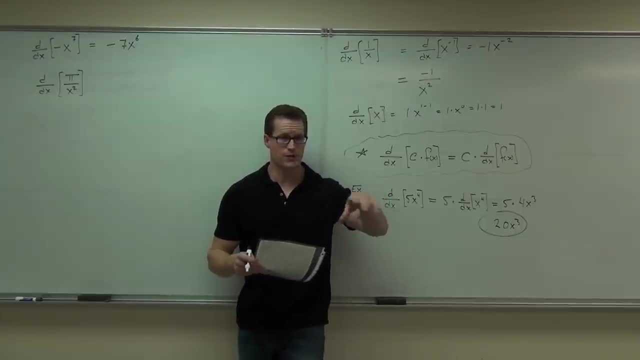 Can you do pi over 2x? No, That doesn't fit Right. That doesn't fit the power rule that I gave you just a minute ago. It doesn't fit that. What would you have to do to the x squared before you can do that stuff? 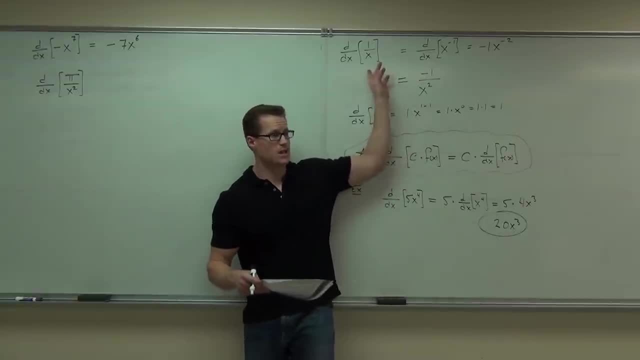 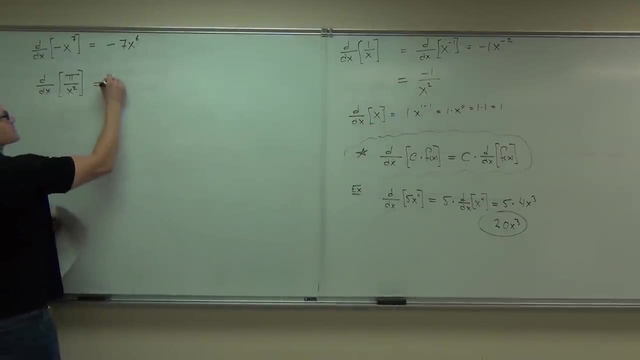 Just what you did here. Same thing you did that You've got to make it this format, otherwise you can't touch it. So right here we've got to say, all right. well, I know that this is the same thing as. 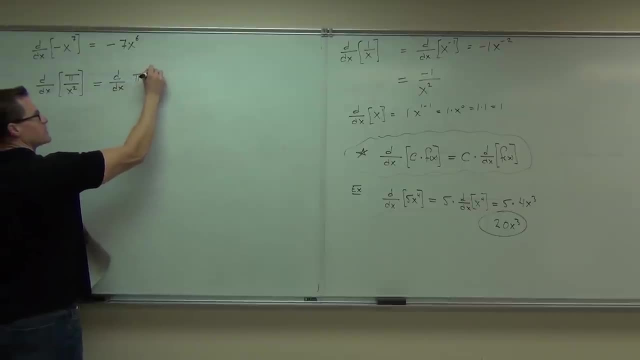 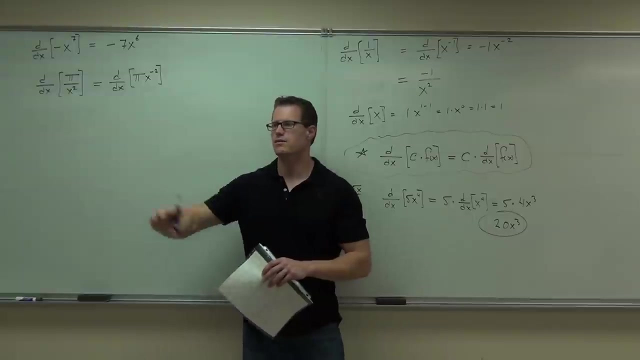 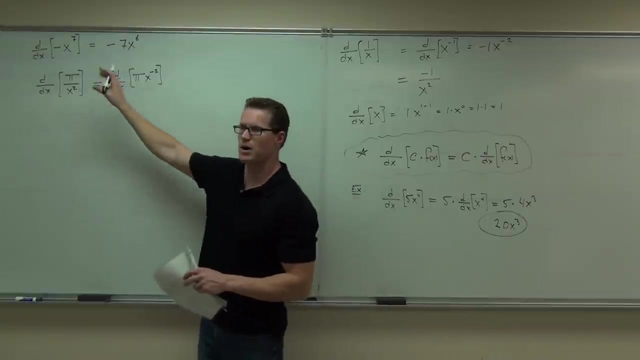 dvx. pi x to the negative 2.. Are you with me on that or no? Move your exponents up and make them negative. That way you can use that power rule that I showed you. Otherwise you can't do it. This in no way is equal to pi over 2x. 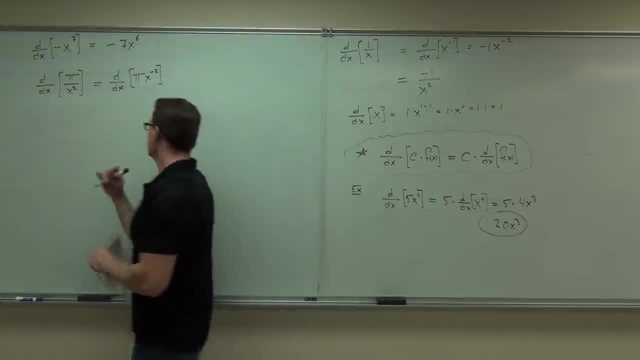 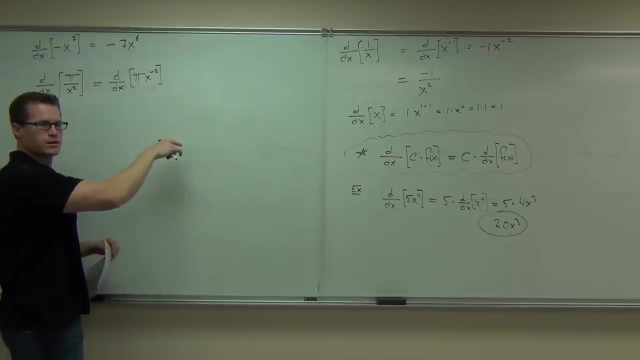 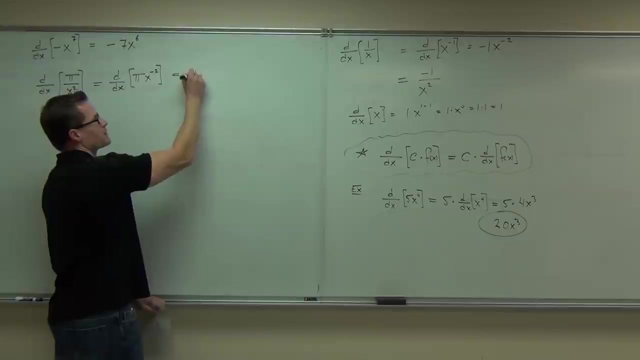 You can't just do that Now. what's next? What do you think? We could pull out the pi if you wanted to, or you could leave it in there if you wanted to. It doesn't really matter. If you pull out the pi, you'll have pi times ddx of x to the negative 2.. 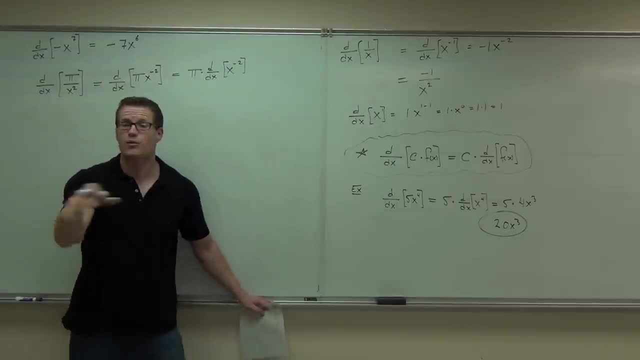 Now can you take the derivative of x to the negative 2?? Yeah, now it fits right. Now you can do it. You can pull down the negative 2.. Take 1 away from that exponent, You're going to get the negative 2x to the negative 3, and then multiply by the pi. 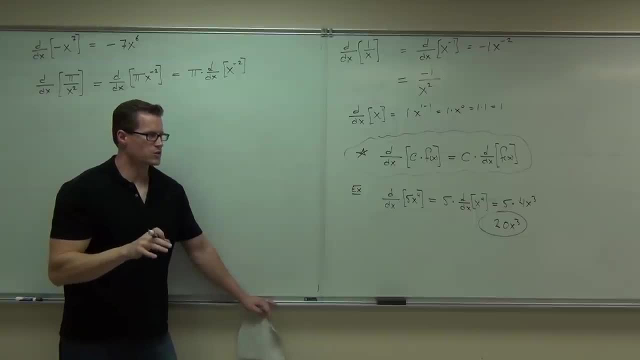 By the way, stop for a second. You know how I told you the derivative of a constant is always 0?. A lot of people ask later: well, wait a second. If the derivative of a constant is always 0,, why don't we get a 0 here? 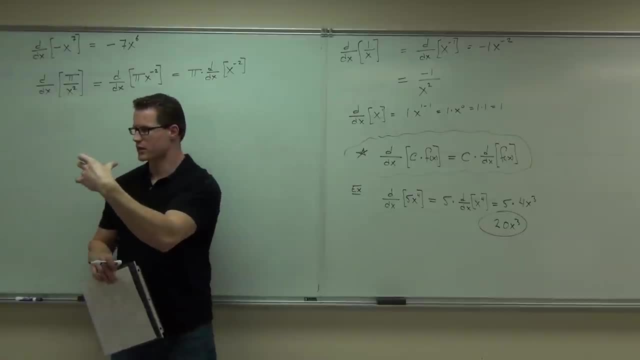 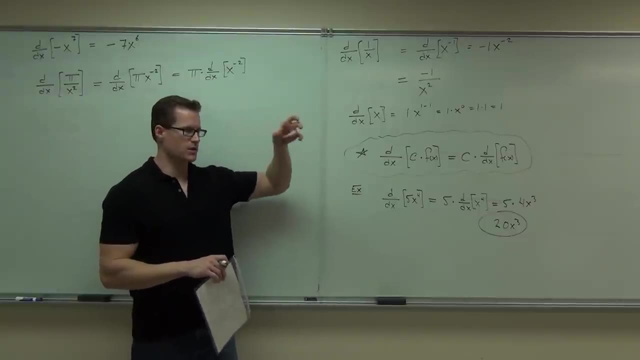 Why don't we do that? Well, that's actually connected to something with a variable, right? If you have a constant by itself, like the derivative of pi, that was 0. However, If you have a constant being connected to that variable, we can pull that outside by. 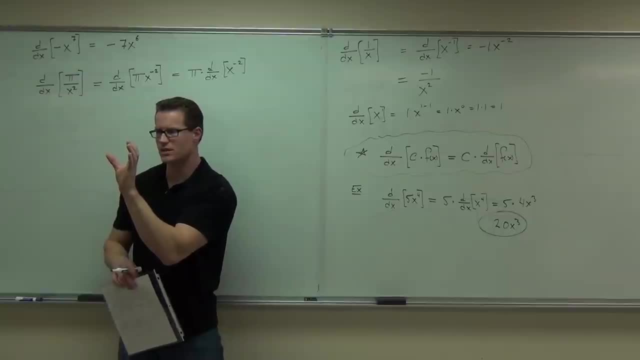 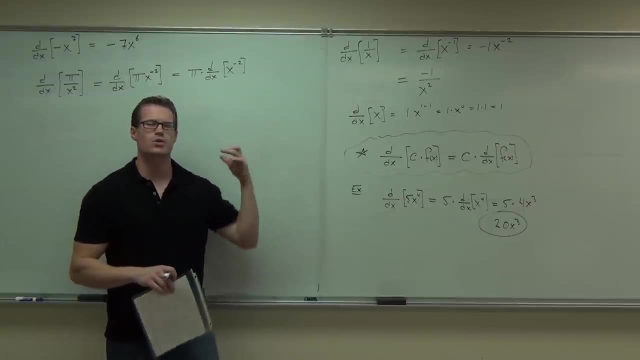 multiplication. So basically it just hangs around and says, no, it's not 0.. I will show you that. yes, a derivative of a constant, it is 0. But if you did that, you'd have to show something called the product rule here. 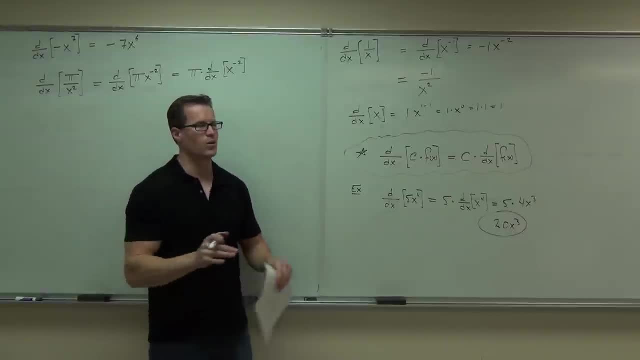 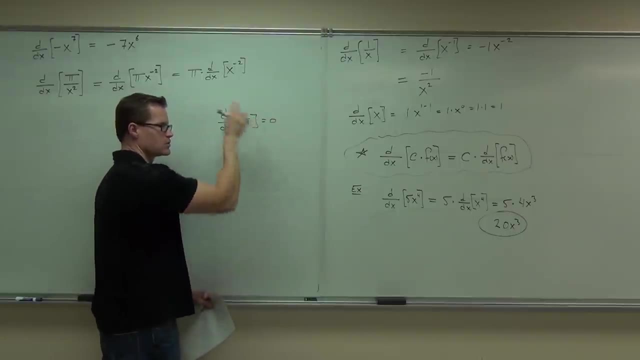 I'll talk about that in the next section, But for right now you go: OK, well wait. A derivative of a constant by itself, yes, 0.. As soon as you connect it to a variable, that now is just a constant being multiplied by. 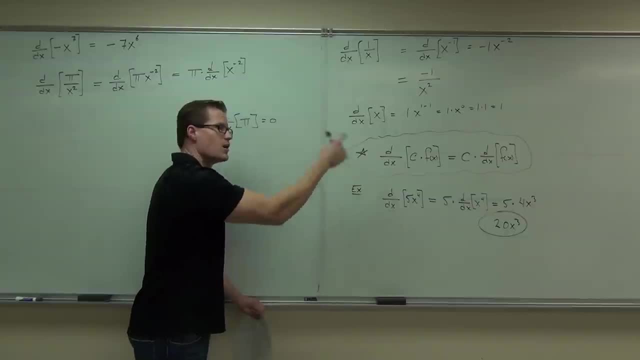 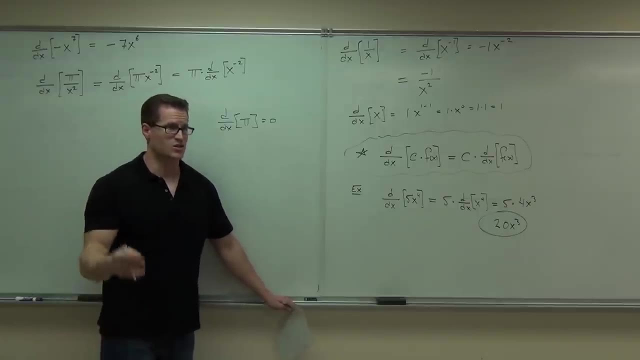 that variable. You can pull it out front. You can use that rule that I showed you, then take the derivative of the function and multiply it back. Does that make sense? Otherwise, all of your derivatives would end up being 0, and that would say the slope. 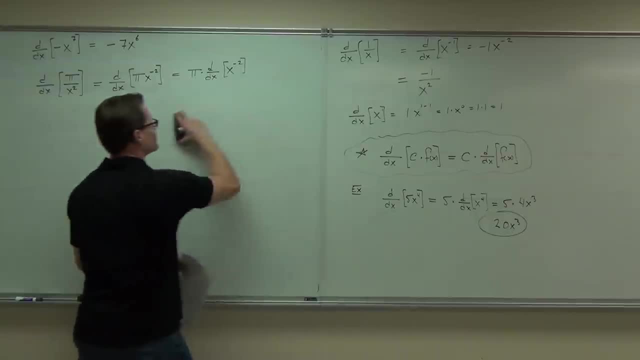 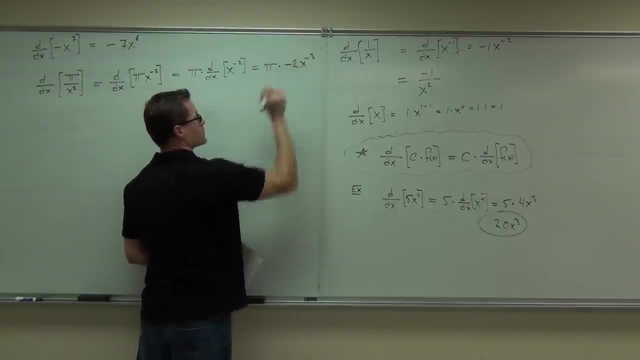 of everything is 0. That's not true. So here you have the pi times. well, you all told me it was negative 2, x to the negative 3.. We bring it down, We subtract 1.. And if you really wanted to kind of pretty this thing up a little bit, you'd make it. 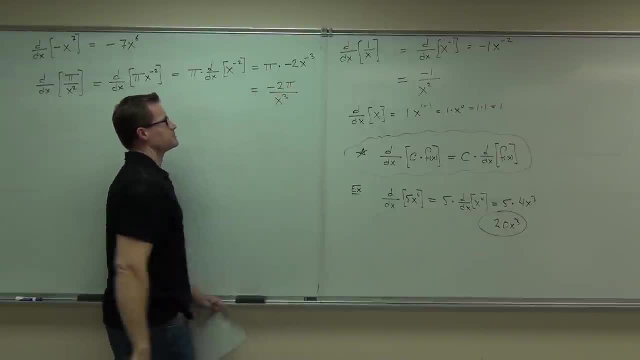 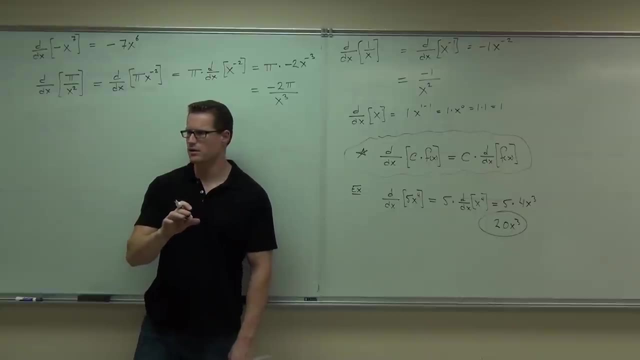 negative: 2 pi over x to the negative. 3. Over x cubed. Do you see how to get to the negative 2 pi over x cubed? Nod your head if you can Feel, all right with that. OK, And that's our derivative. 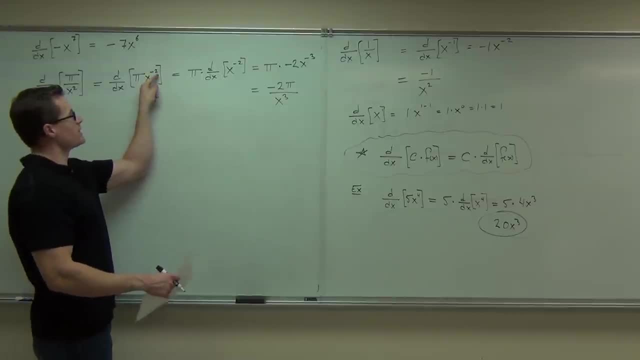 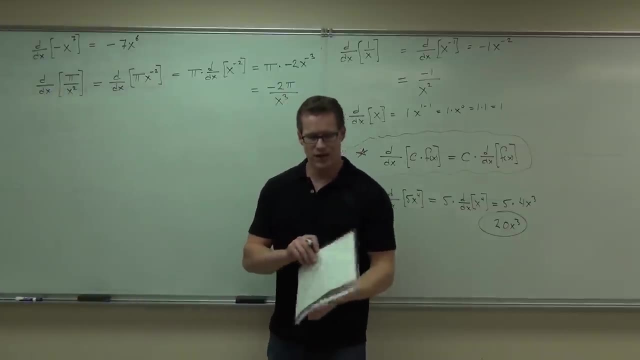 Could you have got there directly from here? Sure, Sure, You bring down that negative 2.. That's the negative 2 times pi x to the negative 3, you can do that, By the way. a couple of nice little rules for us. 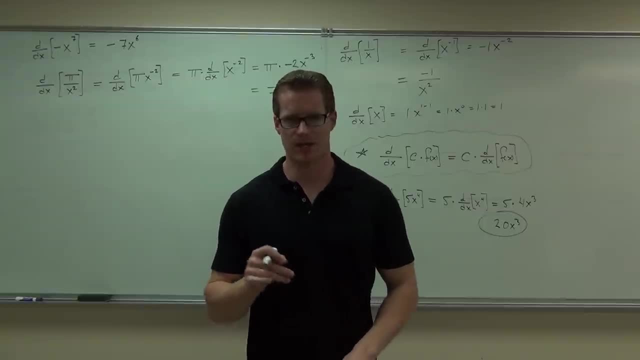 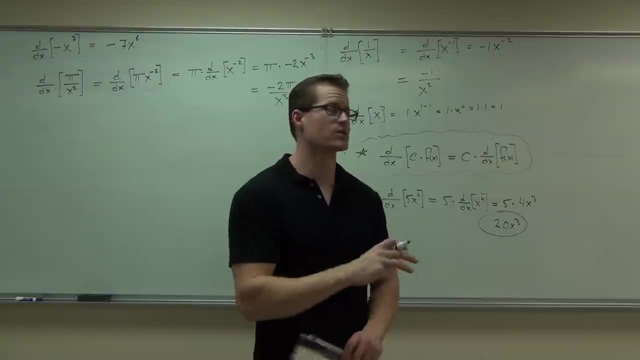 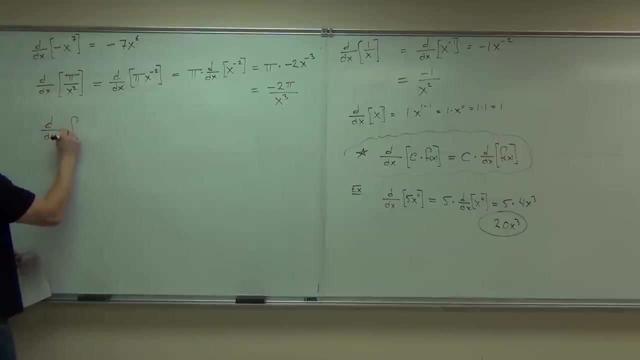 Just like we could do with limits. you see, when we're finding derivatives, we're actually finding limits. right, With limits, you can pull constants out. With limits, you can separate by addition and subtraction. True, You can do the same thing here. 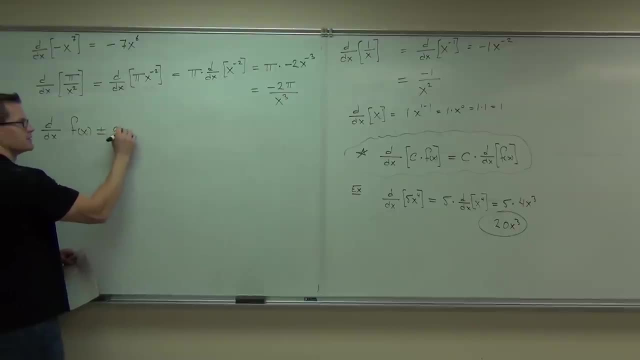 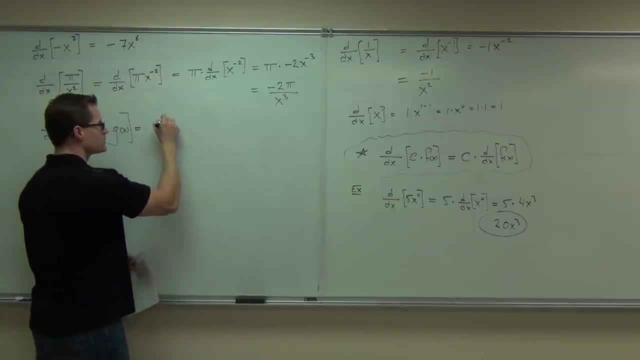 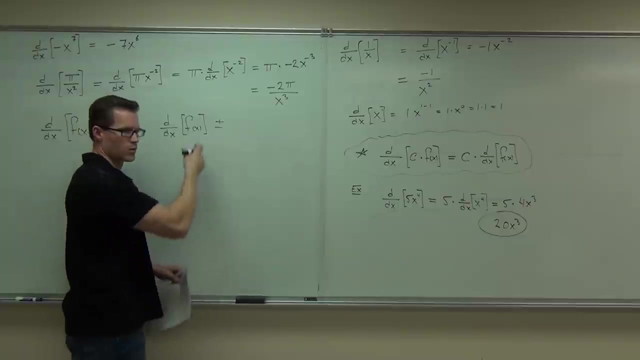 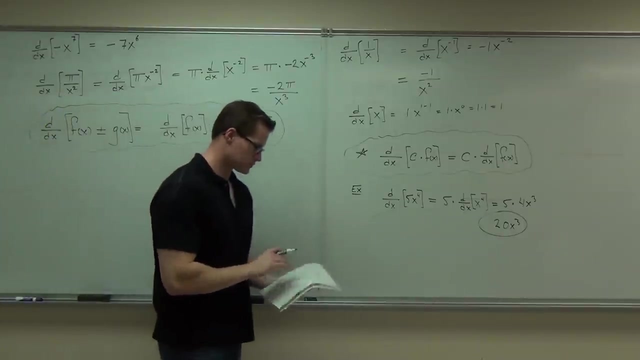 If you have the derivative of a couple functions being added or subtracted, that's the same thing as the derivative of the first function. OK, Plus or minus. if you're using subtraction, the derivative of the second function. You ready to see how we can apply this to some problems? 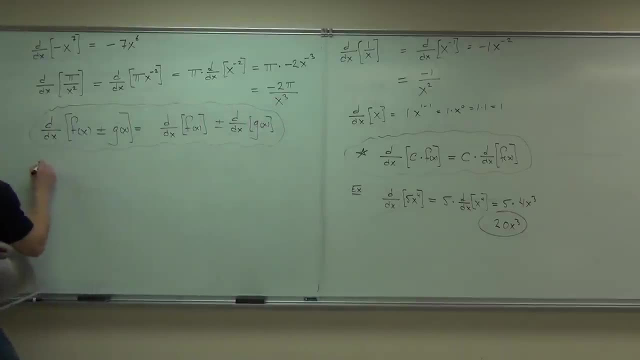 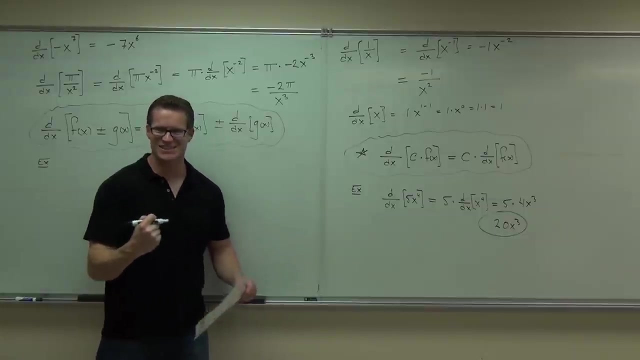 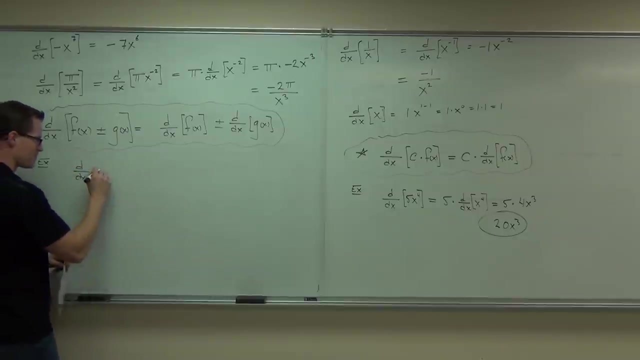 OK, Now check this out. OK, This should be like a booyah moment for you, like, yes, I got this, No more limits, Bam Done. Because if you had to do- oh my gosh, if you had to do this problem with limits, see, 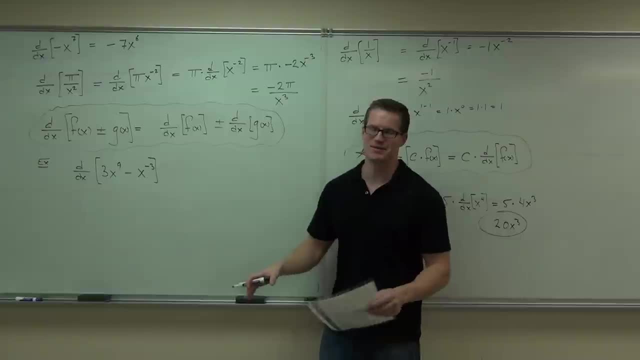 you all. next week, I'll go home for four days and you can just work on that. Well, it would take a week, But it would be pretty difficult, wouldn't it? Because remember what you'd have to do to find the derivative. 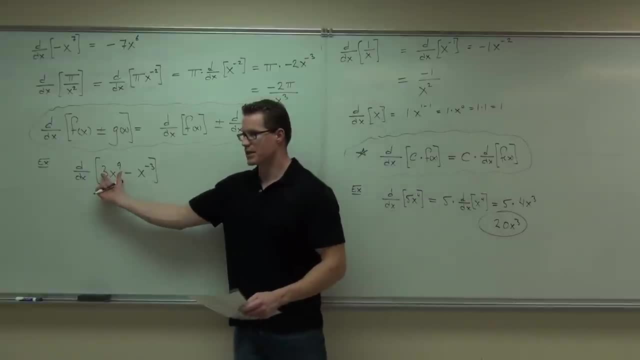 You'd have x plus h and x plus h in here and subtract the whole thing. You'd have to find some common denominators because you have this negative exponent. You'd have some pretty nasty work to do on this thing. Very nasty work. 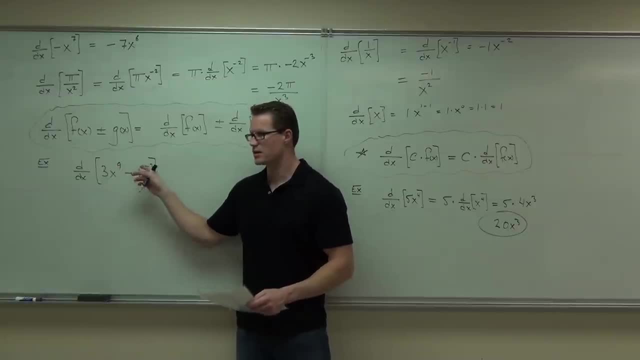 However, using what we now know about derivatives, if we can break all this stuff up into individual functions being added or subtracted, take the derivative of each one and put them back together. we're good to go. I mean, that's not bad at all. 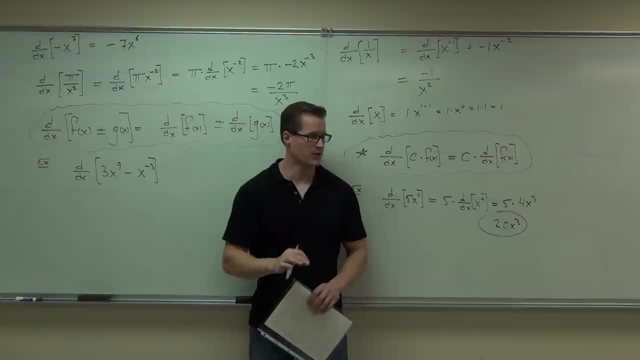 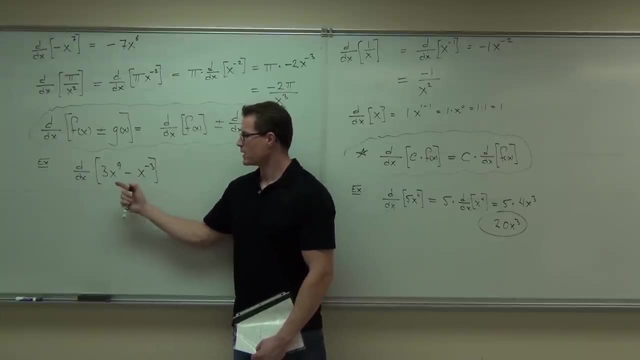 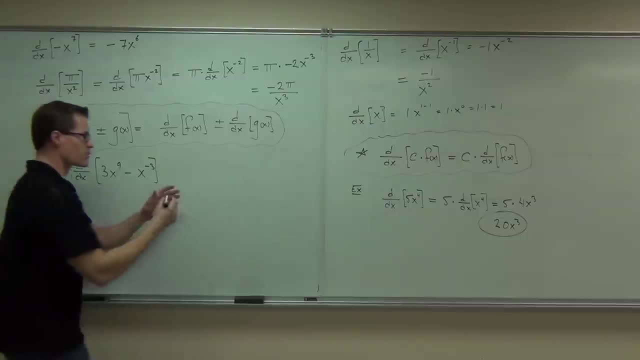 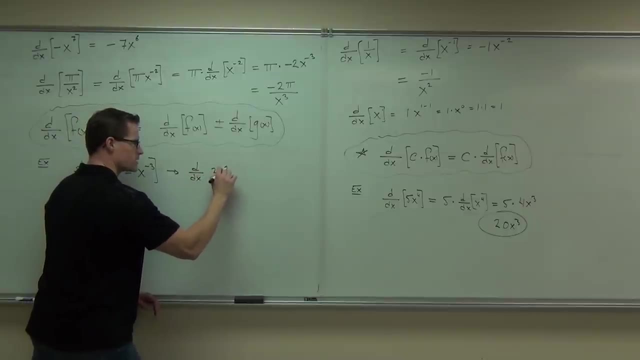 OK, OK, Let's go slowly through this. I really want you to get this. Yeah, you can. You can separate addition and subtraction. So this is the same thing as the derivative of 3x to the ninth, minus the derivative of. 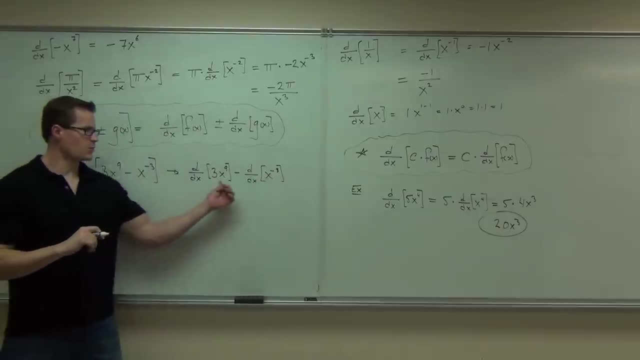 x to the negative 3.. Are you OK on that set? Tell me one thing you could do with this. Is that legal to do? Can you pull the constant out? Yes, We could do that. The constant doesn't become a 0.. 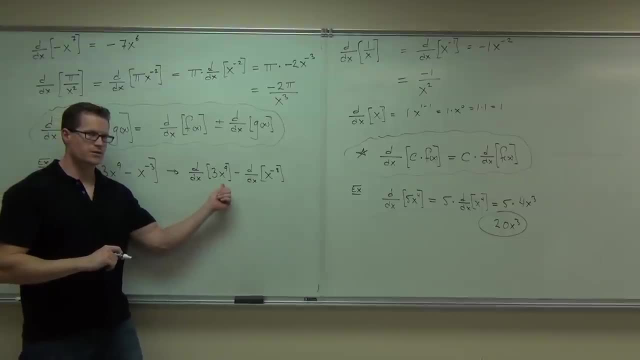 It's connected by that variable. Could you just take the derivative the way it is: Mm-hmm. OK, Let's try that. What's the derivative of 3x to the ninth? everybody? What is it? 27x to the eighth? 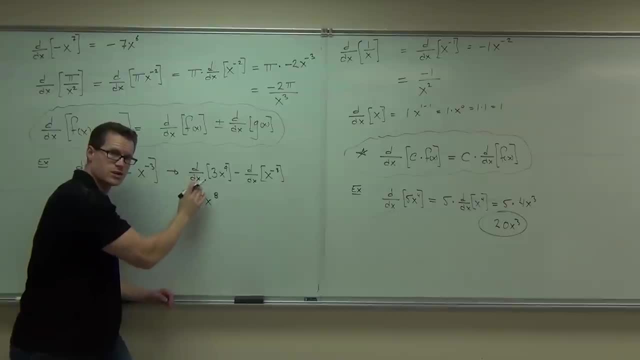 Good, Bring it down. You're multiplying that 3 times 9 gives you the 27.. x to the eighth Sure. We're subtracting 1 from the exponent, Then I have my minus sign. What's the derivative of this one? 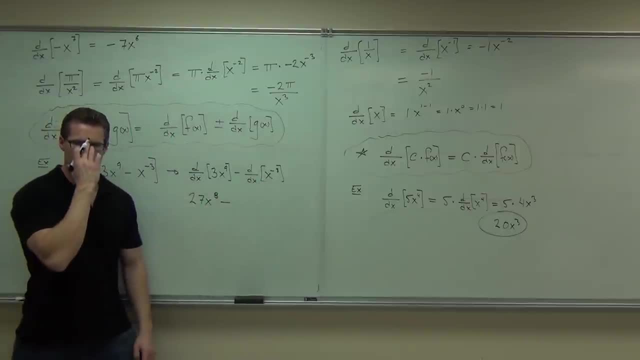 Negative 3x to the negative. 4. Negative 3x to the negative. 4. Positive 3x to the negative. 4. Negative 3x to the negative. 4. Negative 3x to the negative. 4. Positive 3x to the negative, 4.. 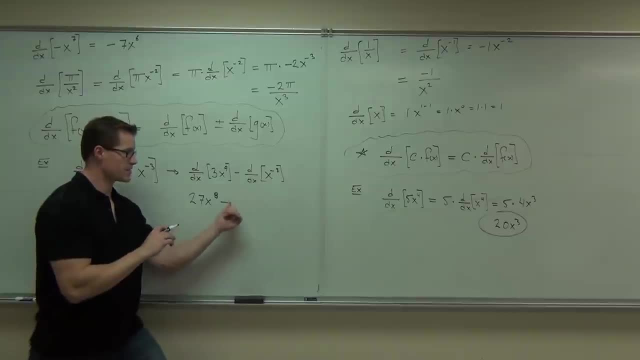 Positive 3x to the negative 4. Positive 3x to the negative: 4. It's going to be ultimately. yes, you're right, But since I have this minus sign right here, what's the derivative of just that piece? 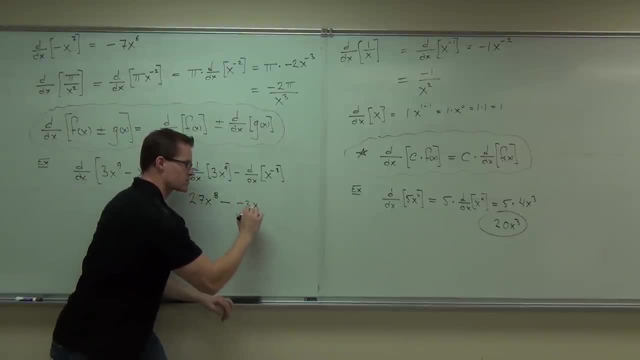 Negative. 3x to the negative, 4. x to the what Negative? 4. Good, I'm subtracting 1. Remember that's in parentheses, because I'm subtracting that whole derivative. there Minus and negative becomes a. 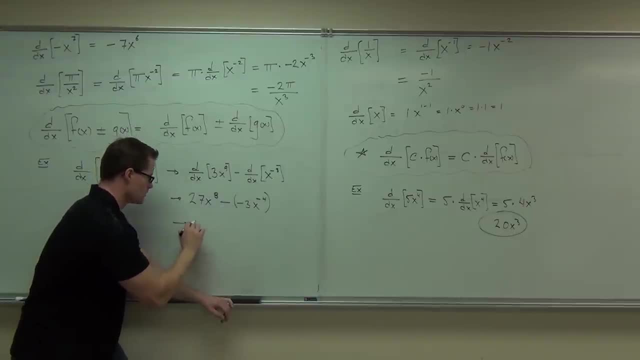 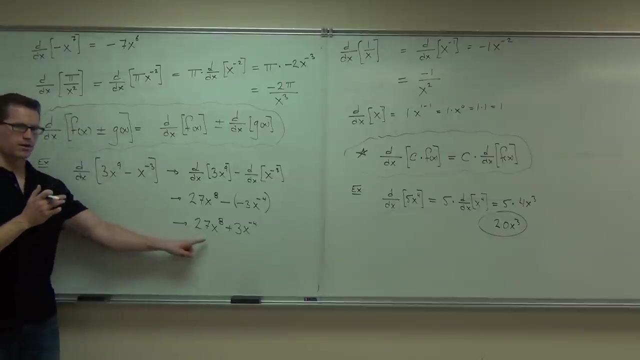 Positive. Does that look okay to you? Hey, quick question. Could you get there directly from here? Sure, What's the derivative of 3x to the ninth? It is 27x to the eighth, Minus the derivative of 3x to the negative 3.. 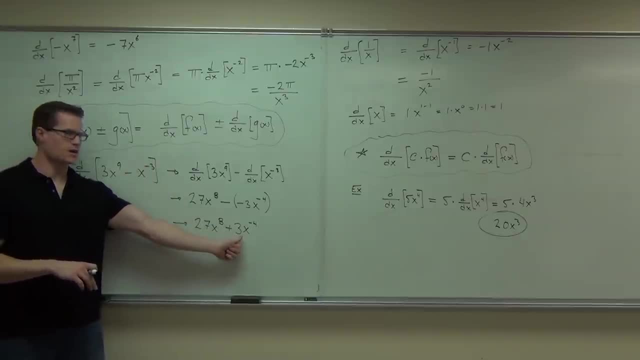 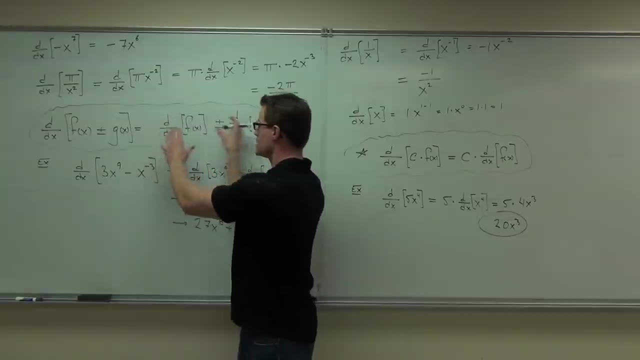 Negative times. a negative gives you a positive 3x to the negative 4.. Can you get that on your own as well? Sure you can. What I'm letting you do here is I'm showing you. sure you can do this. 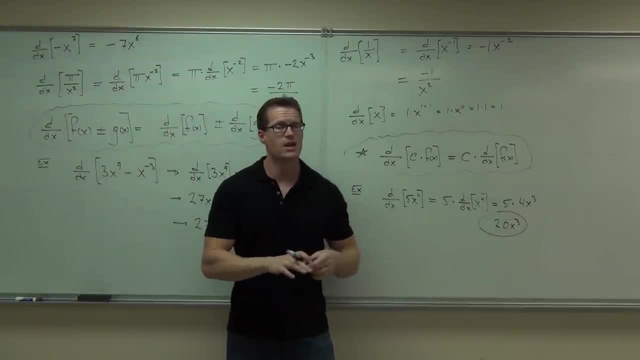 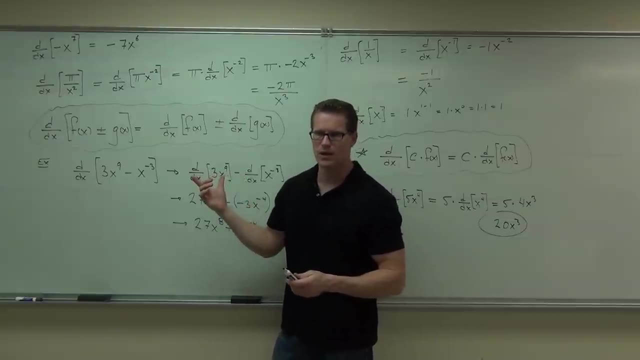 It's legal. Therefore, what that allows you to do in your calculus is take derivatives term by term. That's what it allows you to do, So do you need to split this up for me? No, No, you're not going to do that. 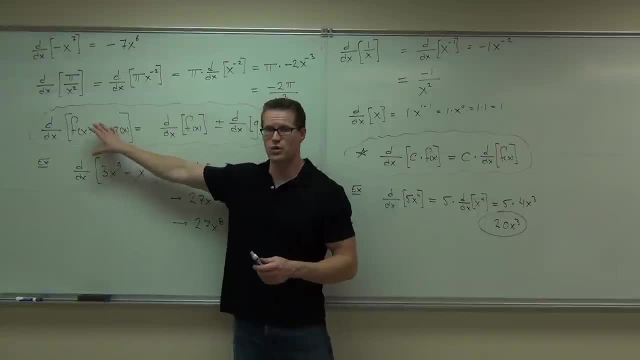 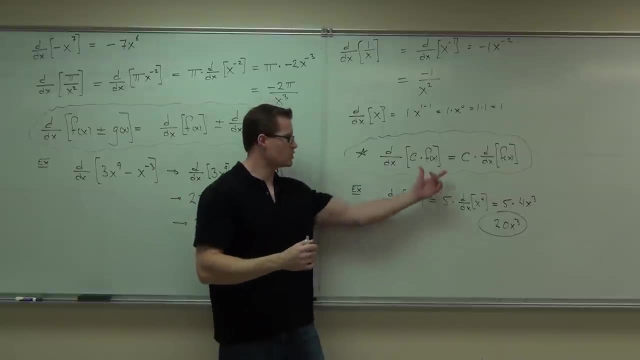 What you're going to do is look at this and go: okay, Mr Leonard said by this rule, split it up by addition and subtraction- that I can split them up. That means I can take derivatives term by term. Since I could pull a constant out, that means I'm just multiplying it. 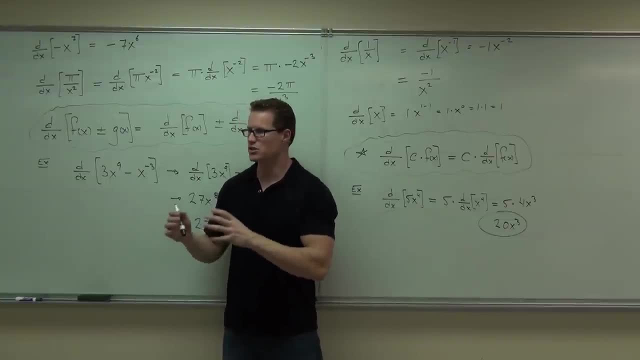 So do I need to show that? No, you don't. It's just saying it's legal to do. That means that when I look at it, it's legal. When I look at this, I go: okay, I know that constant's going to end up being multiplied. 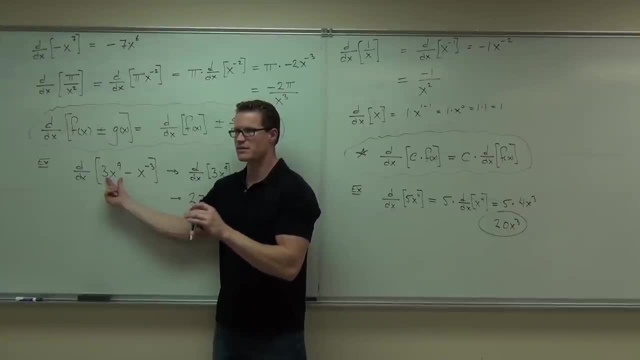 by the derivative of x to the 9th. The derivative of x to the 9th is 9x to the 8th. When I multiply the 3 times the 9,, that's going to be the 27.. This says okay minus. but I'm going to have a negative there. 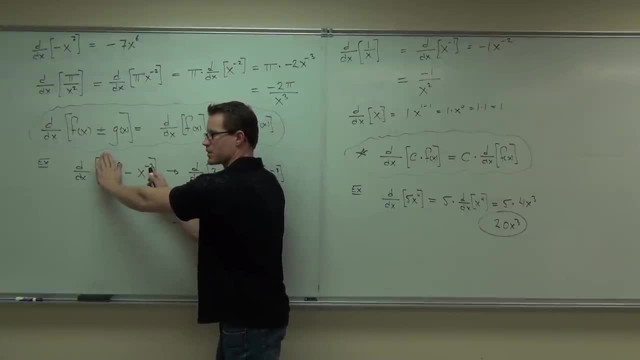 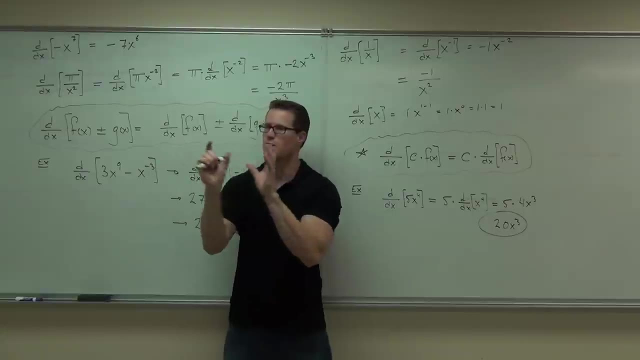 Or if you consider this as one term, negative 1 times negative 3, that's going to give you the positive 3.. Then that x to the negative 4 comes in the fact that I can take this derivative by itself, term by term. 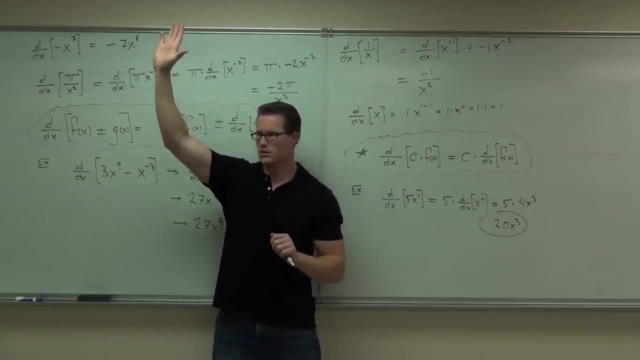 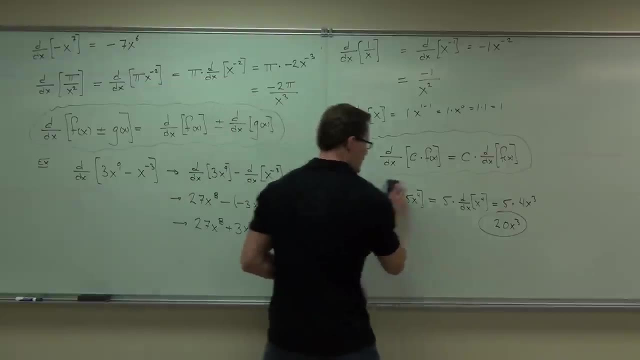 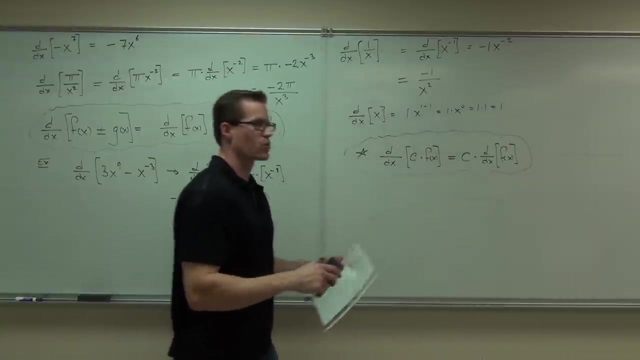 How many people feel okay with our example so far? Good, Okay. Would you like to see one more? How about two more? Yeah, we'll do two more. I'll show you an application of it. We'll talk about higher order derivatives and that'll be our day. 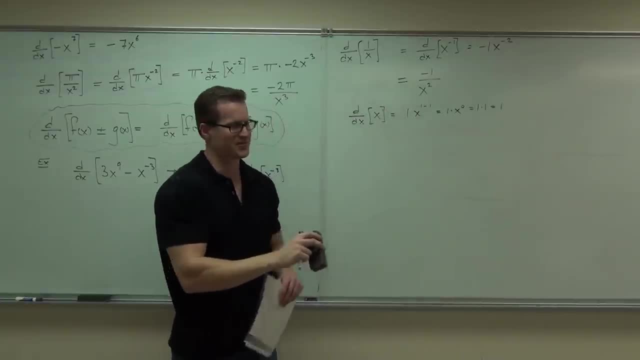 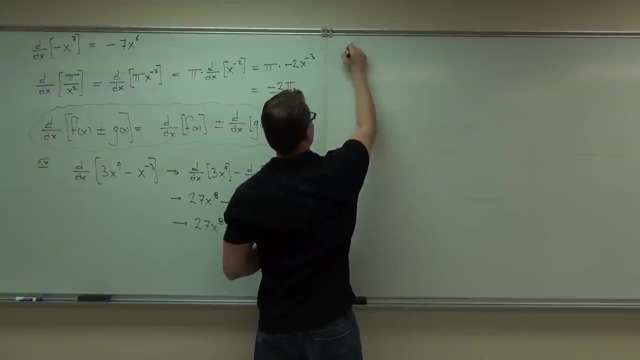 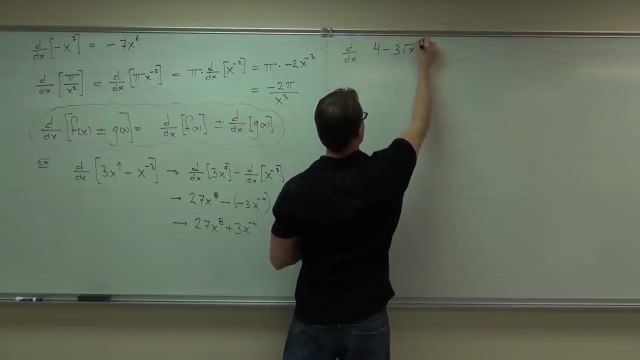 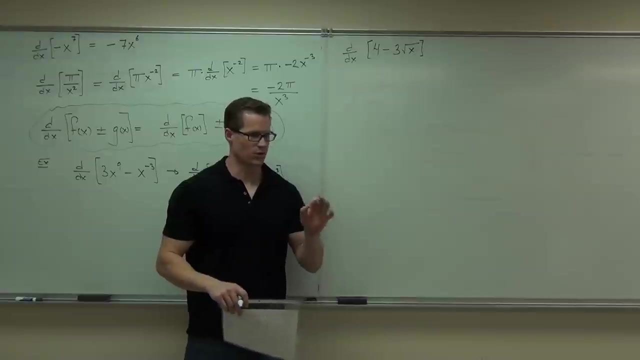 I know higher order derivatives sound much worse, but they're not. You'll like them. I promise You'll like them. I'm going a little bit beyond this section for a reason. I want to show you that this is actually true. 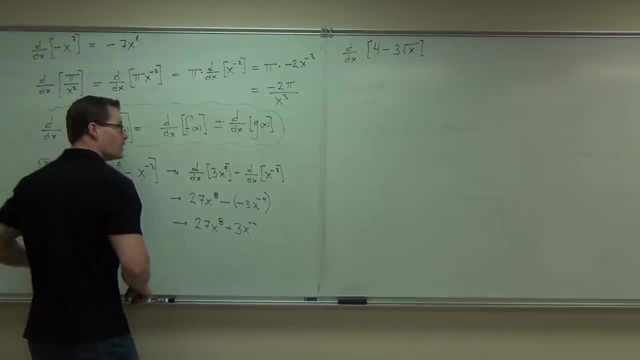 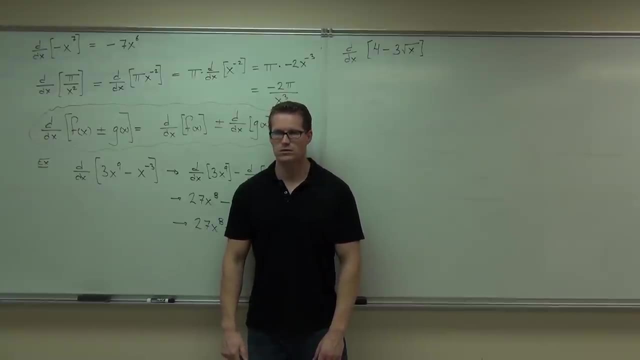 Have we fit our format yet? Have we fit that? No, What's wrong? Square roots are problems for us. Square roots are problems because they don't have an exponent. Can you make them have an exponent? No, Can you make them have an exponent. 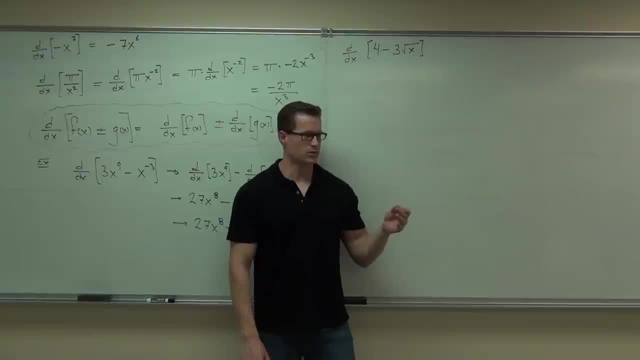 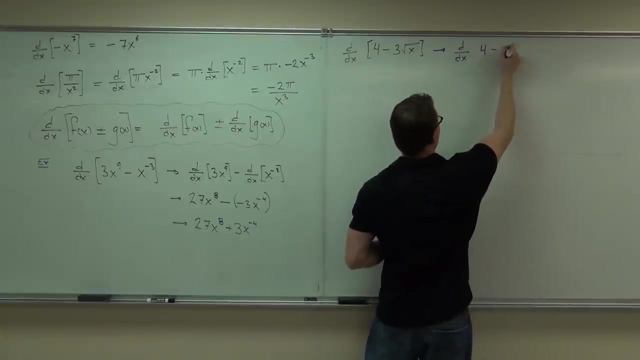 Yes, What is the exponent Power over root? It's always power over root. So the root is 2.. The power is 1. That means x to the 1 half power. So if this becomes a derivative with respect to the variable x, 4 minus 3x to the 1 half, 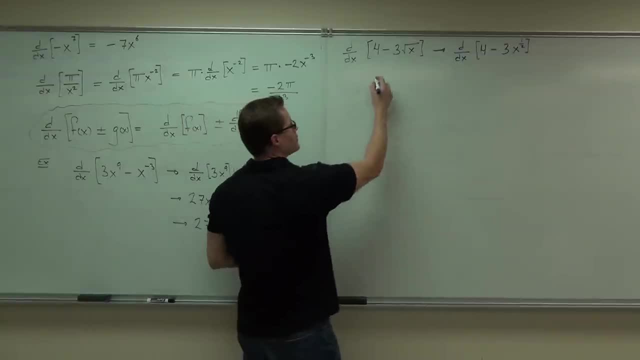 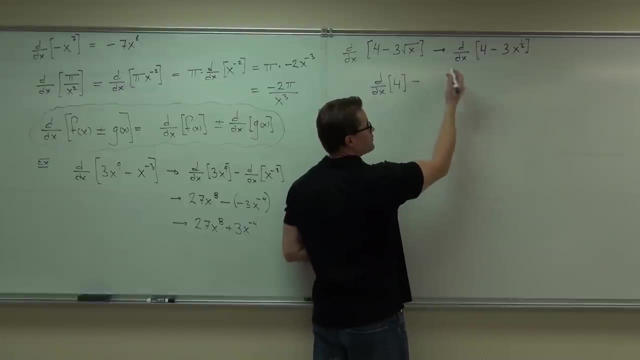 This is the last time I'll show you how to break it up. You could break this up as a derivative of 4 minus 3 times the derivative of x to the 1 half. Do you see how that's legal to split that up? 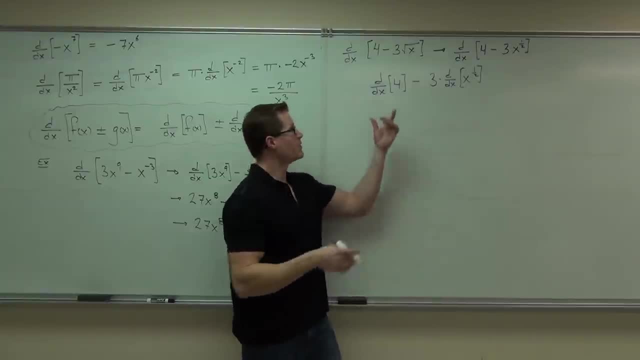 We can split it by subtraction. We can move constants out in front of it. This is a very easy derivative to take. What's the derivative of a constant number? Notice the difference here. This is not connected by a variable right. This is just the derivative of the constant. 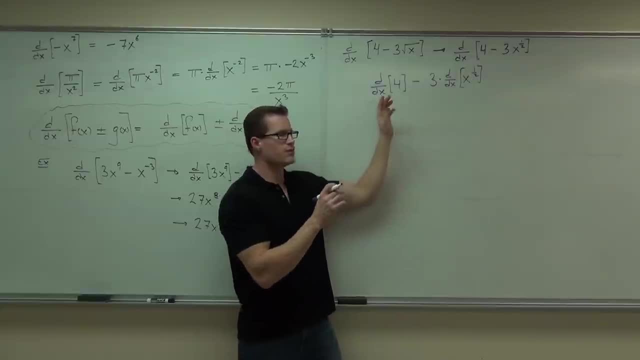 This is the derivative of the constant itself And I pull that out, Even if I were to do this and say: well, wait a second. Mr Leonard, Did you say I could pull the constant out in front? Didn't I tell you that? 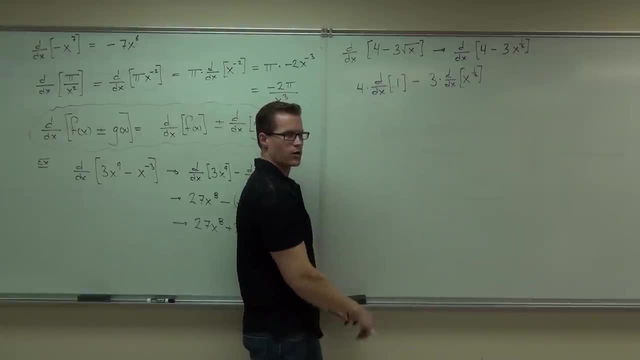 You'd still have a 1 in there, right? What's the derivative of 1?? 1 is still a constant. 4 times 0 is still 0.. The variable affects your problem. That's what it does. The derivative of a constant gives you just 0. 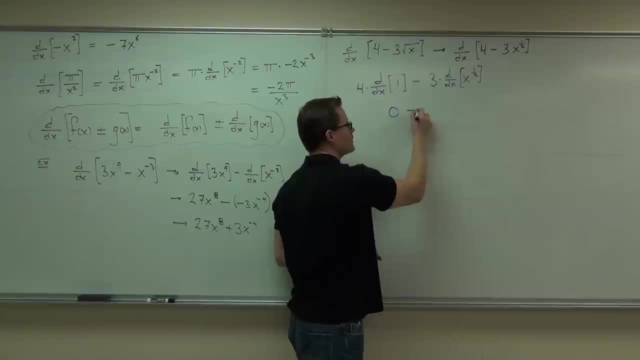 So this is 0.. Don't forget that's a minus. Notice that, Are you okay? We're getting here to here, separating them and pulling the 3 out at the same time. You'd have that 3 times…. Let's do the derivative of a fractional exponent. 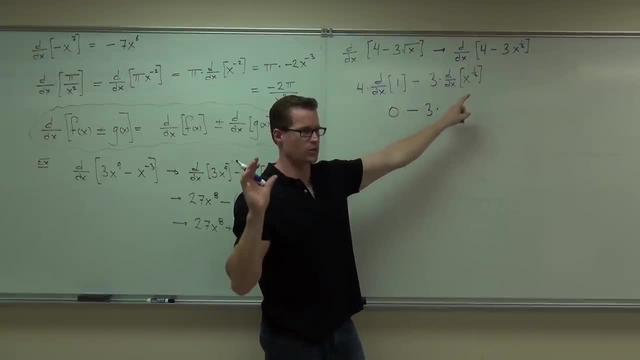 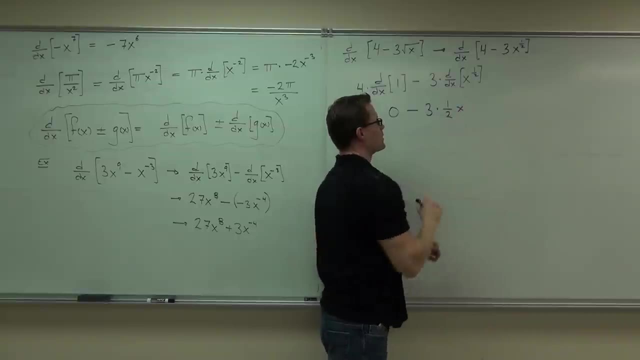 It works exactly the same way as any other power rule. So can you bring down the 1 half. Bring that down first. 1 half x to the…. Can you subtract 1 from 1 half Negative, 1 half, Yeah, 1 half minus 1.. 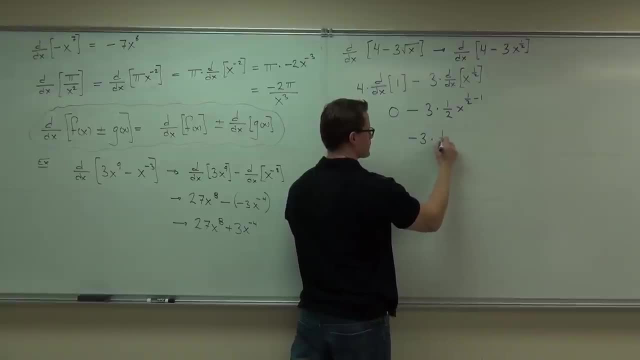 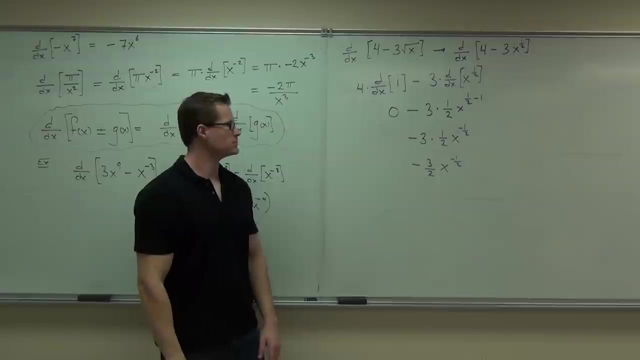 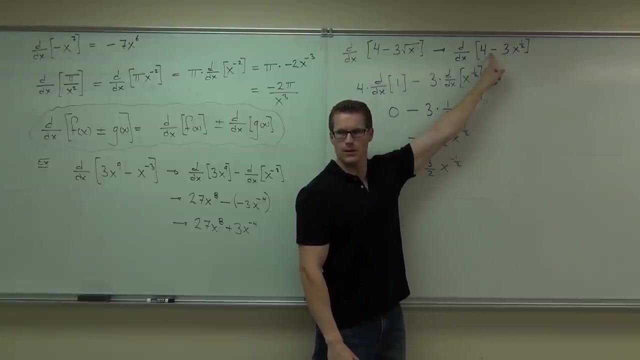 So our derivative is negative three-halves, x to the negative one-half. okay, Could you maybe get that directly from here? Could you get that? What happens to the four Zero? because it's being it's four minus something with a variable, so that's a constant term. 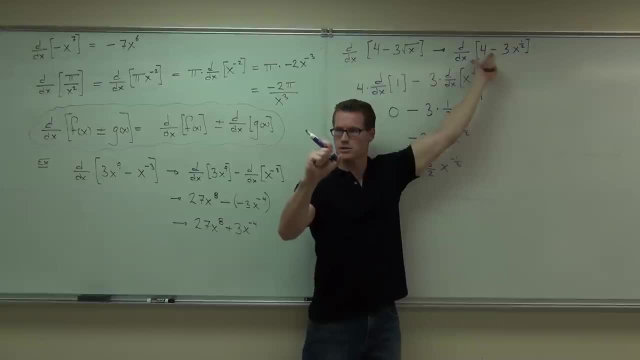 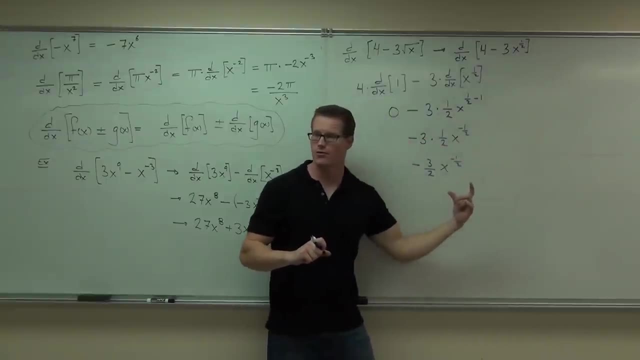 all by itself. The derivative of a constant term all by itself is zero. yes, Minus. oh, that's our negative one-half times three is three-halves. x to the one-half minus one is negative one-half. Can you make it a little prettier? 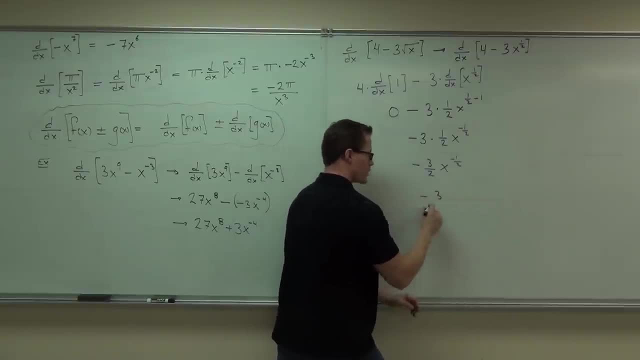 If you make it a little prettier, here's how it would look. The negative three would be on your numerator. Your denominator would have a two from that. This negative exponent would go down to the denominator and it's also a square root. 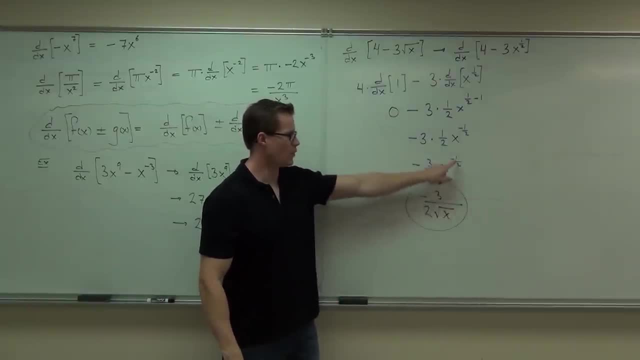 That's how that thing would look. Negative exponent: bottom One-half square root. Show of hands. how many of you feel okay with what we talked about so far? You can do this with any polynomial, Anything with an integer in it, or- and now we're moving on to fractional exponents. 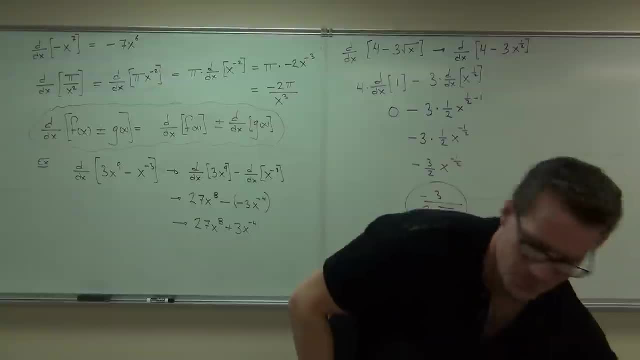 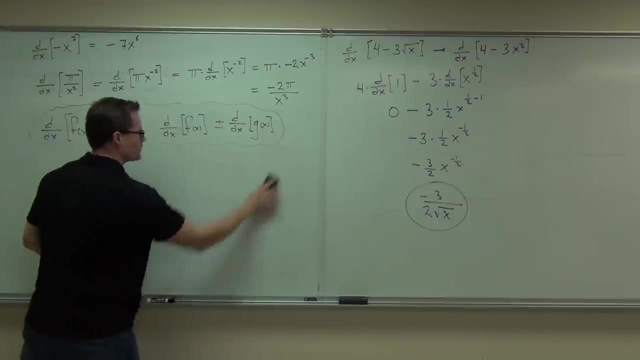 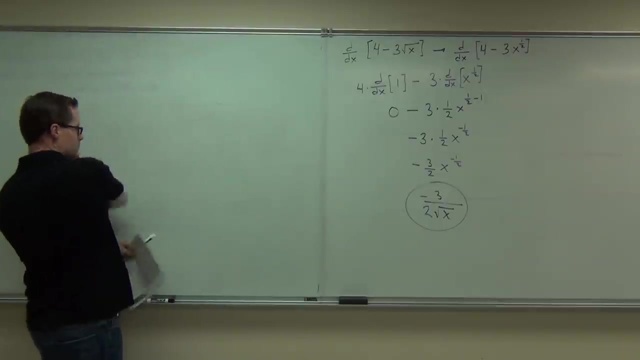 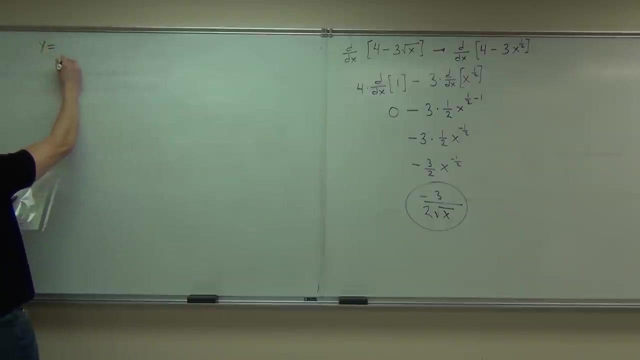 You can do this with pretty much darn near anything that's broken up into terms. So that means, when you get a problem that looks like this: Okay, Okay, Okay, Okay, Okay. And I say: okay, Five x to the seventh minus three x to the fourth, two x cubed plus x minus one. 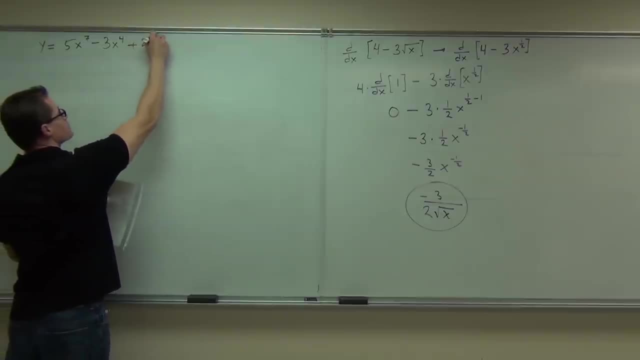 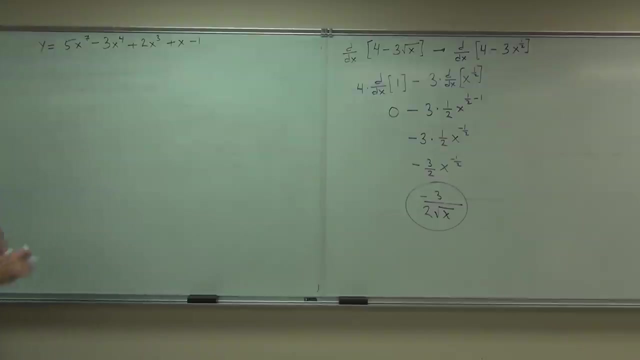 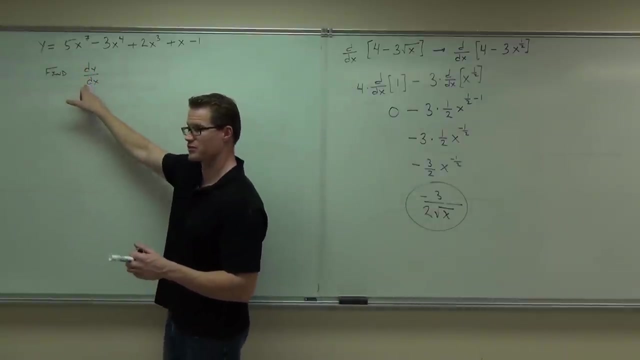 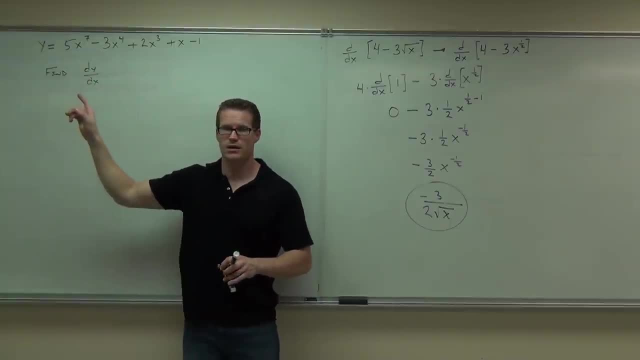 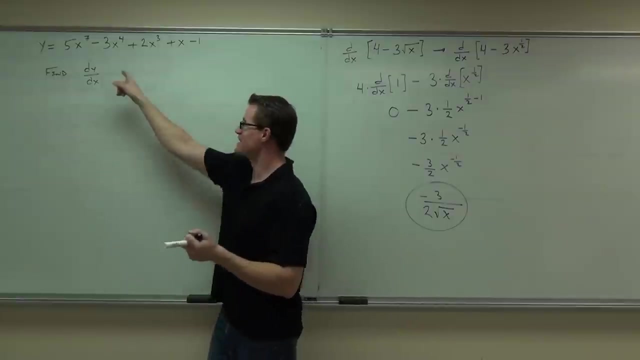 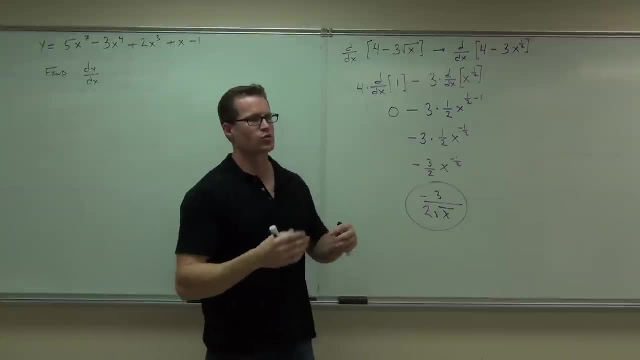 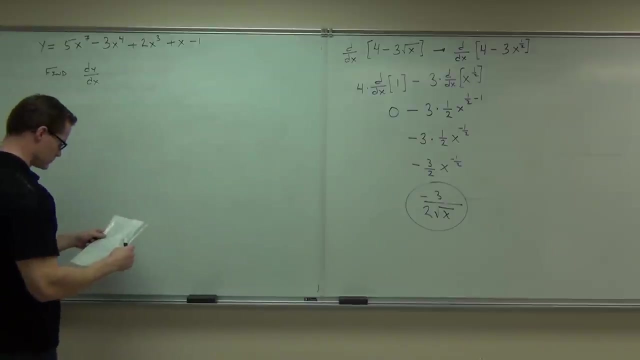 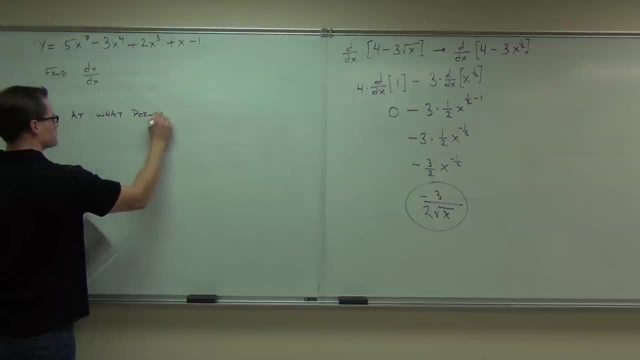 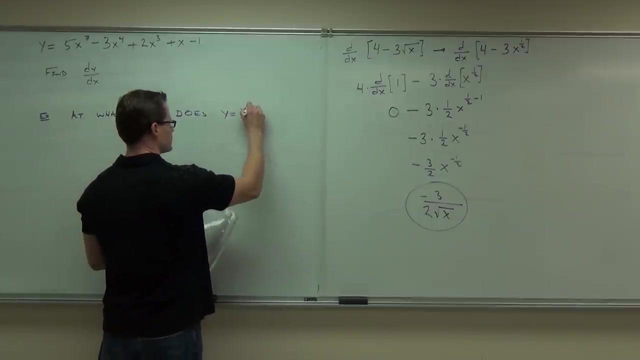 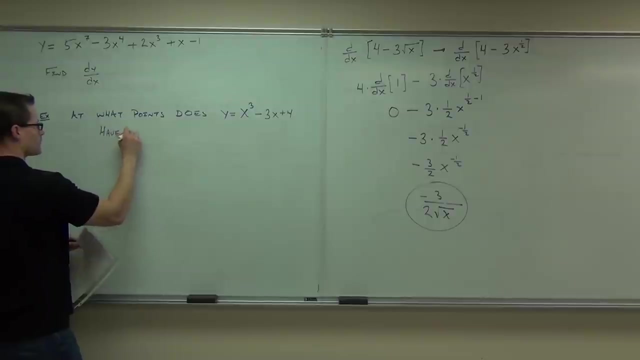 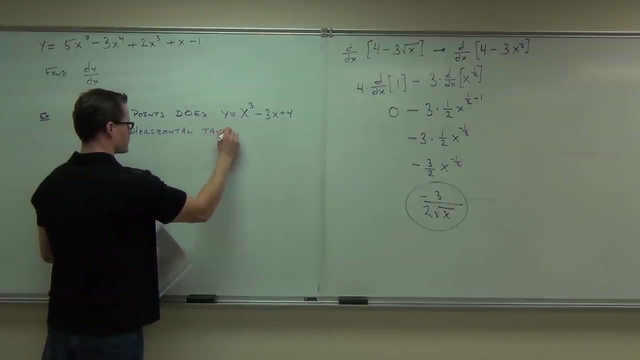 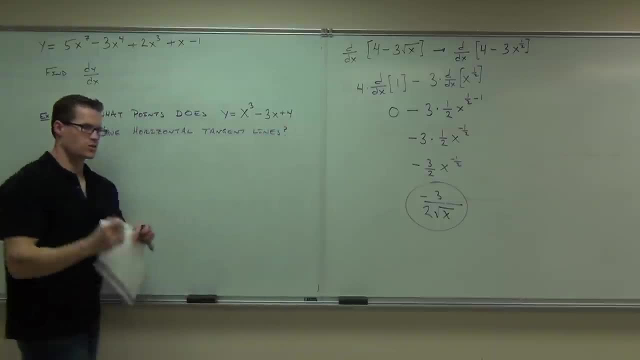 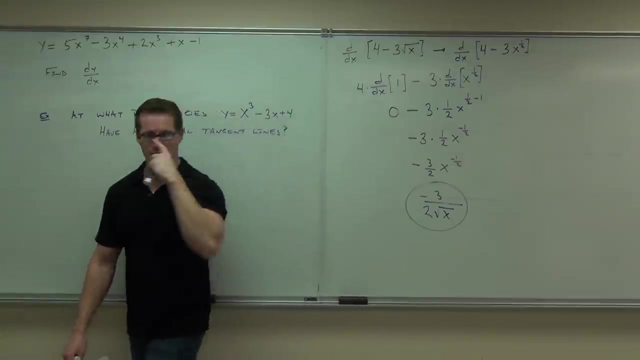 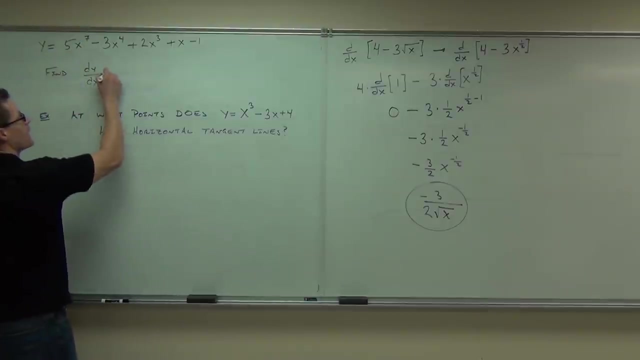 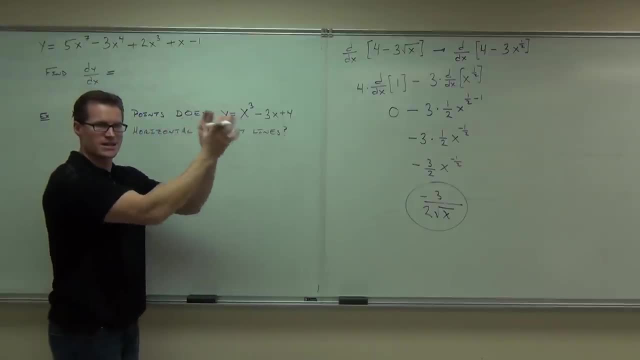 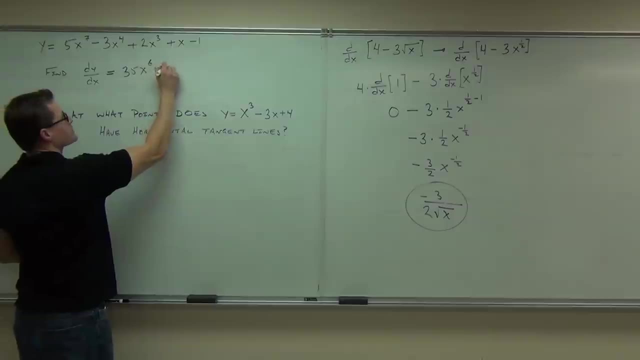 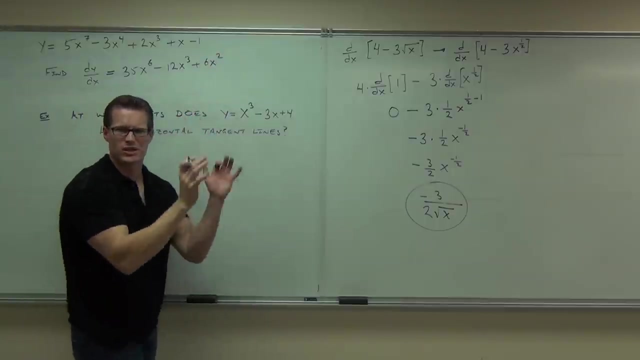 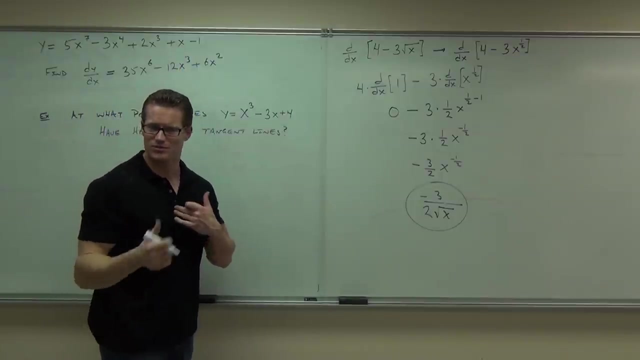 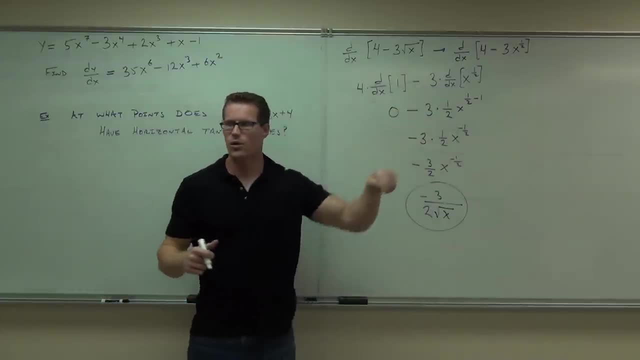 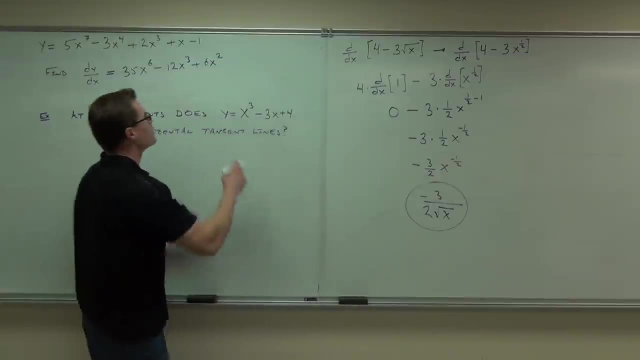 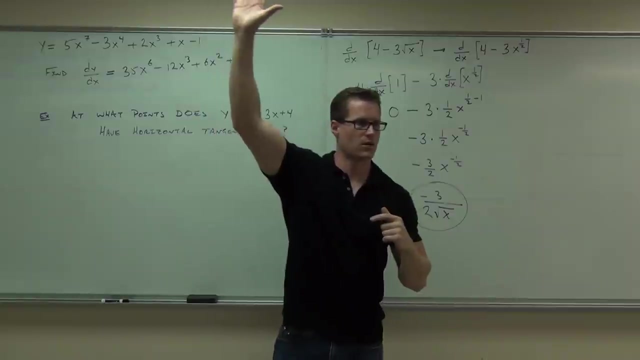 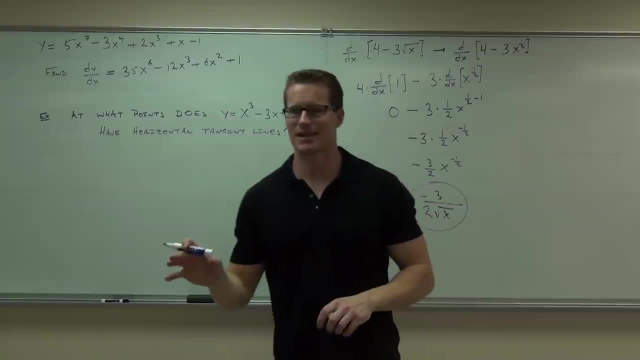 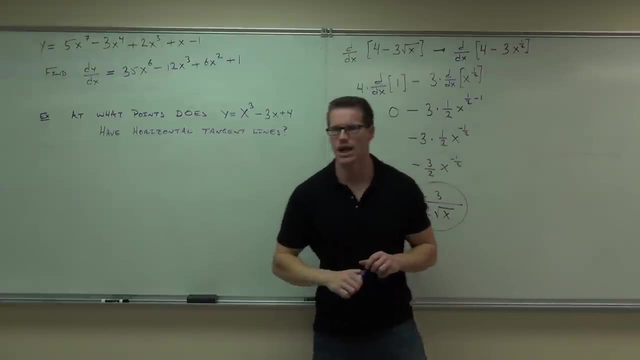 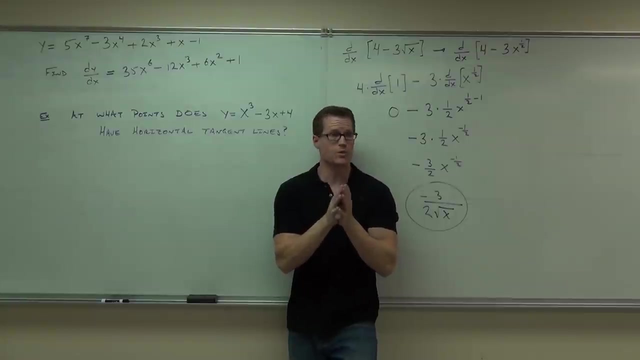 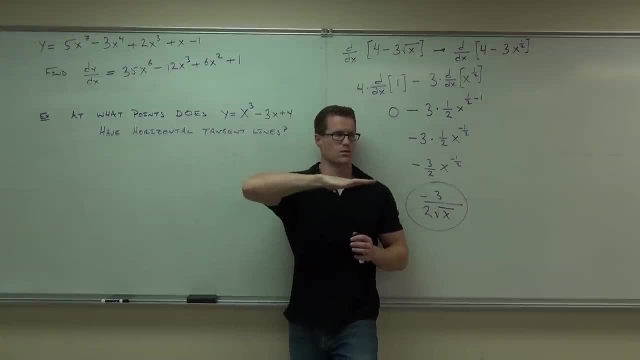 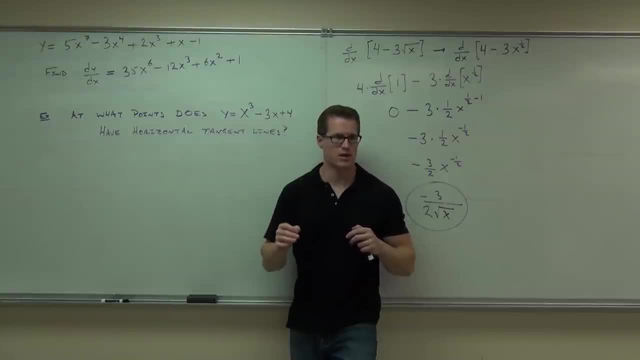 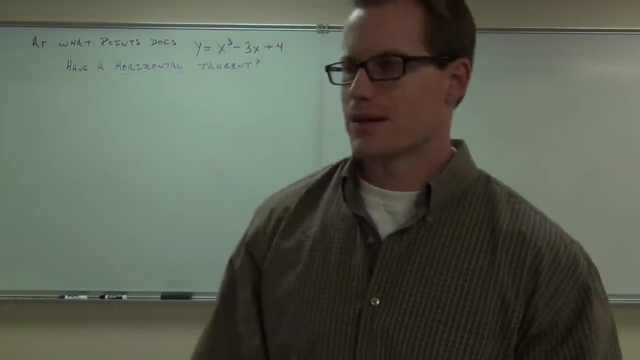 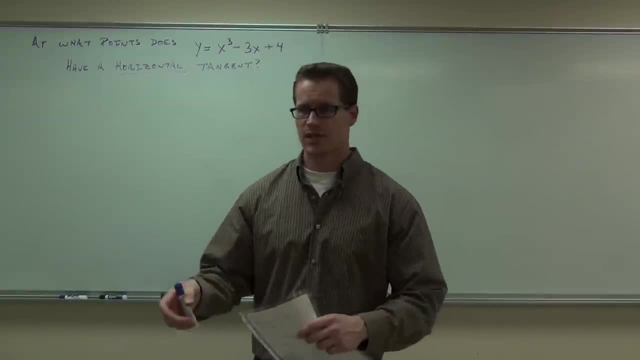 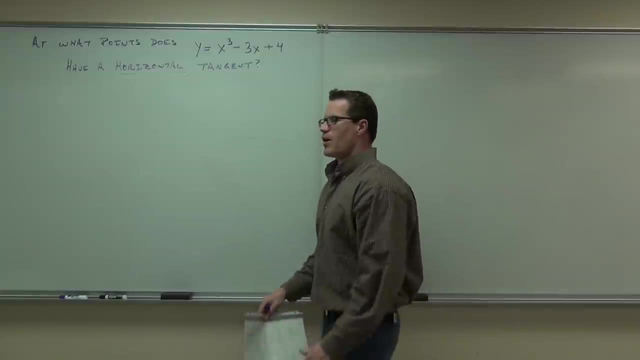 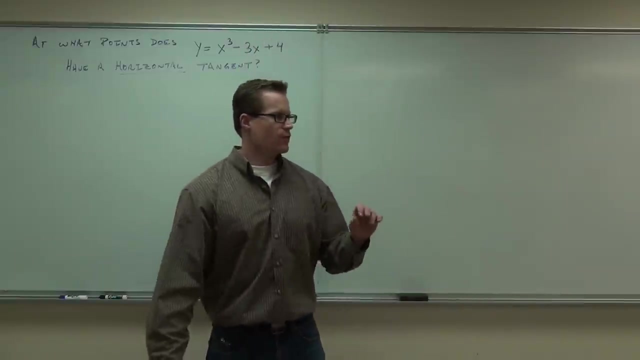 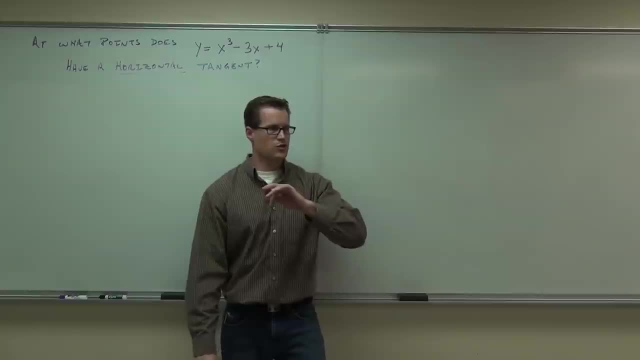 Okay, Thank you. Let's find out where functions will have horizontal tangent lines. Firstly, what do you know about a line that is horizontal? something about its slope, Zero or zero Slope would be zero for a horizontal line. So if we were trying to look for lines that are horizontal to our original function, 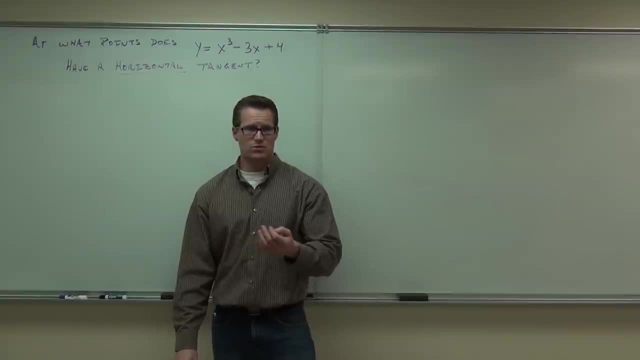 how do you find the slope of the original function? Take the derivative. A derivative would give you slope. So if we found the derivative of our original function and we found out where that was equal to a slope of zero, then we're going to be able to find the points where we have. 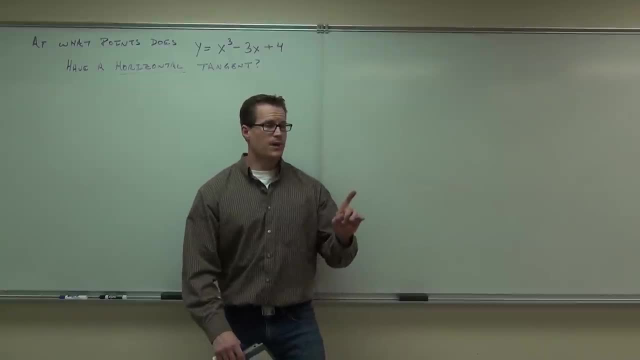 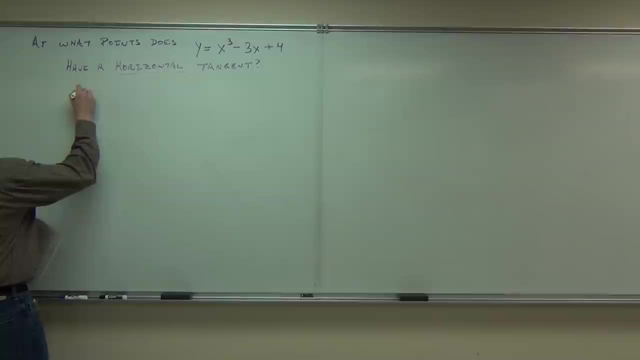 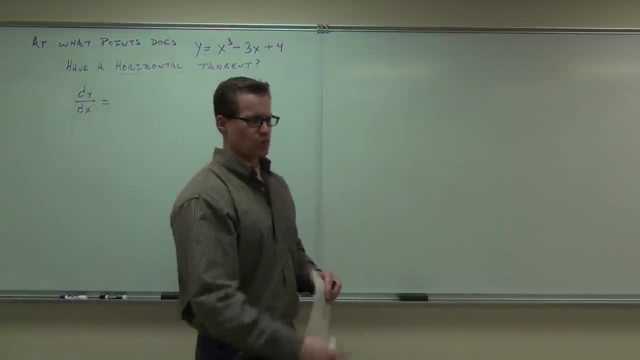 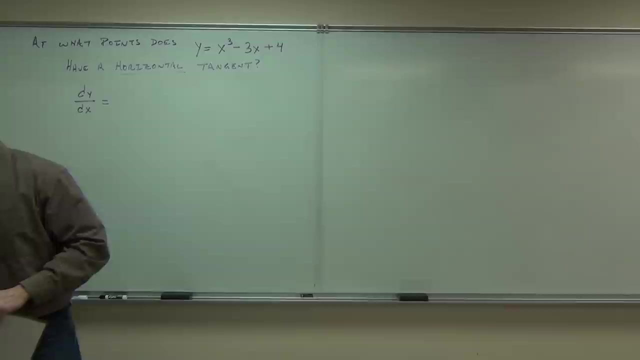 a horizontal tangent line. Here's how you would do that. Number one: take your derivative of your function. Go ahead and do that now. So do dy, dx or y prime. if you'd like Take your derivative, Come on. we got this Last time. take your derivative Derivatives now. 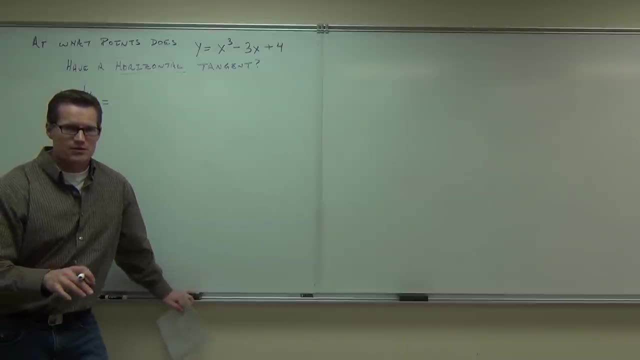 should be. oh man, this should be really quick Shoot. if we had to do the limit for this derivative, that would take forever. right, It wouldn't be that great, But now we can do it in literally five seconds. Like literally five seconds- crazy. What's the derivative? 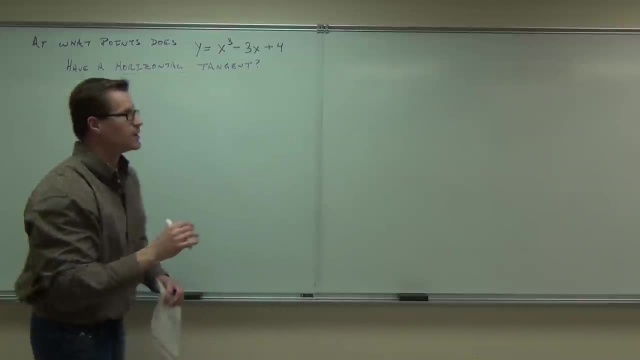 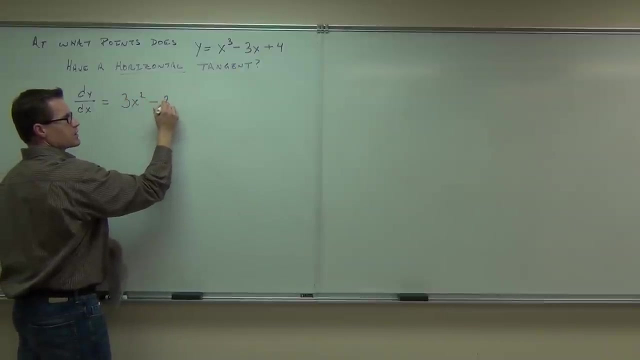 for y equals x cubed minus 3x plus 4? What is that Great, because I told you you can take it term by term. 3x squared, absolutely minus, how much 3x, 3x. What happens to the 4?? That's a constant. Derivatives of constants gives you zero if 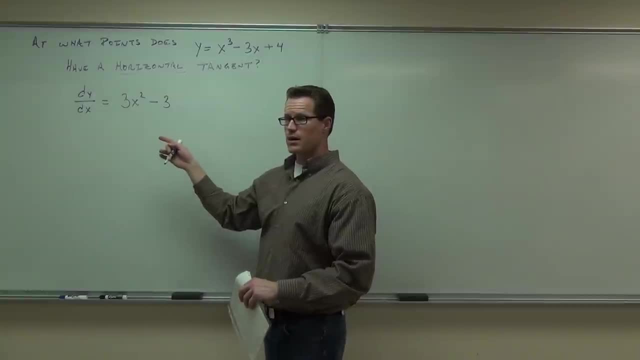 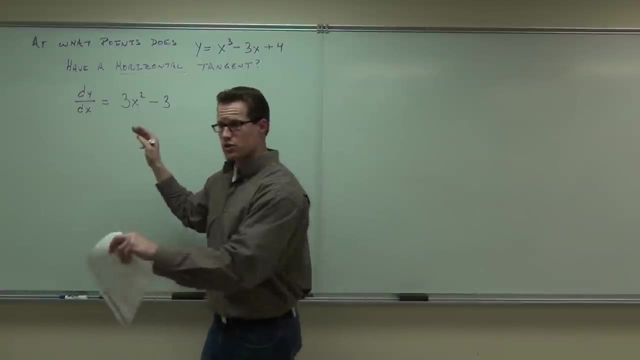 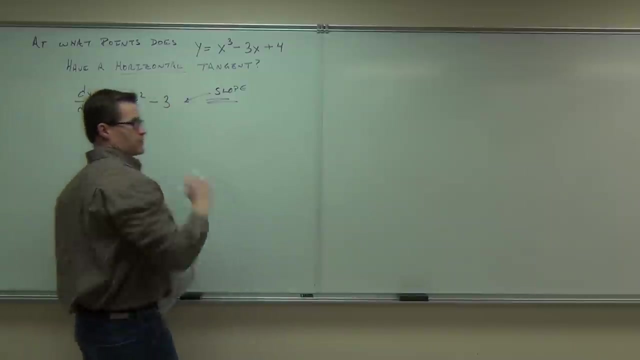 it's not attached to a variable. Did you get 3x squared minus 3? Okay, What does this give you? again, Formula for slope. So this right here is your slope of that curve. That's the slope of that curve, What I want. 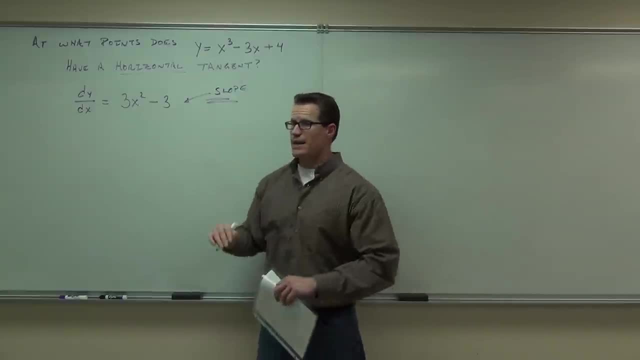 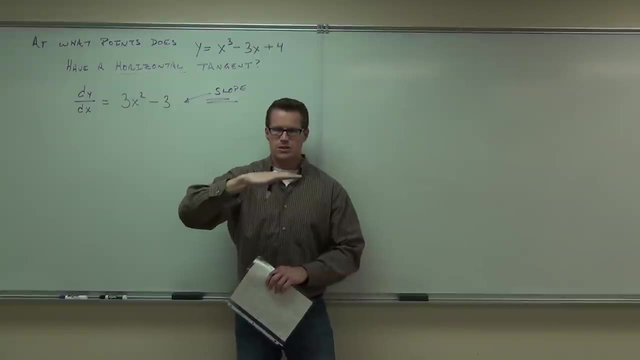 to know is where this curve has tangent lines which are horizontal. What we found out earlier is that the slope of the tangent line is the slope of the curve at the point. Does that make sense? So, if this is the slope of the curve at any point, 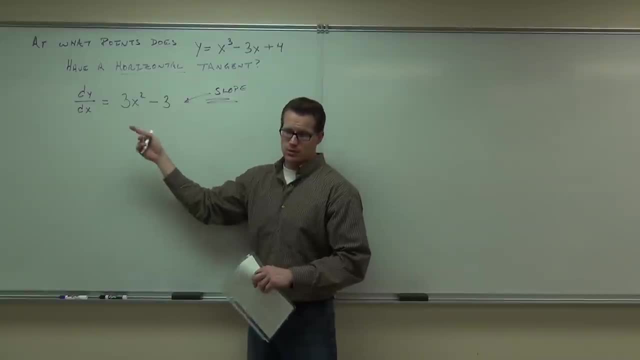 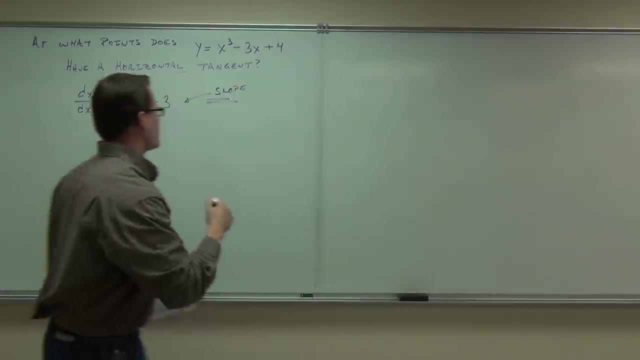 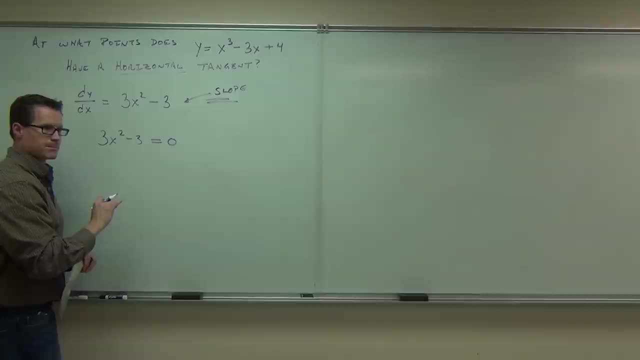 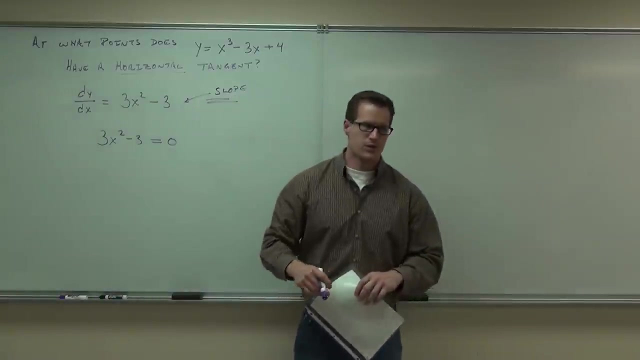 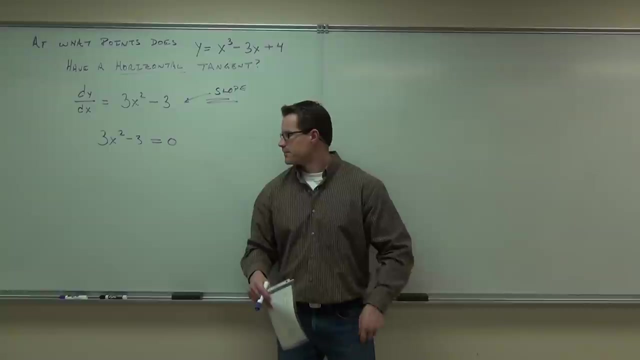 Zero means horizontal. Can you do that for any slope you were looking for? Say you wanted a slope where it equals two? Absolutely. So if I want a slope of one, I'd have it equal to one. Probably be harder to solve in this particular case, but you could do it. Yeah, this is a formula for slope. 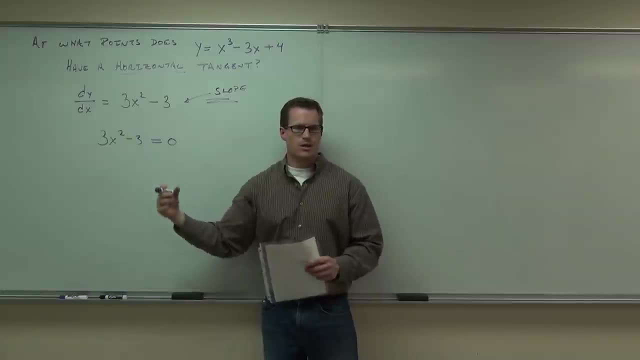 So if we set it equal to whatever we want now, the idea is we're typically going to pick horizontal, because interesting things happen when you have a slope equal to zero. That really does happen. It does happen to some things, For instance this At this point up at the top: notice: 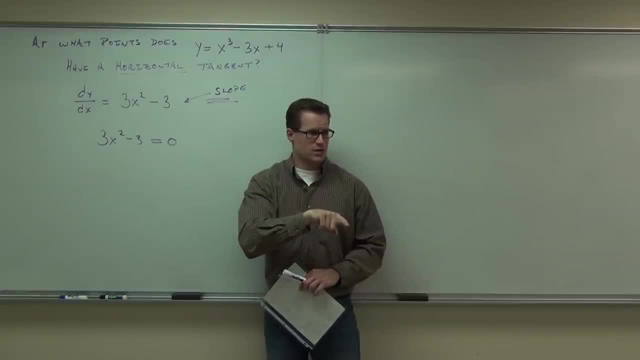 positive slope- positive slope- positive slope. negative slope- negative slope- negative slope. Do you see that? Therefore, at the top it has to have a slope of zero. That would be a change from increase to decrease and that would give you a relative maximum sometimes. 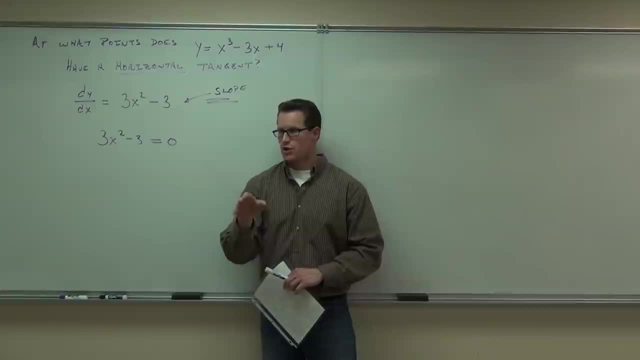 an absolute maximum of your function. So interesting things happen there. Curves are optimized normally when you have some sort of a slope equal to zero. So this is going to be the most common question I'm going to ask of you as far as we're going. 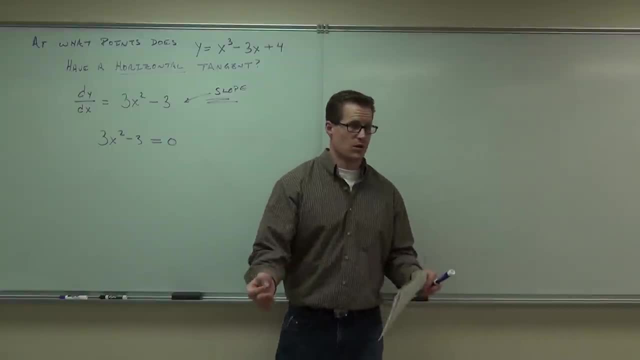 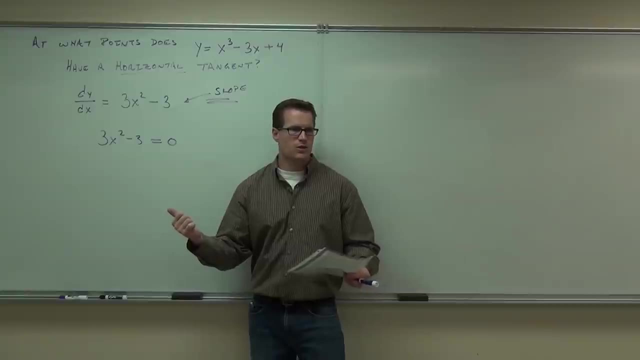 to relate the slope to some number. It's typically going to be zero. Do you follow the idea? Now, can you solve that? Hey, that's just some basic algebra. So if we solved it, how might you solve it? You could, You could do factor three: difference of squares. you're going to get one and negative. 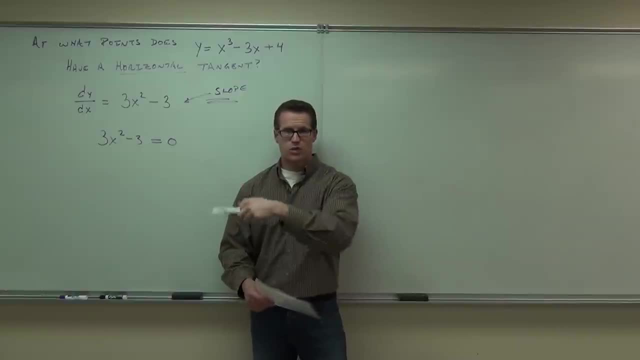 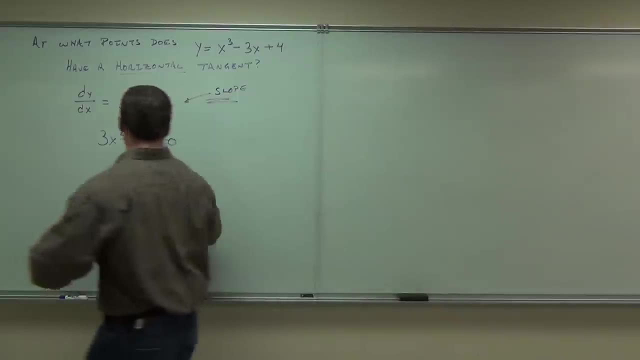 one. Do you see it? Or if you added three divided by three and took a square root, you'd still have one and negative one. Do you see it? either way? So, either way, because when you take a square root, you have plus and minus. 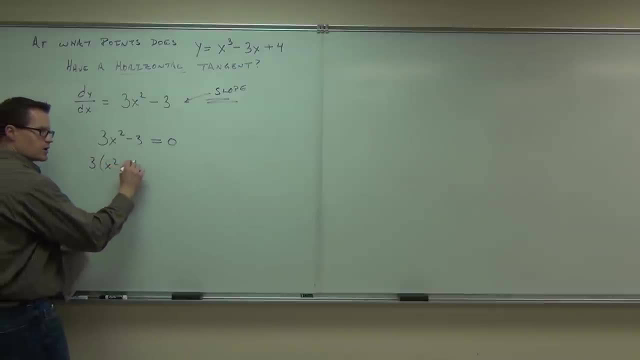 I like the factoring, The factoring version. Sure, we get: x squared minus one equals zero. That's three X plus one, x minus one, X plus one equals zero, X minus one equals zero. Therefore, x equals negative one, X equals positive one. Hey, do something for me real quick, Just verify. 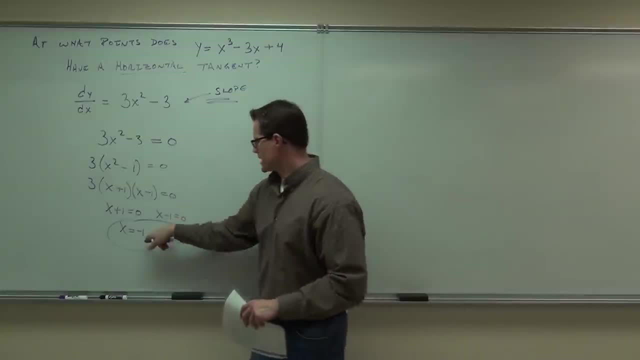 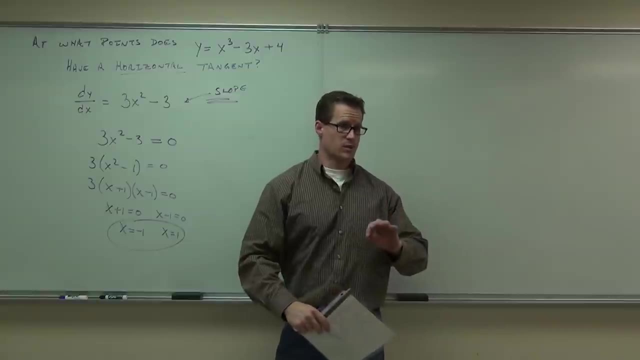 this for your own edification here, for your own knowledge. Take those, plug it into the torment stories. These are the points on the tangent. Take those and plug it into that. Take these and plug it into that and see what you get. okay, Just so you can see what happens. 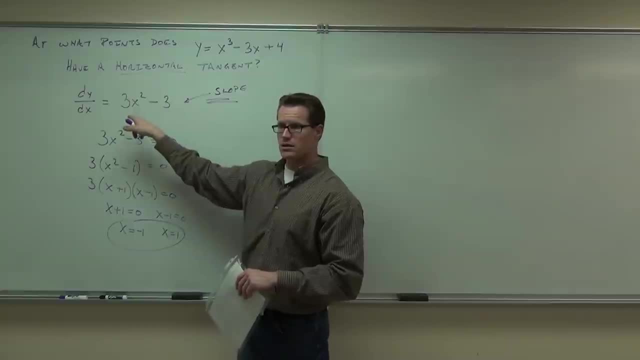 here. Take negative one and plug it in. How much do you get? You get zero. Take one and plug it in. how much do you get? So would you agree that these are the points where your slope is going to equal zero? These 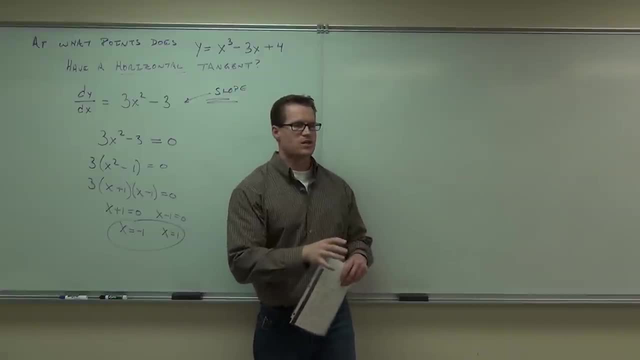 are the points where you're going to have a horizontal tangent. These are actually not the points I misspoke. These are the x values. Can you now find the points at which you will have a horizontal tangent, The points? These are your x values. How do you find points? 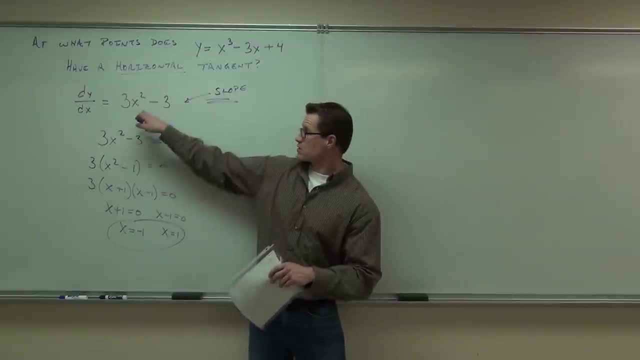 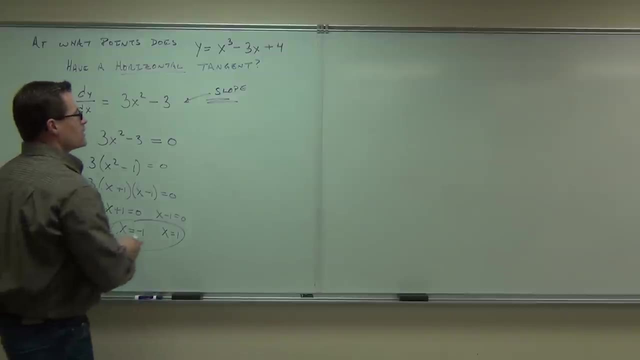 how do you find points to this one? no, that gives you slopes. that would give you points, so the points would be at all right. well, let's see if x equals negative 1 and x equals 1, if I plug in negative 1 and I plug in 1, these two. 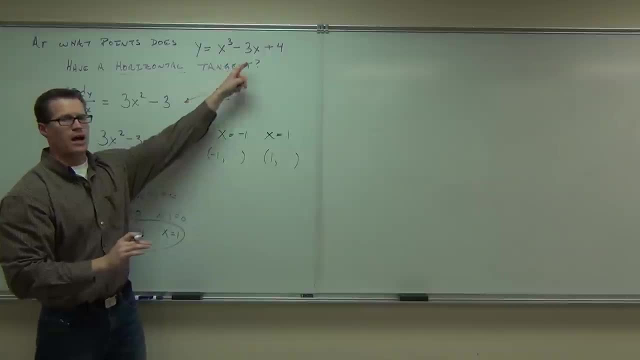 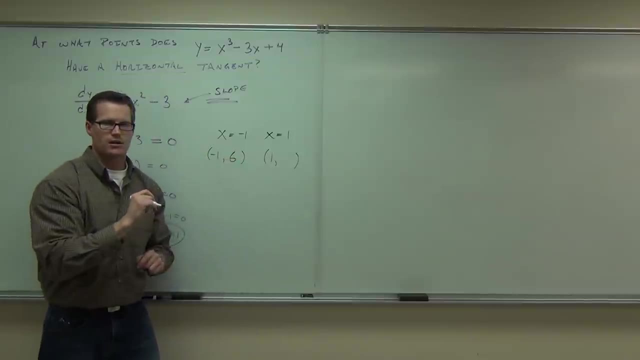 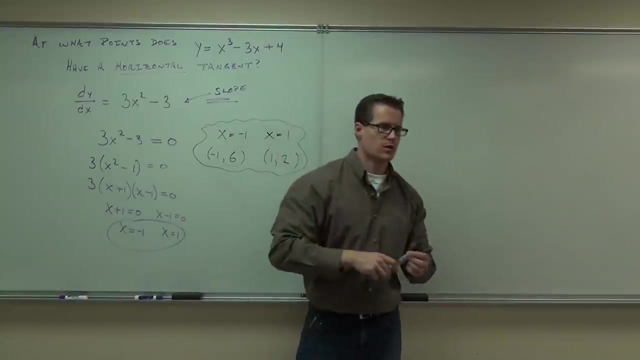 points will have horizontal tangent lines. plug in negative: 1. how much do you get out of that? six, okay, plug in positive: 1. how much do you get out of that? those right, there are the two points where you will have horizontal tangent lines. nowhere else, that's it. I can say for certain. nowhere else, because we have 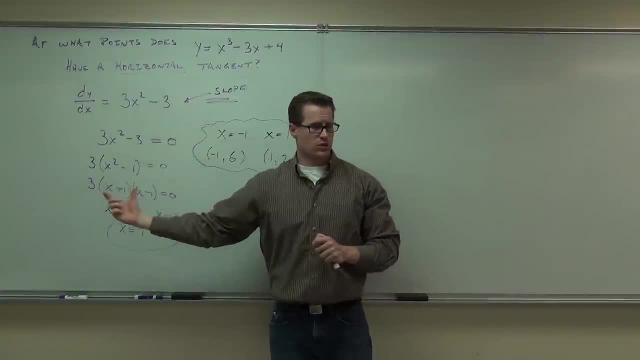 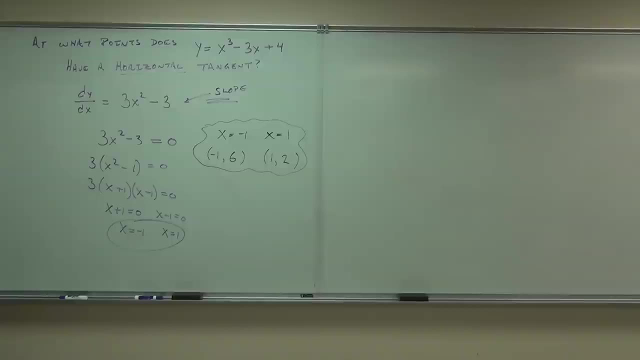 found the function for the slope, if you said equal to zero, and we solved it. these are the only two points that existed, that's it. how many people understood the idea of a horizontal tangent? it's kind of interesting, right, right. the last thing in our section really is: we can also talk about higher. 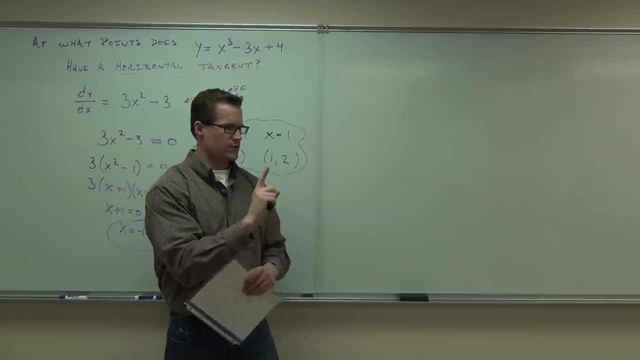 derivatives. we've been taking first derivatives this whole time, which means you take the derivative of the function and that's it. right now we're going to. I'm going to tell you that you can take a second derivative and the third derivative and as many as you want to take. so we're going to look at higher. 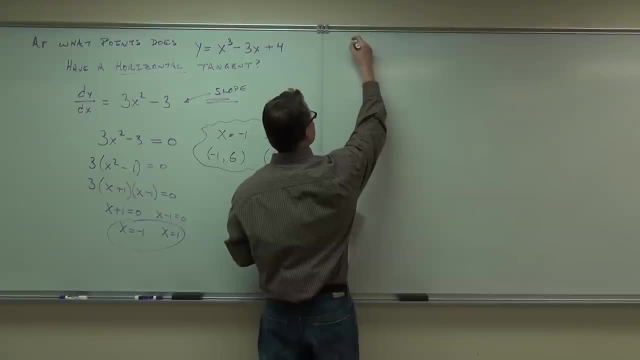 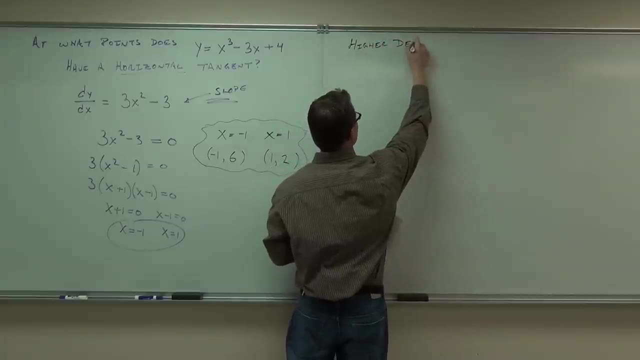 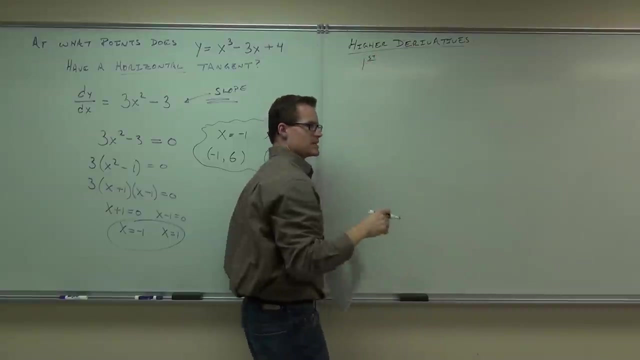 derivatives: first derivative, second derivative, third derivative, the fourth, the fifth, eighth, the ninth, ten and the running out of point that comes out from the underlying equations of constant Heavenly ahead. I do need to tell you the notation, though, how we say, how. 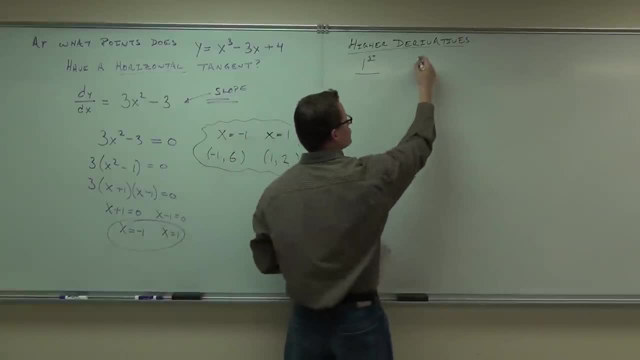 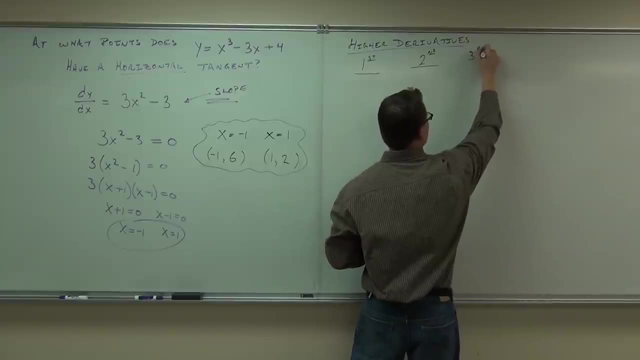 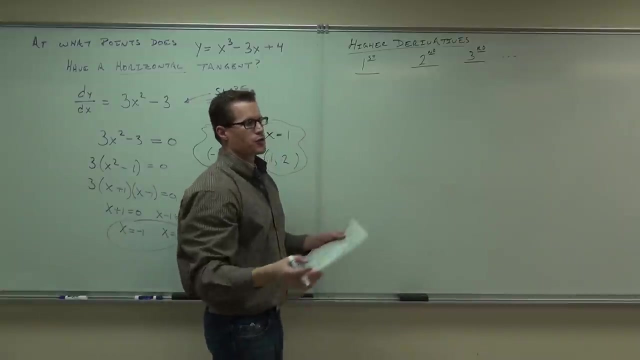 we write out our first and second, a third and fourth. so here's the first derivative. second derivative will talk about a third- FE4 billions- and we're going to, and you can go further and further, and further, however many derivatives you want to take. Our notation for a first derivative was typically this: 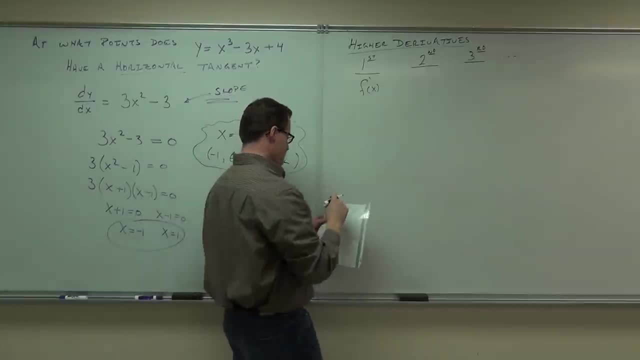 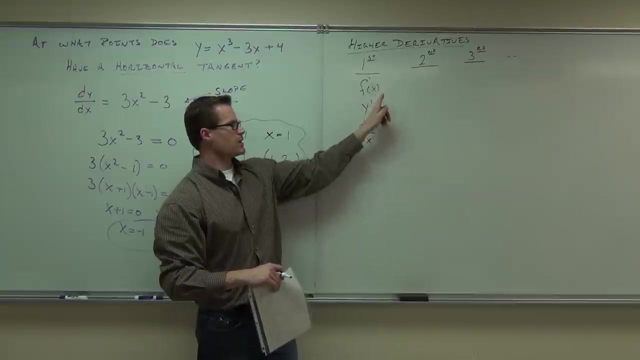 f, prime of x. you remember that one right. Or we'd have y prime. you can write y prime or dy dx. Those are the main three. We stick with those normally. Actually in this class we'll be sticking with this one. 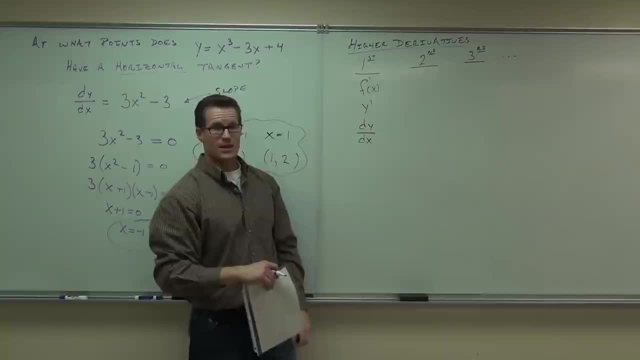 and that one typically is where we like to go. You all right with that. so far. That should be like old school stuff- Well, not old school, It's all new for you- but like from the previous section. So we have that. 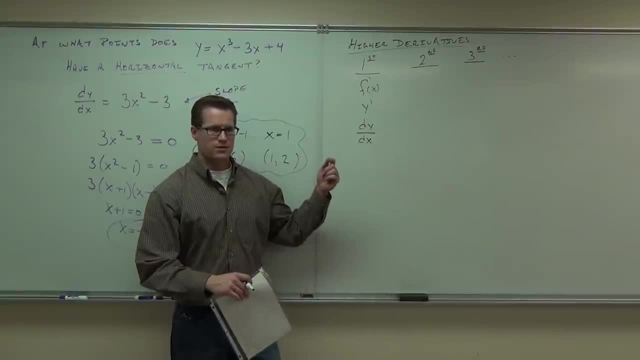 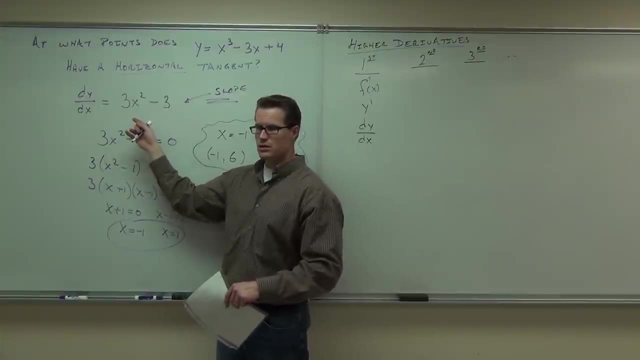 Second derivatives say this: You take your first derivative, then you take a derivative of that. So, for instance, could you take a derivative of this? Yeah, it'd be pretty easy. You'd get how much? 6x, 6x, very good. 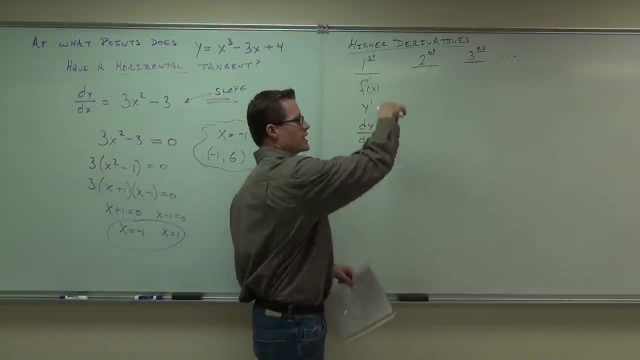 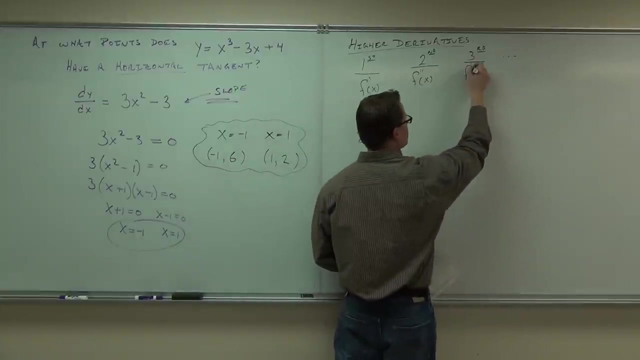 That would be called a second derivative. Second derivatives are notated this way. So this is the f prime of x. You'd say f double prime of x. If I took another derivative, I'd have f triple prime of x. And you just keep on writing little dash marks. 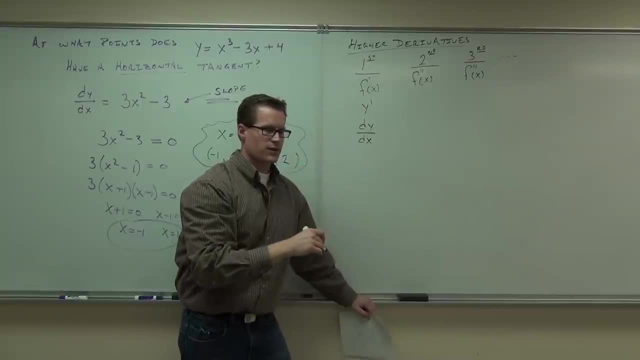 Some people I've seen put a little 4 up there for fourth derivative, although we rarely get to a fourth derivative. but you could. But you keep on writing those little dash marks. This is called the Newtonian method of writing derivatives. See, there's these two guys: Isaac Newton and Godfrey Leibniz. 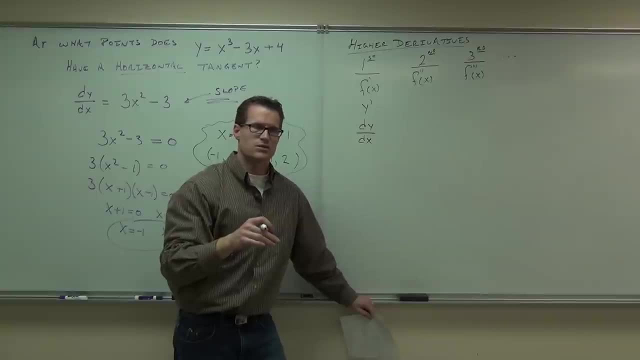 who invented calculus about the same time. One of them was English. I think Newton was English, wasn't he? And then Leibniz was German. And of course, back then the nations want to say: well, we invented calculus. 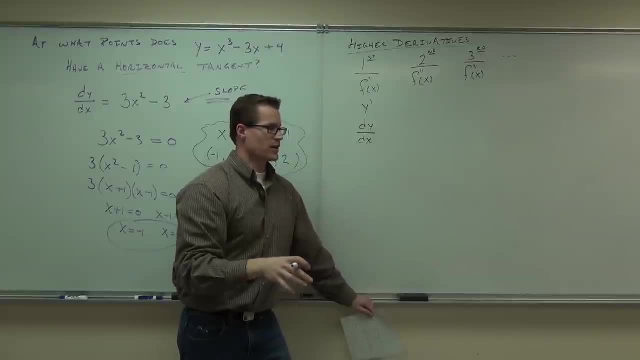 This is ours, And so they kind of stuck with their own notation. And this right here is Newton's way of doing it. He used little dots, And this is the Leibniz way of doing it, And we still have the notation to this day. 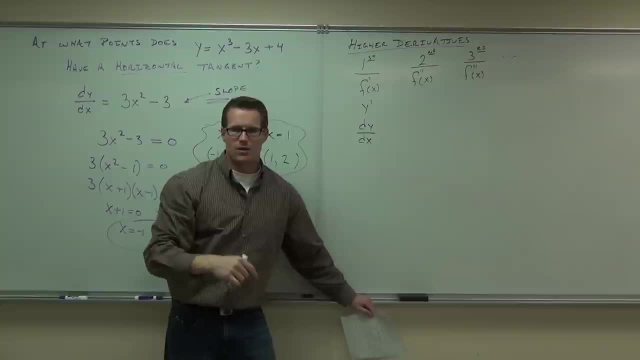 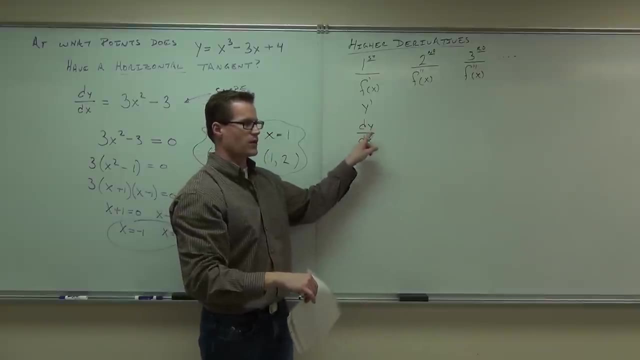 So this comes from the German guy and this comes from the English guy, how they notated it, And we still use that, And each of them have their advantages. This one. I'll show you some advantages to this later on, why it's kind of nice, why I do it this way. 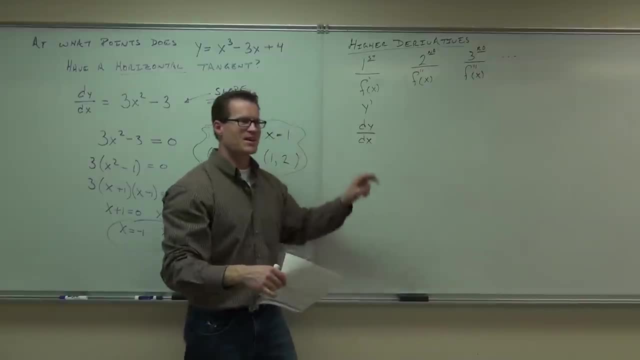 First because of my German heritage, you know, But then- no, I'm just kidding- Because we actually can do some pretty cool things with this type of notation. I'll show you that, especially when we get to like differential equations, things like that. 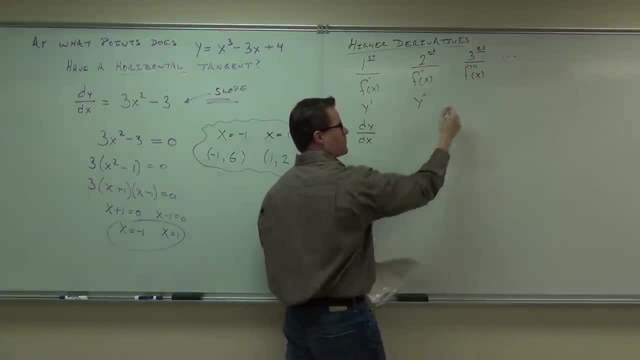 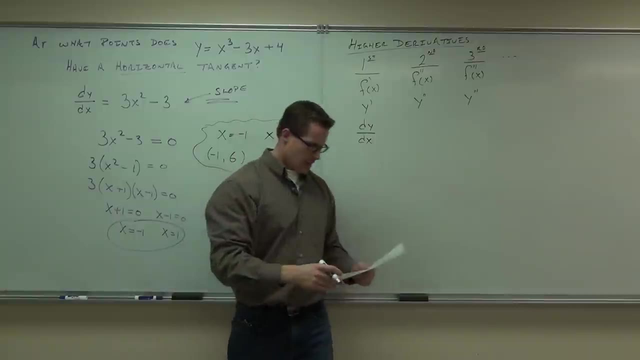 All right, Now y prime. you'd still stick with the y double prime, Y triple prime, and so on. The dy dx does this a little bit different. It says: okay, this is a first derivative of y with respect to x. 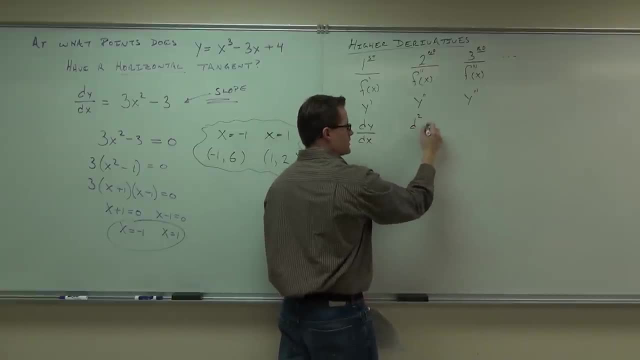 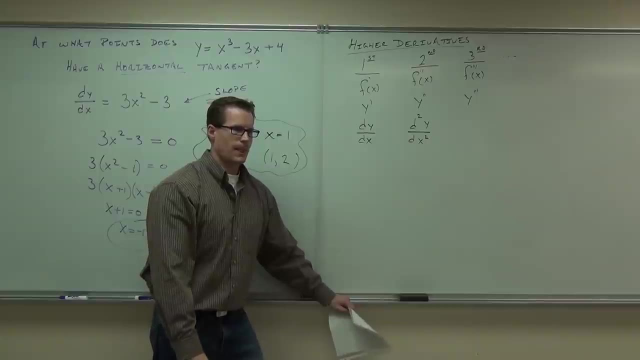 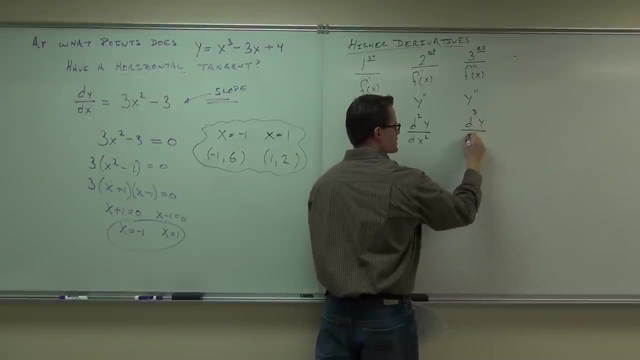 Okay, One time This says: take a second derivative of y with respect to x. both times That's how I think of it. So you have a little 2 saying that's the second derivative. This is a third derivative with respect to x. 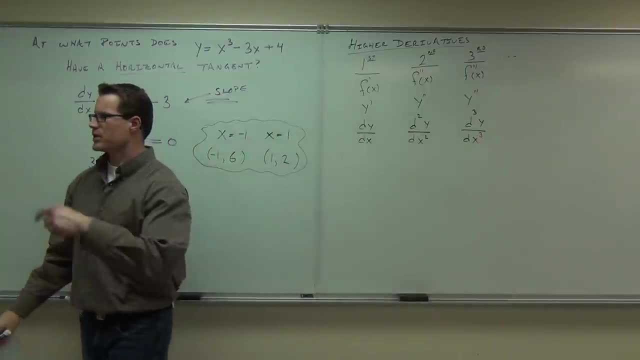 Every time. So we keep on putting on another number. That's a little bit more concise than those little dash marks. I like that a little bit better. It looks better, You can see it more. Also, if you're going through and you just, oh, lost one, 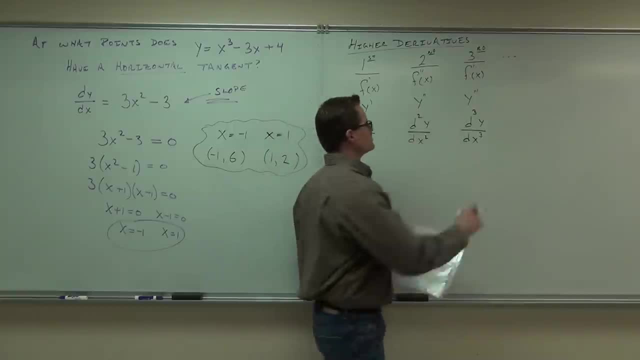 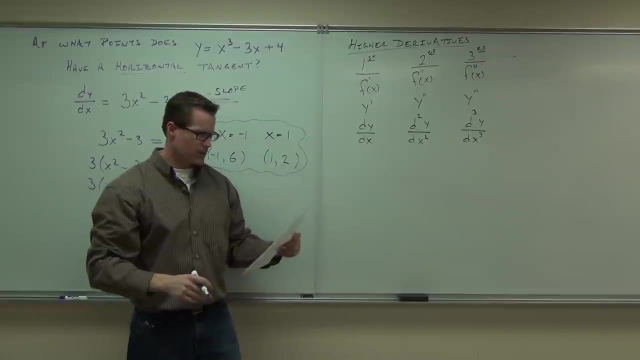 well, that would suck right, Because then you don't know. But it's hard to screw up a 2 and a 3.. Well, maybe not. Maybe not that hard, But harder than messing up a dash mark. Are you guys okay with the derivative notation? 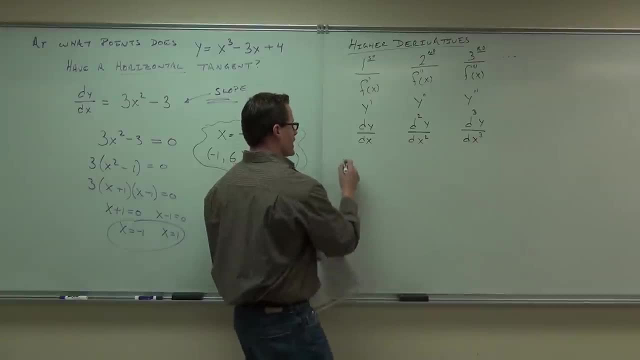 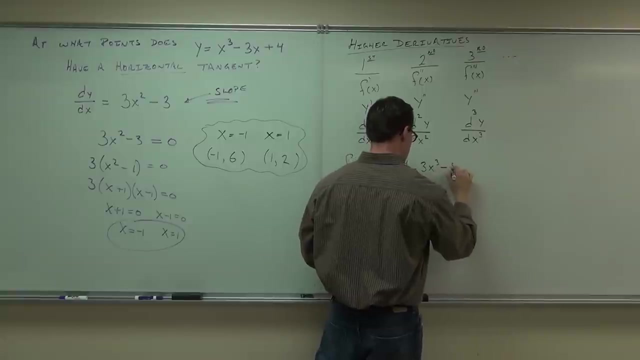 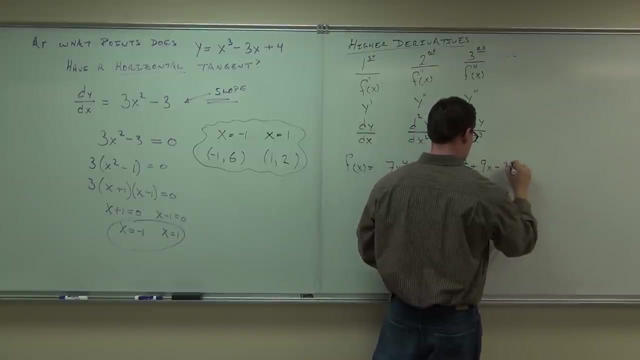 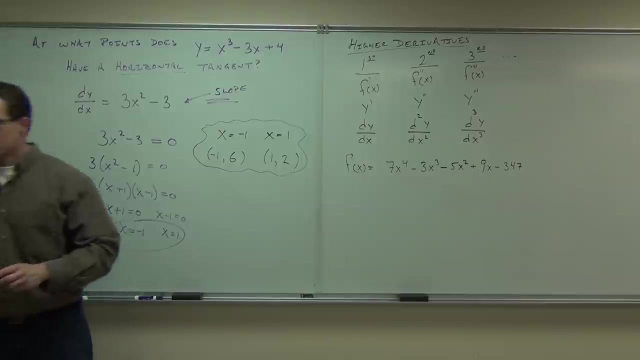 First, second, third, What I'd like to do now, just for for fun. can you find all of the higher derivatives of this? Can you find all the higher derivatives there? So start with the first derivative. Find the first derivative. 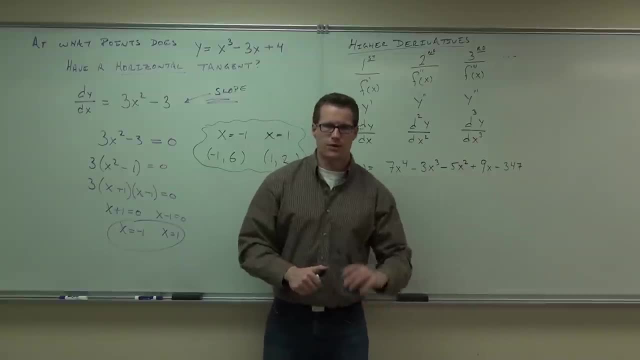 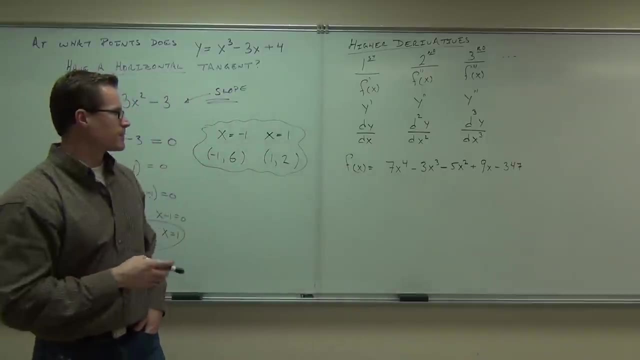 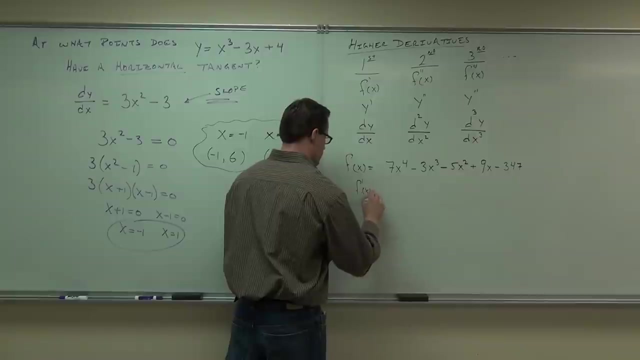 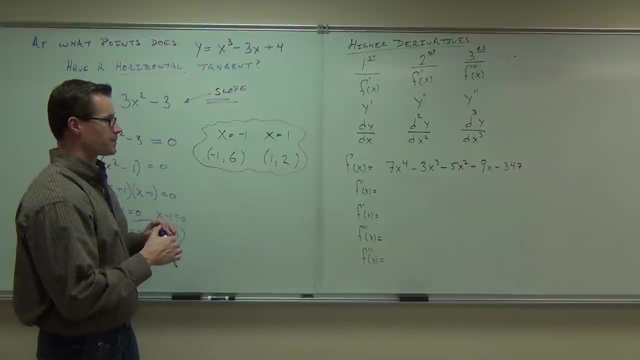 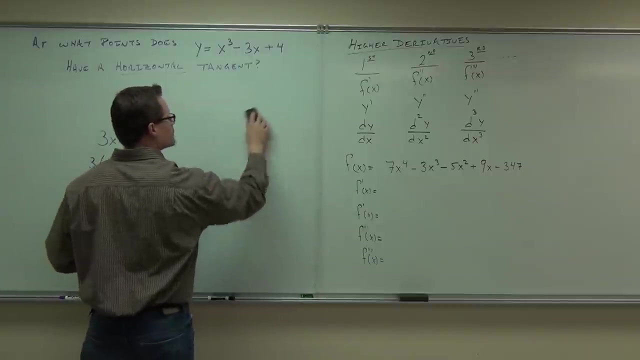 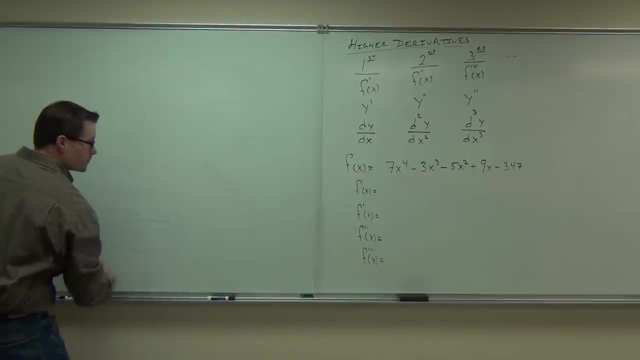 Then find the second one, Then the third one, Then the fourth one, Then the fifth one, Then the sixth one And see what happens. Okay, I want you to keep going. Did you find them? Did you find them? Did you find them? 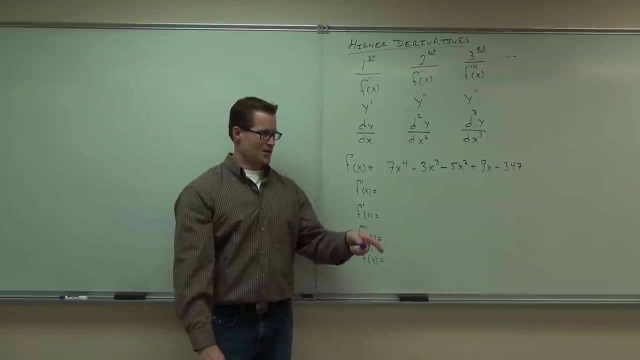 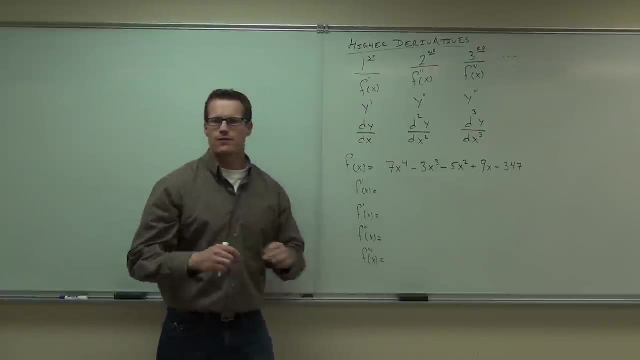 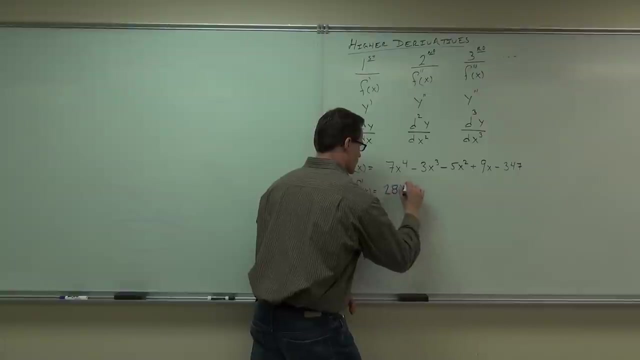 Are you still working on it? Are you still working on it? Keep going? If not, well, let's start up here. First derivative: can you please tell me what the first derivative is on this 20x cubed? You got that one right. 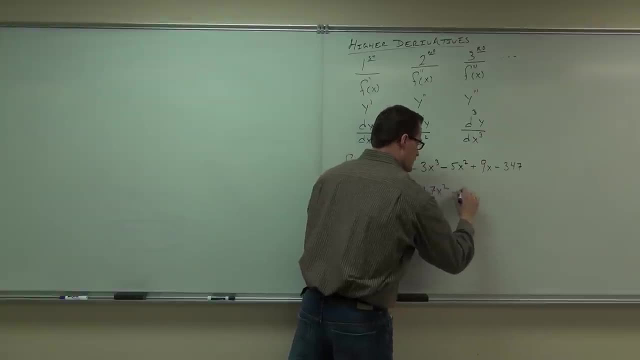 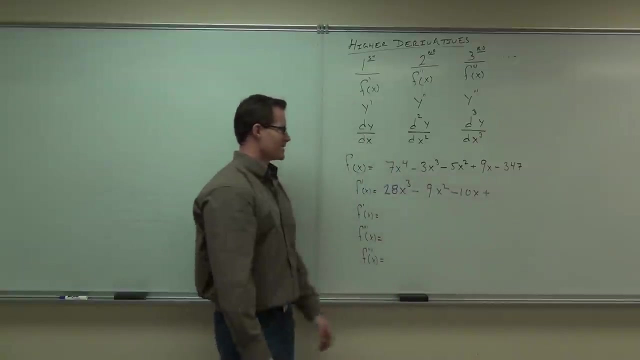 Okay, then I heard: 27x squared, yes, minus 10x, Minus 9x squared, Whatever, Oh, 27.. I actually cubed it, my bad. I was on this one Shoot. I guess three times three is nine. that's good to know. 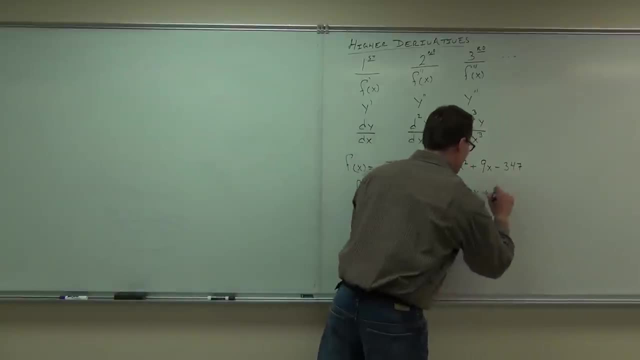 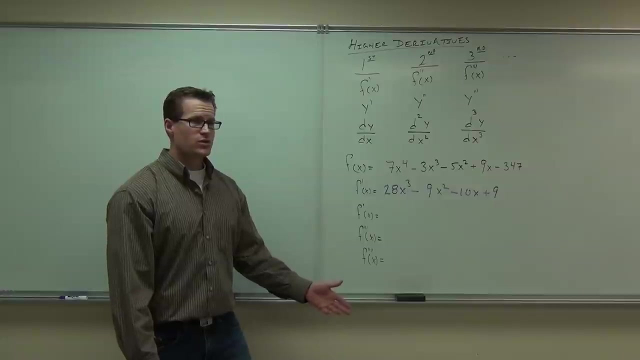 Yeah, and lastly, what else do we have Nine, Yeah, my bad. What happens with 3.47?? What Bye-bye. They need to go away. Here's what's interesting too. What if I did made this 34,755?? 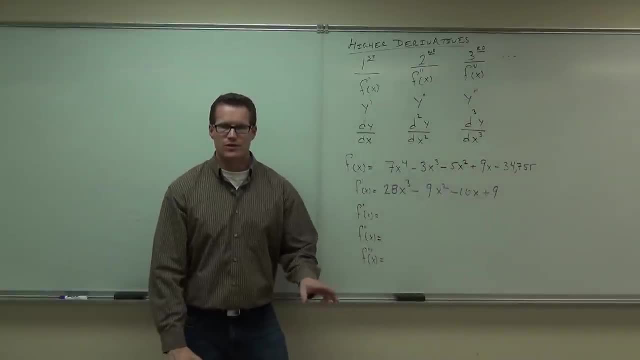 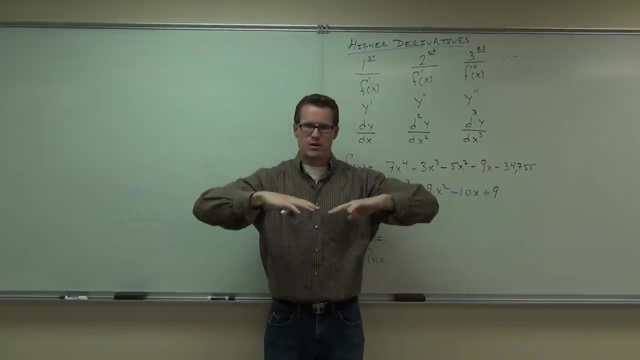 Would this derivative change, So that constant really has no effect on your derivative that we're talking about the slope right. So all this is is really a shift upward or downward. So if we're just shifting the whole function up or down, 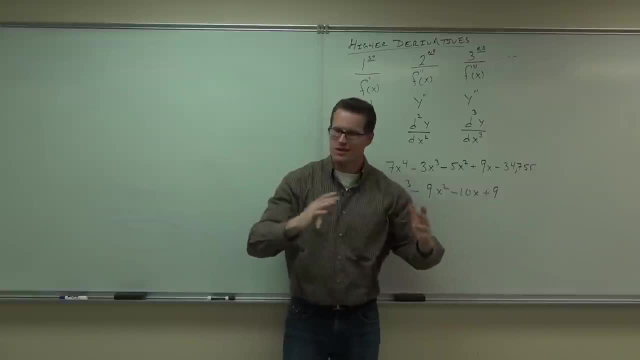 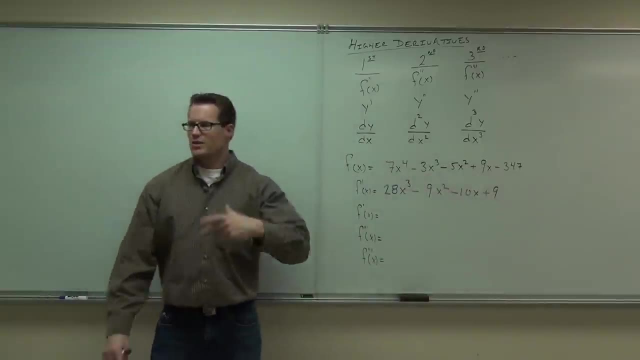 it doesn't affect the slope of the function. It says: oh, now it's way up here, now it's way down here, So that really doesn't affect it, which is interesting. Okay, next up, Second derivative: We just take the derivative again. 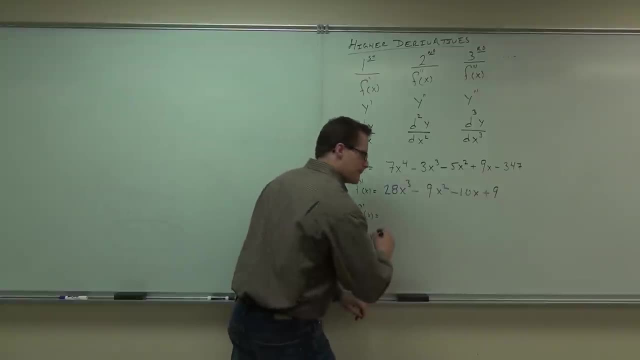 So we're going to do? what's 28 times three? What is that? X squared minus 18x, you got that one right minus 10x. What happens to the nine? It's a constant. It goes away. 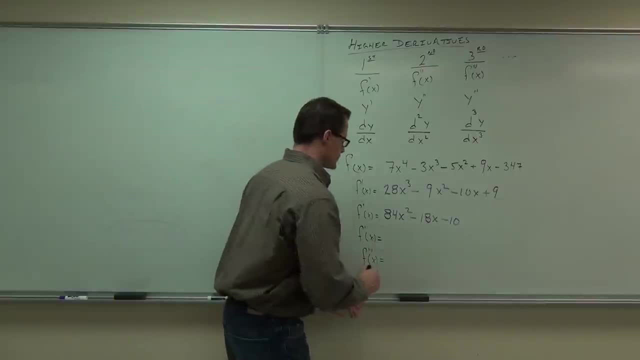 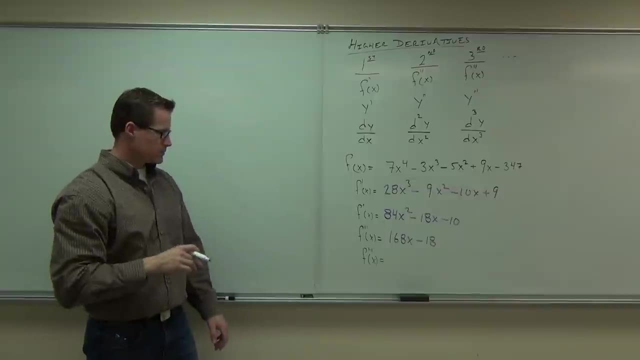 Now what? You can do it again with the fifth derivative: 168x minus 18x 168.. Okay, And then you get 168.. Then we take the derivative again and yeah, we're going to get 168,. 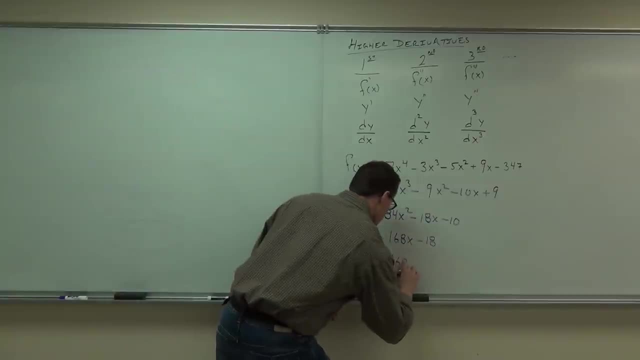 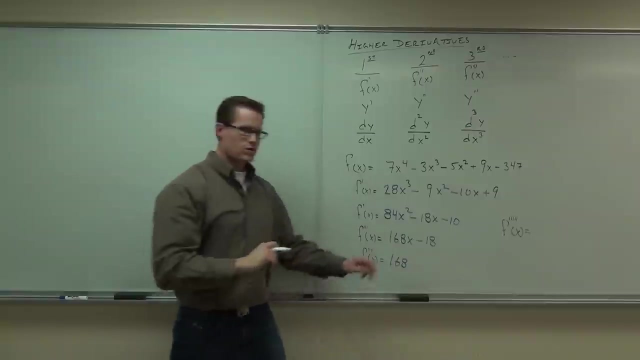 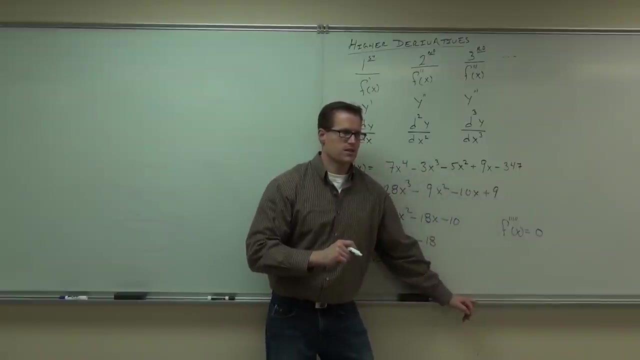 and again that constant goes away: 168.. And that's it. Well, let's do the fifth derivative Two. What's the fifth? what's the derivative of 168? Zero. What's the sixth derivative? Zero. What's the seventh derivative? 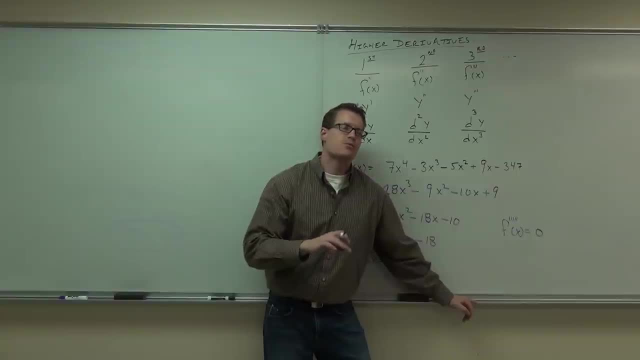 Zero. What's every derivative after that? Zero. This is going to happen for every polynomial. You see, at some point, no matter what you start with, if it's a polynomial, you'll be able to take a derivative, and what happens every time is the order of the polynomial. 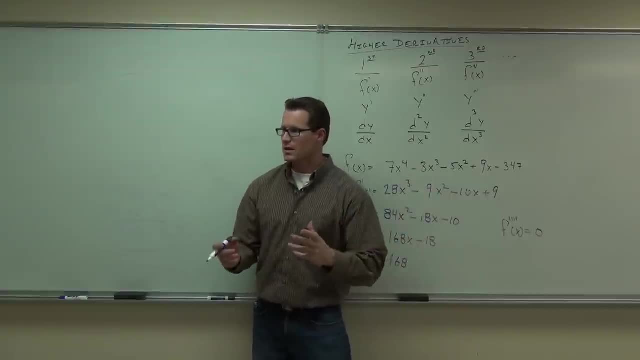 decreases by one. So four, three, two, one zero and then a constant. That's going to happen with polynomials. Now, does it happen all the time? No, All the time. All the time. Think about something that's not a polynomial. 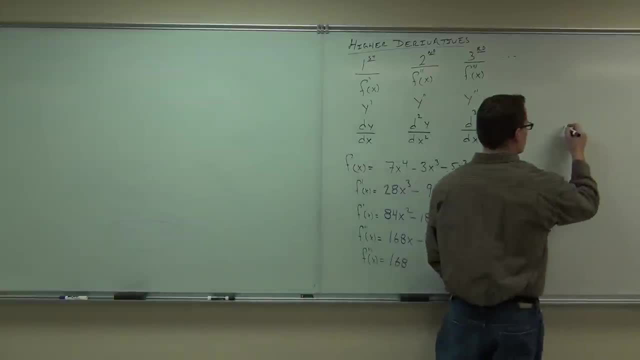 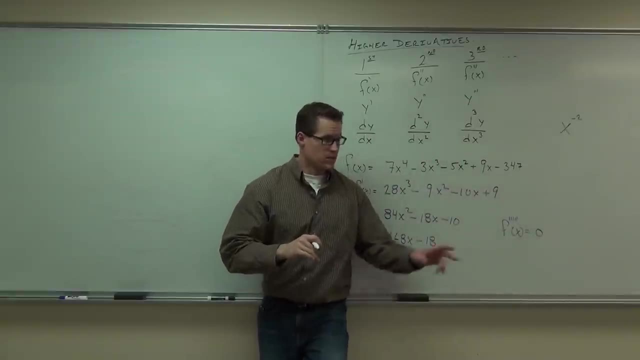 I'll give you an example, if you need one. How about that? Well, decreasing, because we subtract one, but it becomes more and more and more negative. right, This derivative would, the derivative of that would give you negative two x to the negative three, right. 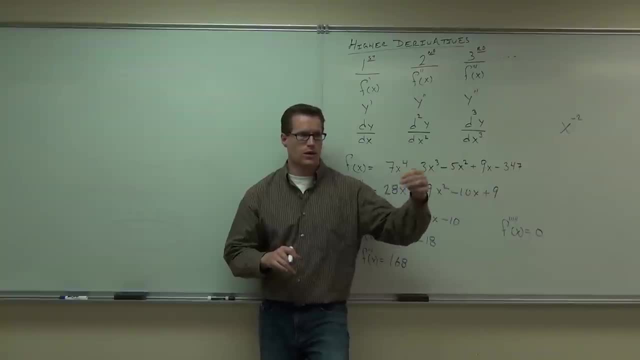 Then you get positive six x to the negative four, and then so on, and so on, and so on, And so that actually that exponent keeps on getting smaller, more and more and more negative. So this won't cycle out to zero eventually. 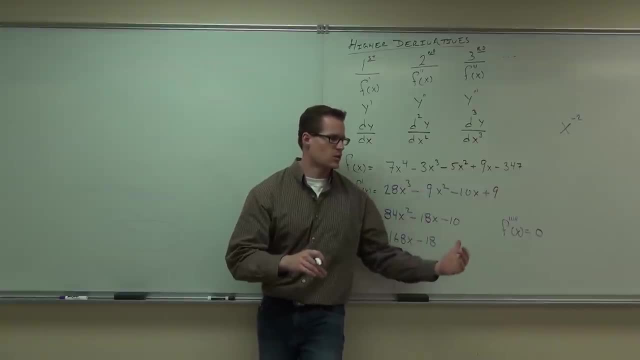 It's not a polynomial, So be careful on it. You're not always going to go to zero, but you can find more and more and more derivatives on this. How many people feel okay with our higher order derivatives? So it's basically just take a derivative. 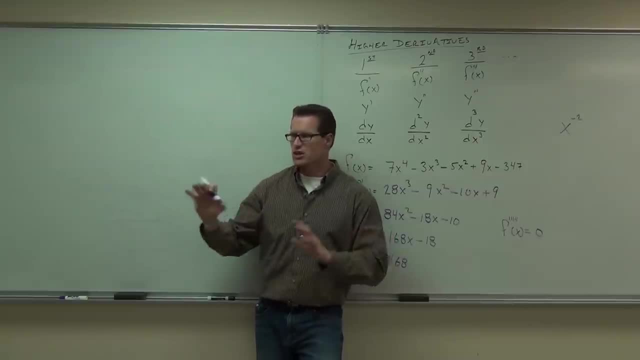 and then take it again, and again and again. That's what this is asking you to do. So what would really be the correct place? to stop? at 168, or when it reaches zero, Zero. This is all the higher derivatives, because every other derivative is going to be zero. 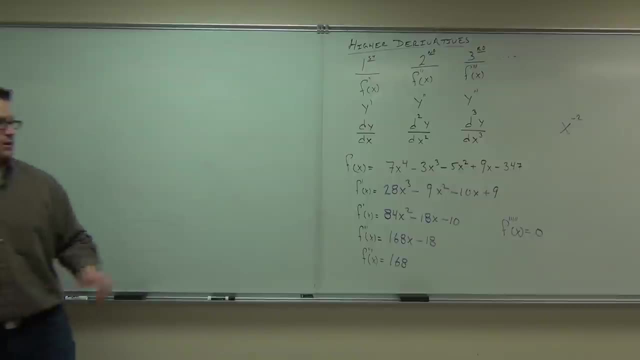 So zero counts as a derivative, Absolutely. Yeah, this, we've taken one, two, three, four, five, six, seven, eight. But then you can take this again and get something different, right, You can get five. 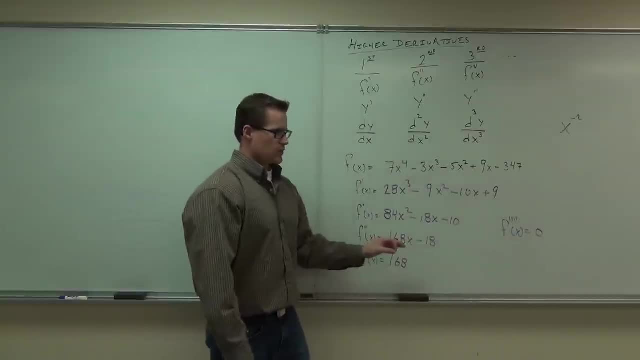 But then as soon as you take it to six, it's not doing. you can take them as many times as you want, You're just going to get the trivial answer of zero. after that, Yes. What if it was one over x squared? 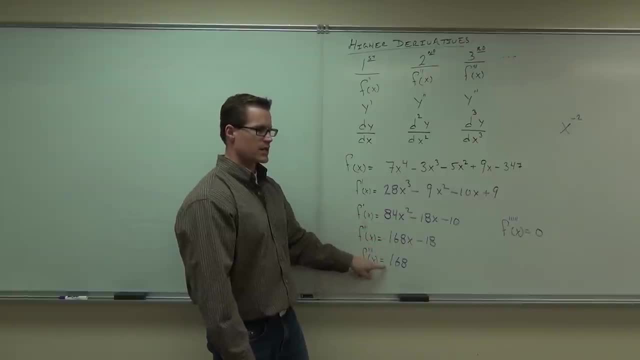 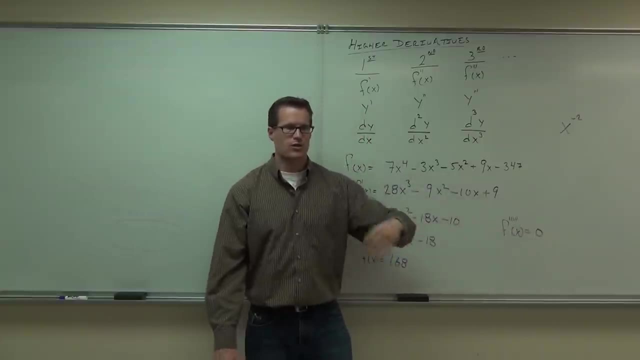 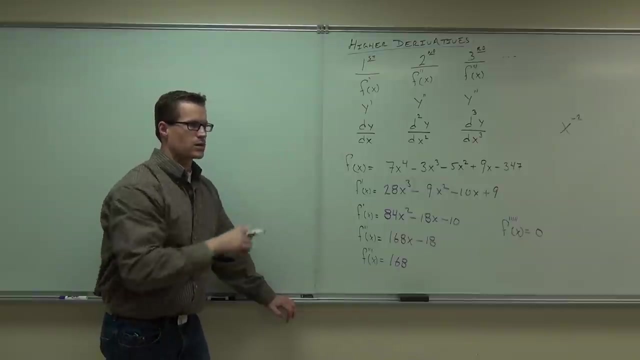 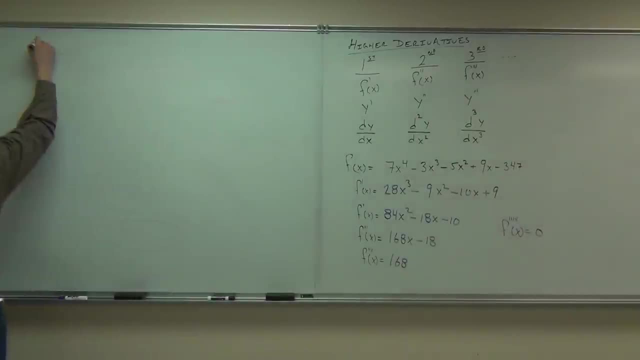 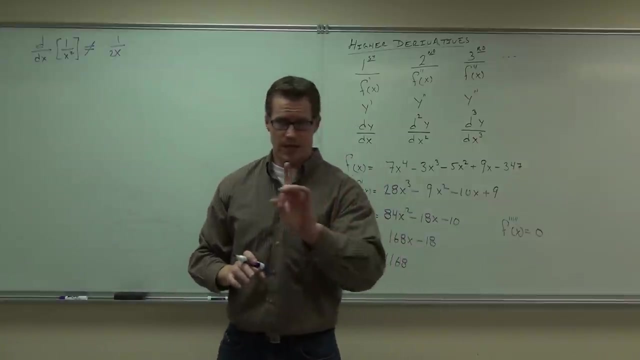 No, The derivative of this Is in no way one over two x At all. You're breaking the rules here. There's only one rule that we have. The one rule that we have is: it must fit this format, folks. It must fit this format. 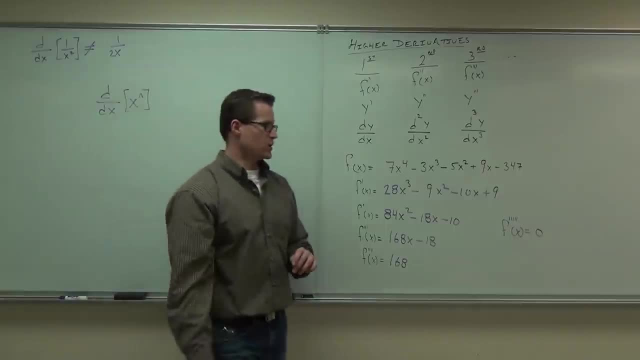 If it doesn't fit that format, you can't do it. That's it. to break it down in such a way that it does fit this format, All we can do is separate by addition, subtraction and pull out constants. So in order to make it fit this format, we can't just say: oh, 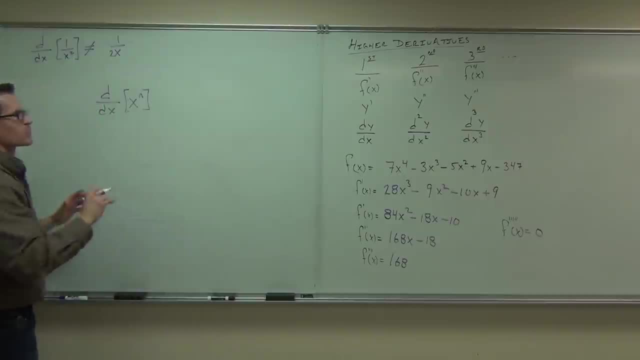 derivative of x squared is 2x. That would be awesome, but no, it doesn't work that way. Instead, you have to say: oh, this is the derivative of x to the negative 2.. That fits that format. Do you see the difference there? 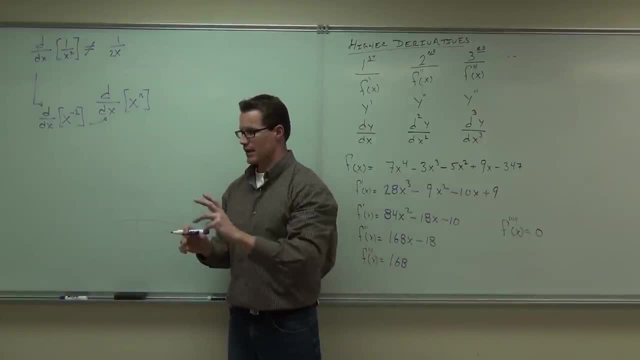 You have to make it fit that. So you have to pull that negative, that exponent up and make it a negative. That way you can work with your power rule. Does that clarify your question? Okay, so we can't just take derivatives of parts of, like quotients. 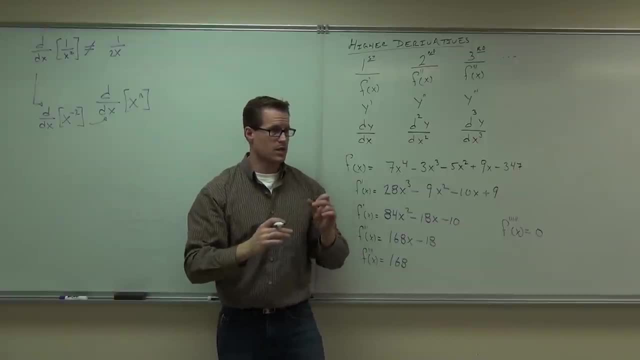 We can't take it to parts of products. We're going to talk about those things in just a little while, but you can't just do that. Are you with me on this? Would you like to see one more example? It might be good for you guys to see this one. 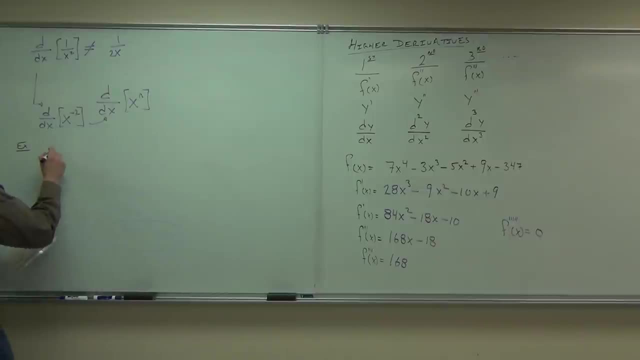 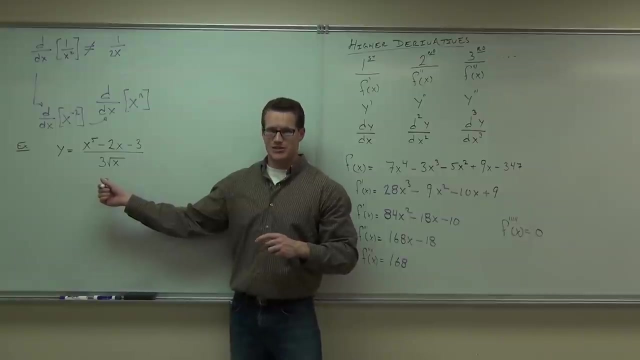 Could you take the derivative of all those things? Mm-hmm, Okay, Could you take the derivative of this thing? No, Got your head. Yes, you can, Yes, you can. Can you take a derivative altogether? No, not the way it is right now. 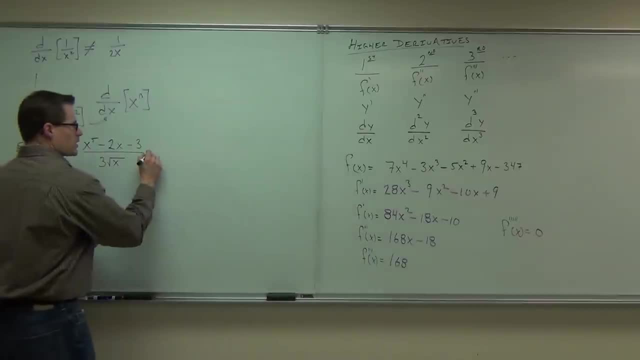 Let me show you a couple things about this problem. Number one: well, you probably are going to want to make this x to the 5th minus 2x, minus 3, all over 3x to the 1 half. Do you see what we did there? 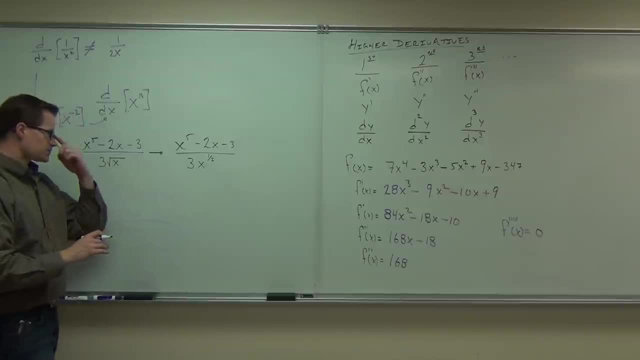 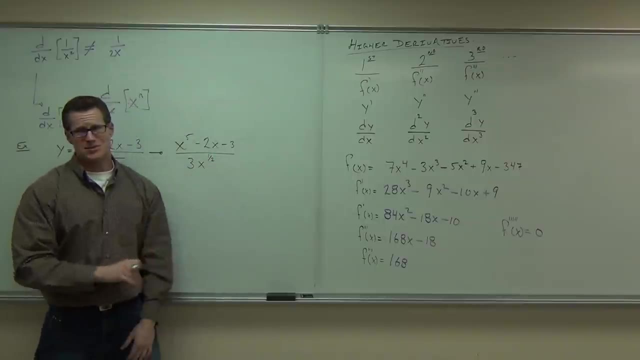 You okay with that? That's okay, That's great, That's fine, But here's what you can't do. This is going to go back to our previous problem: What you can't do, folks, you can't do this. 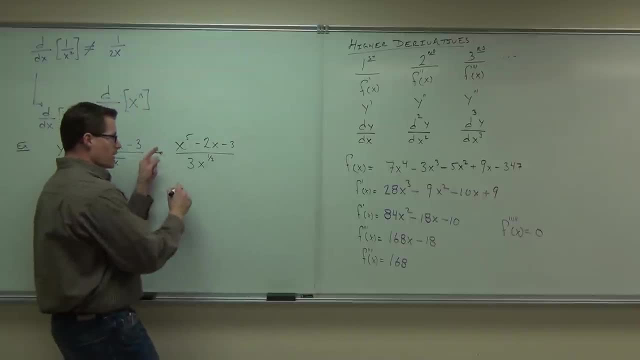 I wish you could, but you can't. You can't go. oh, you know what? This is: 5x to the 4th minus 2x over 3 half, x to the negative 1 half. Do you see what I did? 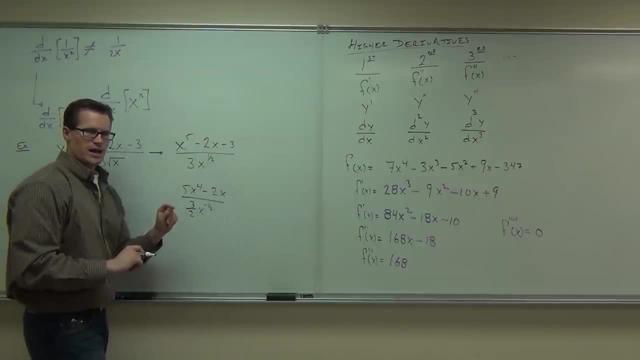 I took derivative derivative. derivative derivative. Can you do that? No, No, you can't. They're connected. They're in there in a quotient. We're going to find out later. you can't do that. You can't do that one. 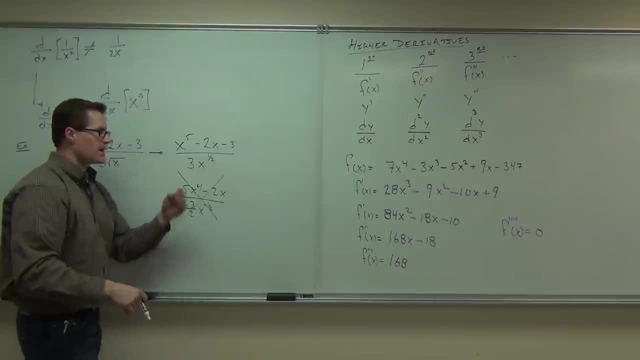 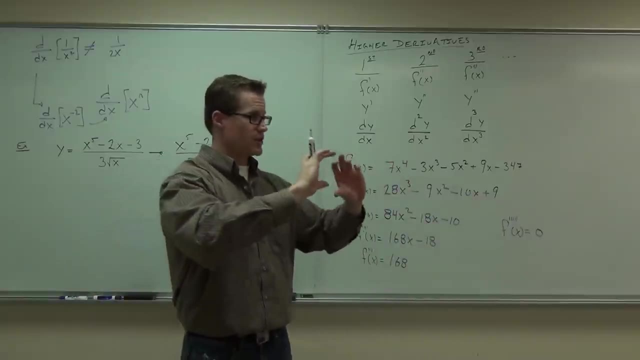 If you want to write that down, cross it out. If you wrote it down, cross it out. You can't just take it piece by piece. if they're connected, You have to be able to separate them completely and take a derivative term by term. 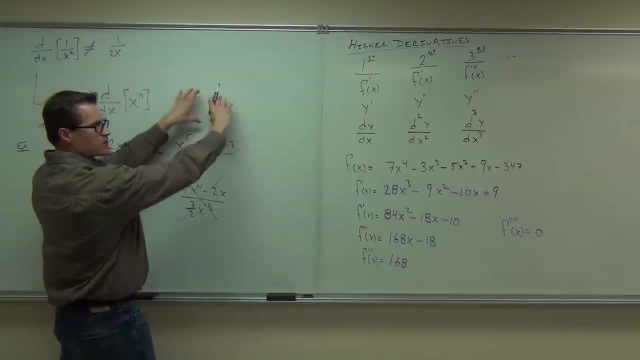 You can't do that here. You see, you can't separate this and have its own derivative minus its own derivative, minus its own derivative, and then have it over another derivative. That's something we can't do. We can't do that. 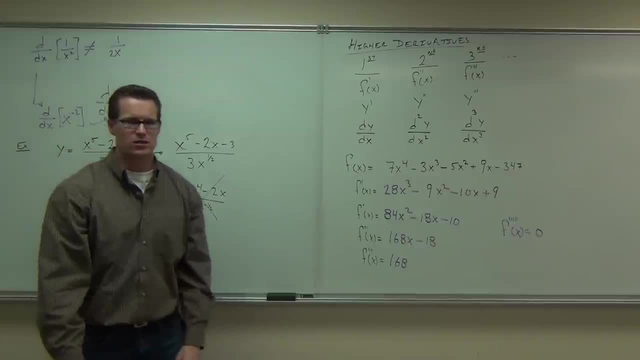 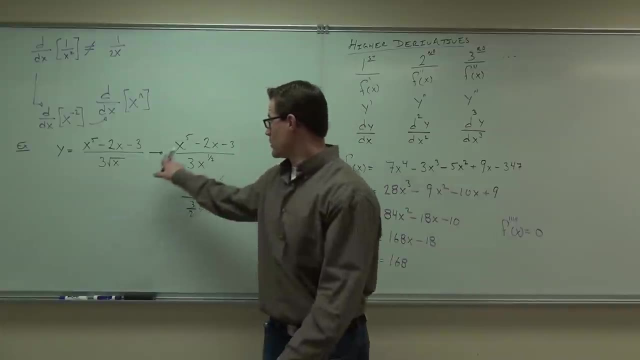 So what we would have? oh, give me another option. What could I do? Whenever I have some expression over one single term, what could I do? Move it up? I can't move that up. I don't want to do that. 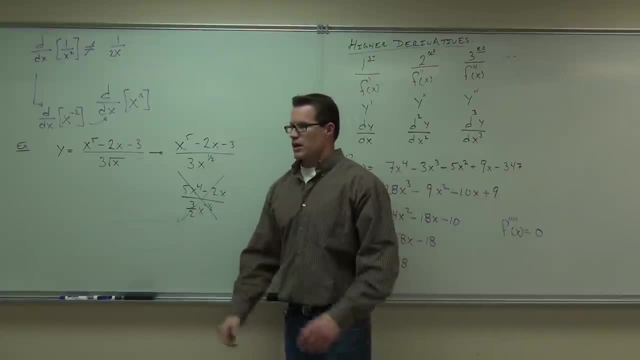 What can I do whenever I have several expressions, several terms over one single factor? Split it up. What now? Split it up over the- Let's split it up So sometimes these daunting looking derivatives that you need to do. what would happen if I did split this? 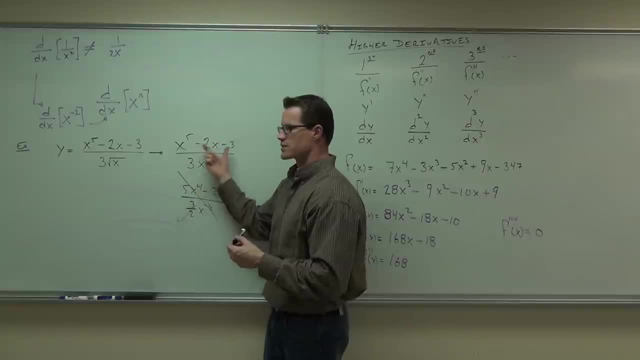 up as x to the fifth, over this, minus 2x over this, 3 over that. Let's see what happens there. Then maybe we'll make it fit into our equation, Maybe we'll make it fit into our scenario that we can work with. 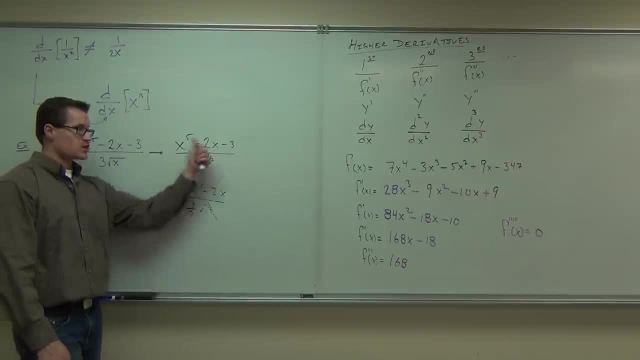 Firstly, are you okay that this doesn't work? as a matter of fact, You can't just take all these pieces if we have a quotient or a product or something crazy. The only time we ever found out that that did work was this. 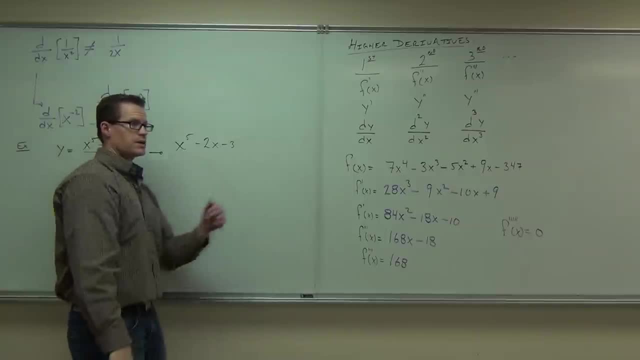 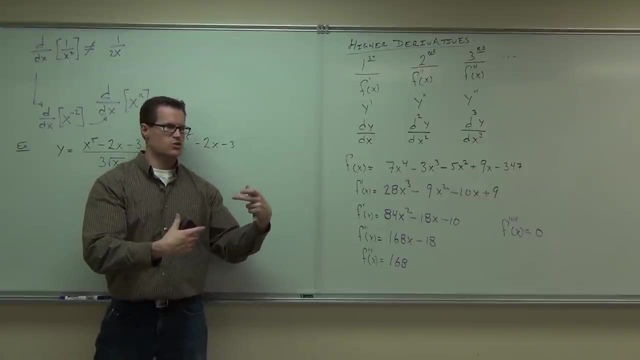 Look When I had a polynomial: yes, that works, Because I can separate by addition and subtraction. that's what makes that work. I didn't tell you you can separate by division, because you can't. I didn't tell you you can separate by multiplication. 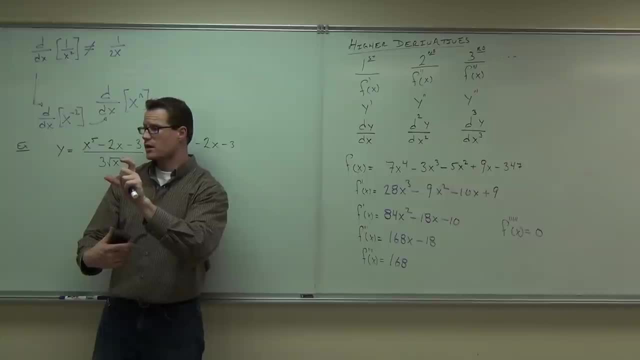 because you can't unless you have the constant that comes out. That's the only way, That's the only thing. So you can't separate by division. You can't do that. Only thing you can separate is addition and subtraction. You follow me on this. 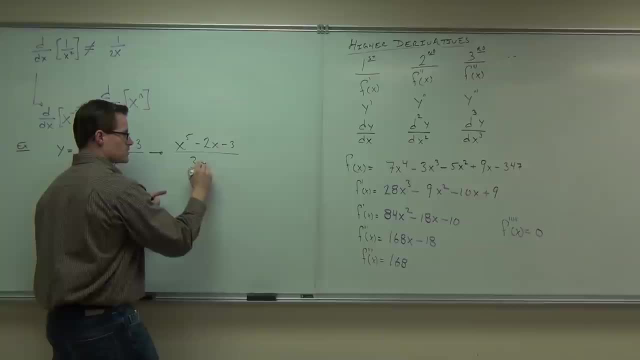 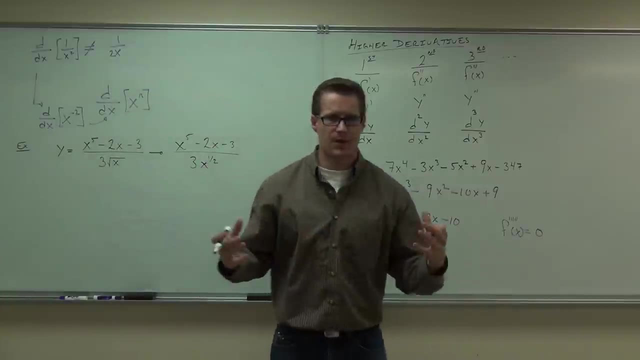 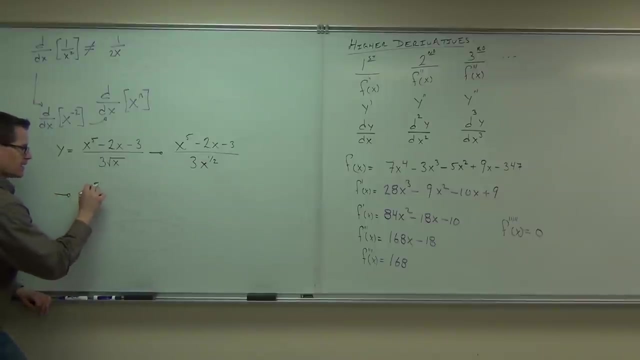 So, when I translate this into 3x to the 1 half, we've got to have something better than this, this, this over that. that doesn't work. What we could do is potentially split these up into three different fractions. So, for instance, why don't we try to make it x to the fifth? 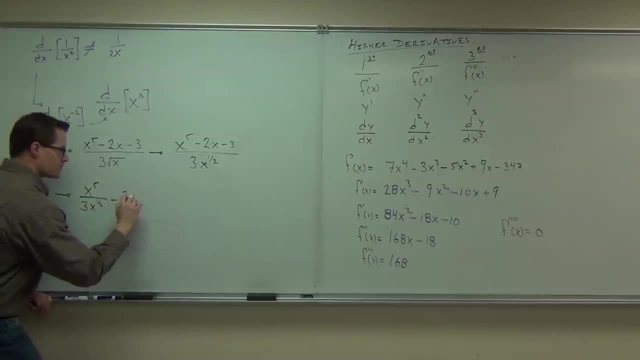 over 3x to the 1 half, minus 2 over 3x to the 1 half minus 3 over 3x to the 1 half. And then we'll try to simplify each of those fractions to make them fit in our power rule. 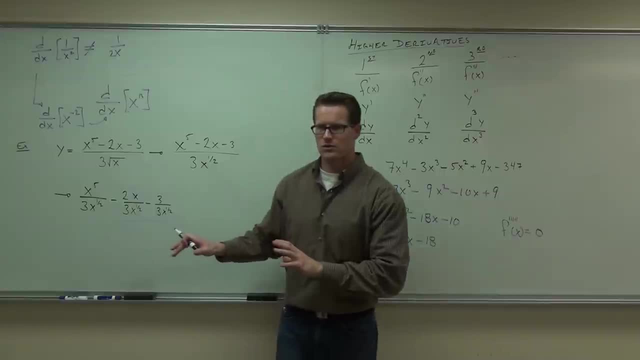 and then take the derivative. Are you guys all right with what we're doing so far? We're trying to make it fit into this. We have to make it fit there. If we can't make it fit there, we can't take the derivative right now. 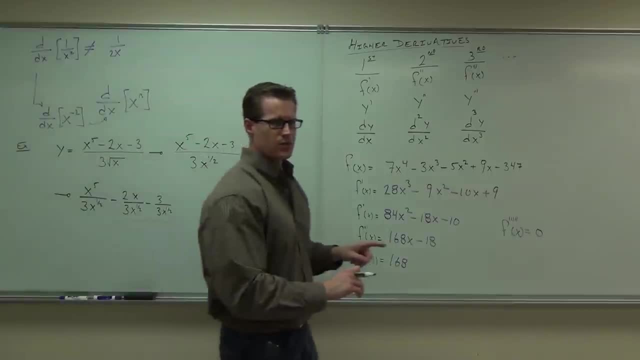 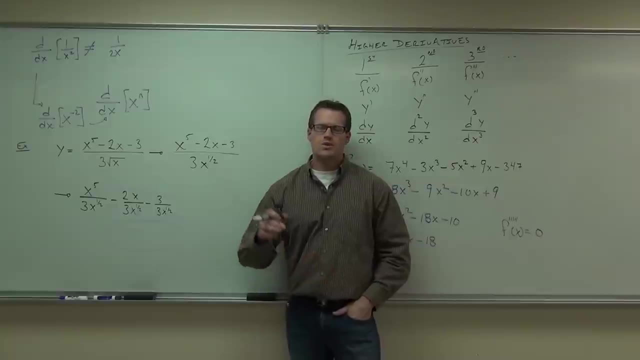 Can you combine those x to the fifth and x to the 1 half? How do you do that? Okay, what happens when you have common bases that are being divided? Do you add exponents, subtract exponents, multiply exponents or divide exponents? 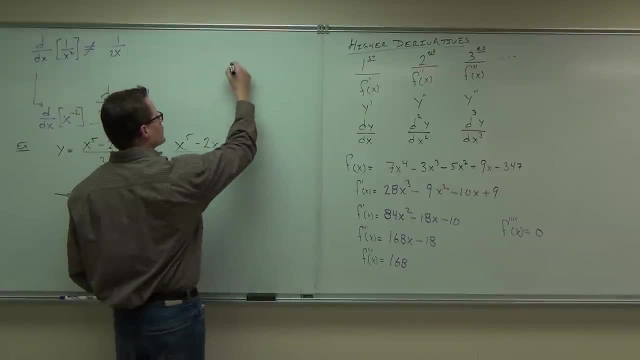 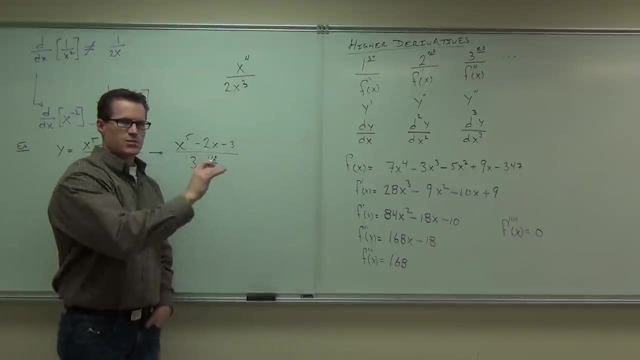 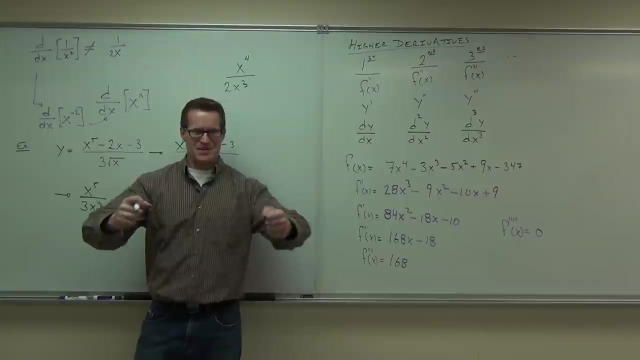 Let me break it down even easier for you. Okay, watch, No, just watch. Can you simplify that? Yeah, Please, goodness, say yes. Please say yes, Mr President. Mr President, I know how to I'm supposed to be in this class. 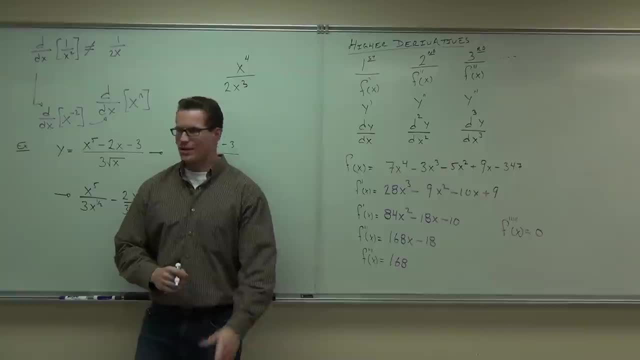 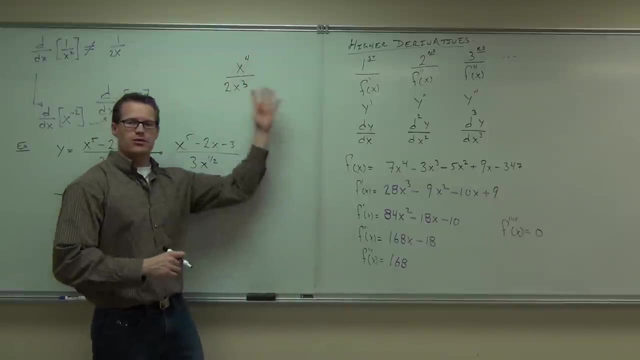 How do you simplify this? What is it? What is it Subtract? You subtract what Subtract? your exponents. because when you divide exponents, you have four of them here, You have three of them there. You cross out three of them. you have one of them left right. 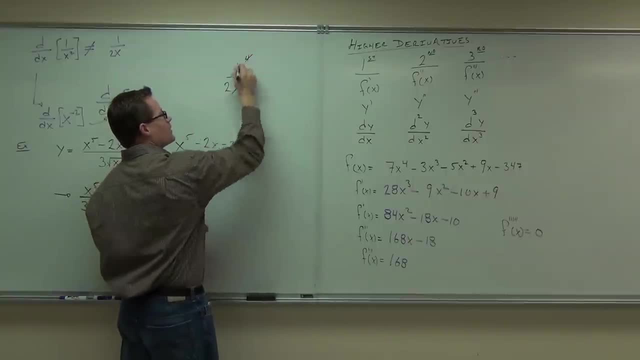 That's subtracting exponents. You go- oh yes, this is completely gone. That becomes an x. What happens to the two? Go on the top, stay on the bottom. So you would have x over 2, true. 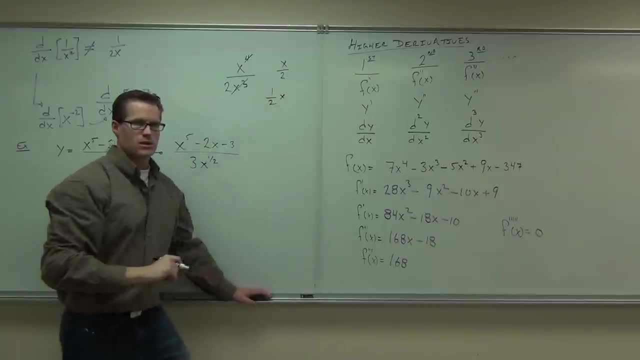 Or you could get 1 half x. Do you follow? Okay, so you know, whenever you have common bases, you subtract exponents. This is not a hard concept. You've seen this since your algebra. beginning algebra days. beginning algebra days. 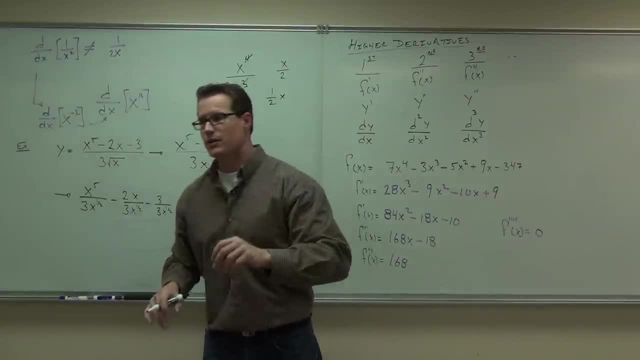 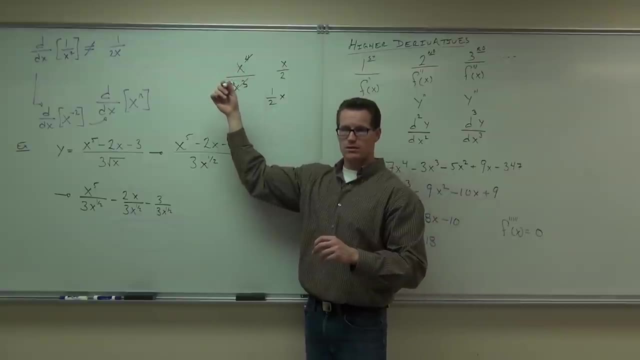 So can you combine these? The answer is: what? How do you combine those? How did you combine those? Subtract? what Subtract your exponents? What's 5 minus 1 half? How much are you going to get? 4 1 half? 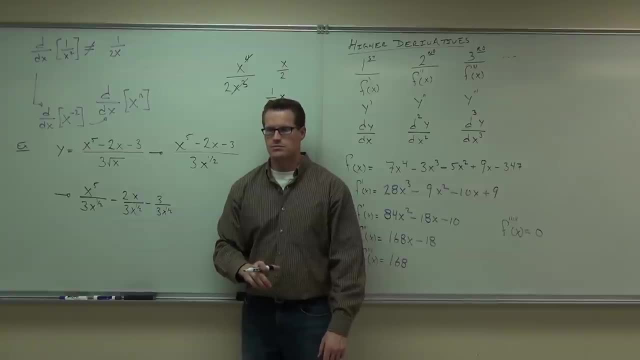 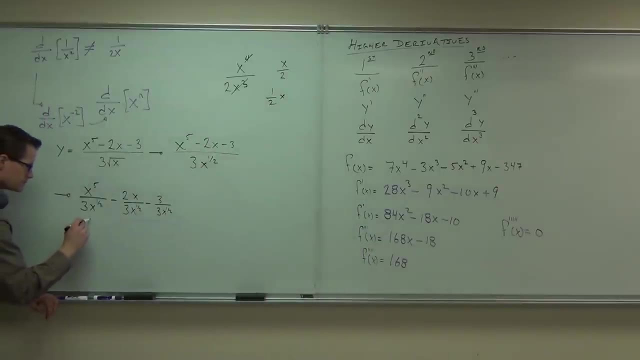 Give it to me. It's an improper fraction: 9 1 half. 9 1 half. Really, I didn't do it in my head. Yeah, 9 1 half. I need you to be able to get there. 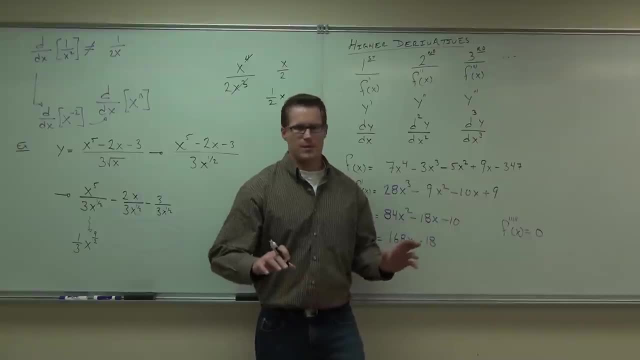 That's not calculus. Okay, that's algebra. This, right here, I mean, people have said, before you take calculus to finally fail algebra. don't let that be. you know your algebra. if you know your algebra, this is a piece of cake. I mean really honestly, calculus is easy if 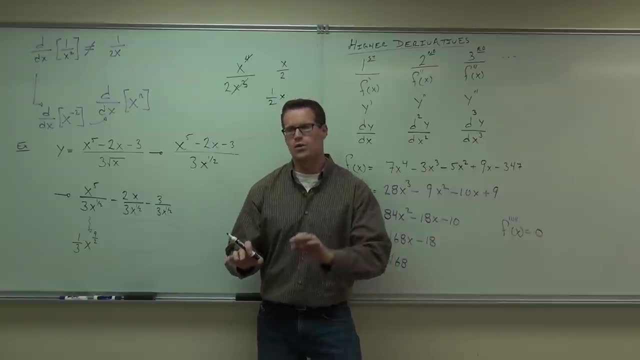 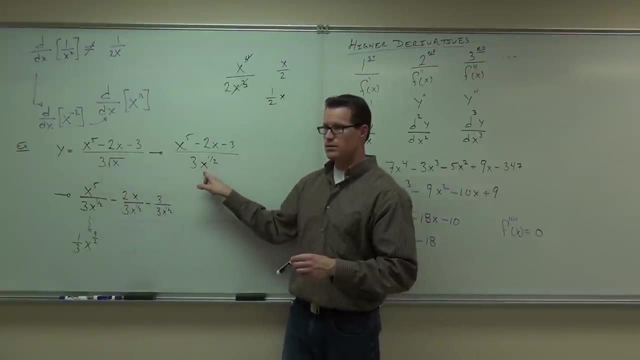 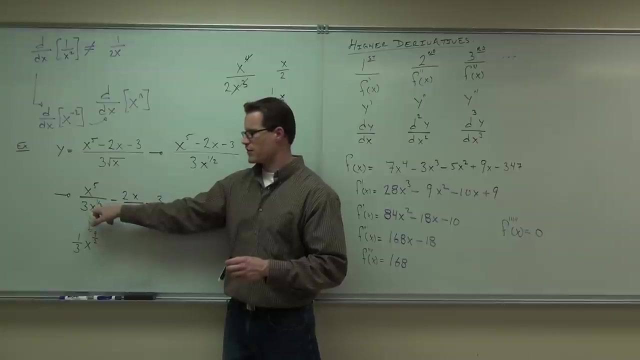 you know your algebra, promise and trigonometry? if you don't, yeah, it's gonna hold you back a lot. are you okay on, firstly, going from here to here, secondly, going from here to splitting them up and now, thirdly, do you see how to get from the X to the fifth, over X to the one-half into one-third X to the? 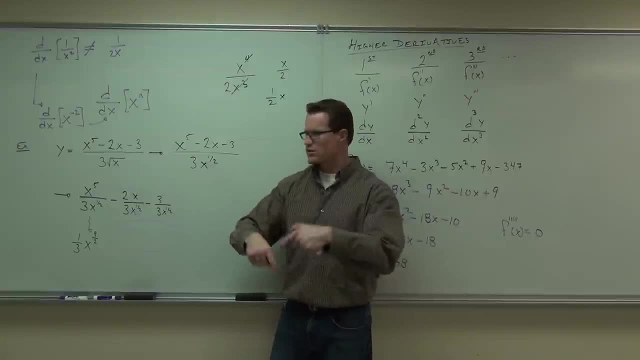 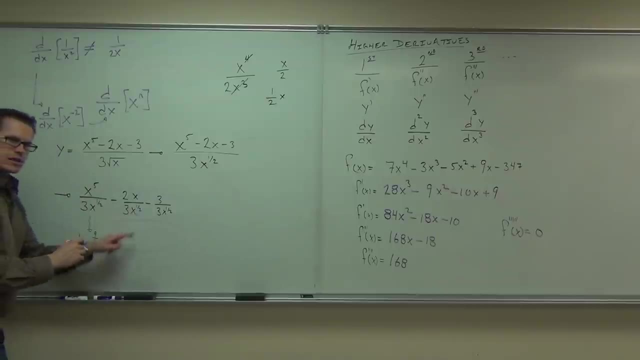 nine-halves. we're subtracting those two exponents. do that and calculate. if you want to. five minus a half, you can get four and a half or nine halves minus. let's look at those numbers. that's gonna give me two-thirds X over X to the. 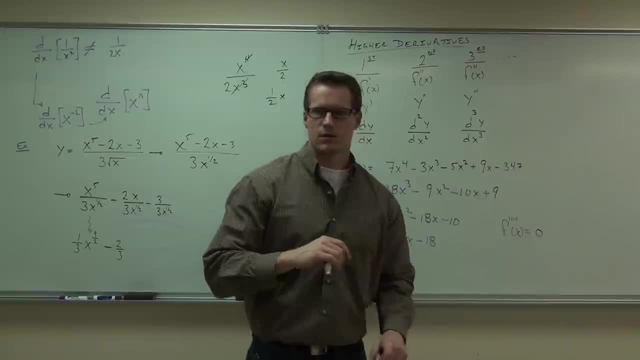 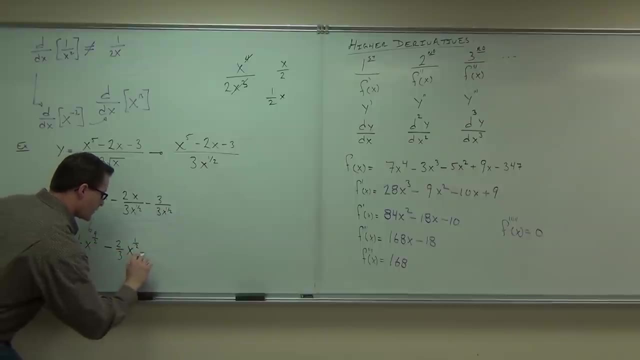 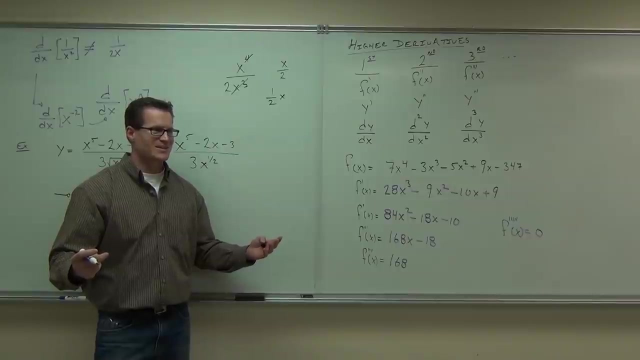 one-half. gives you what? please one half good, because you subtract one minus one half and get X to the one half minus. oh, what's that become? this is supposed to be a new video. you have that old-school ringtone on. come on, give me some 50-cent or so. that's even old too. what's new? I'm on the edge give. 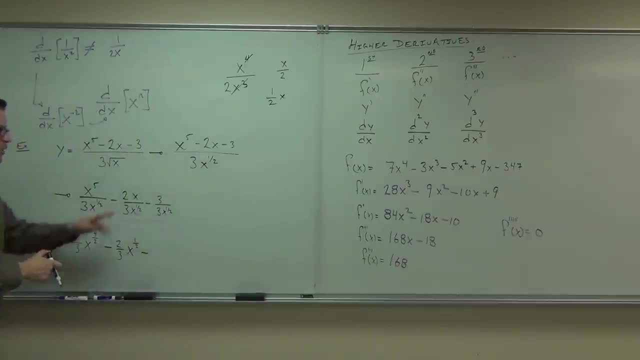 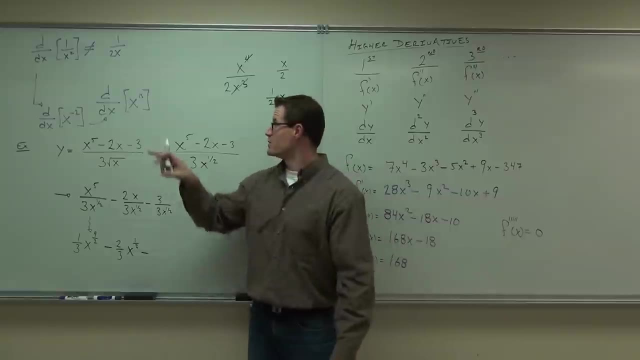 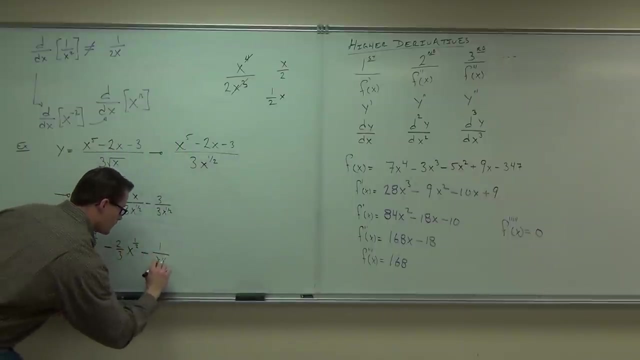 me that one next time. all right, thanks. what happens to the threes? they become a one. what happens to the X, to the one-half? what are you gonna have to do with that in order to make it fit that? what do you do? can you leave it like this and take through? that would be the scenario that 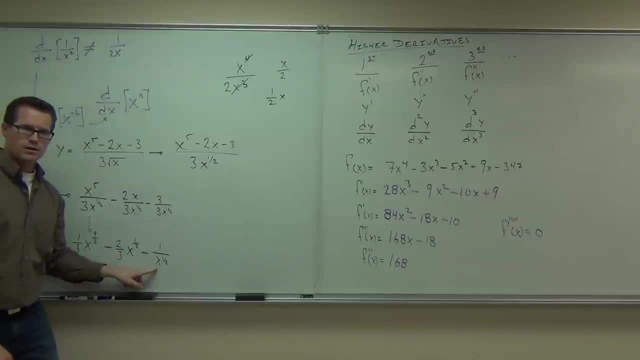 would be that scenario. what do you have to do to the one-half? so we're gonna have to move that to the numerator and make it a negative one-half. do you follow me? you're constantly trying to make it just look like that. that's what you need, so. 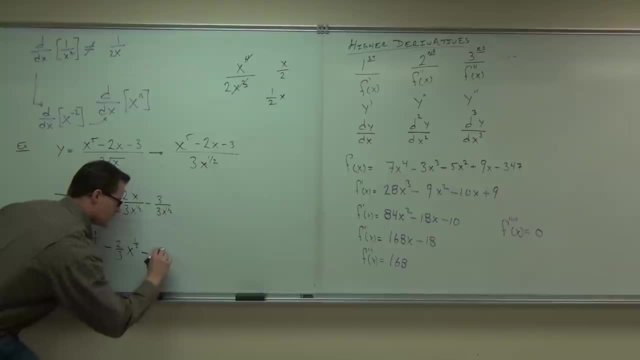 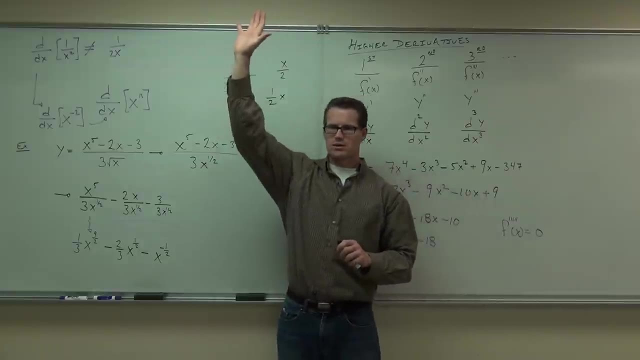 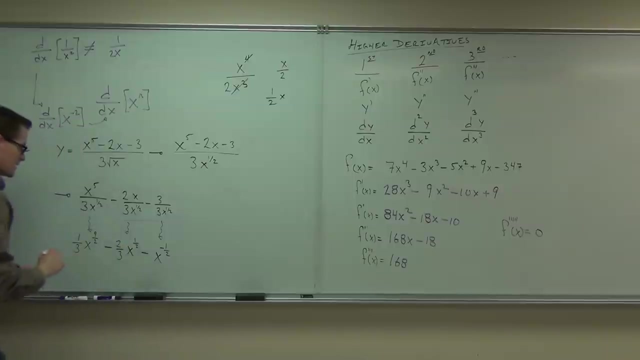 one over. X to the one-half, no, X to the negative, one-half, yes, yes, show of hands. how many people feel okay with this? so far, simple algebra, good, all right. some of youAn州 noodle now that why? this is still. I haven't even ducked you notice. I haven't done. 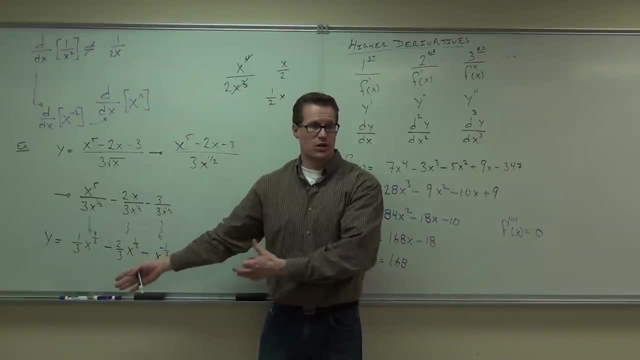 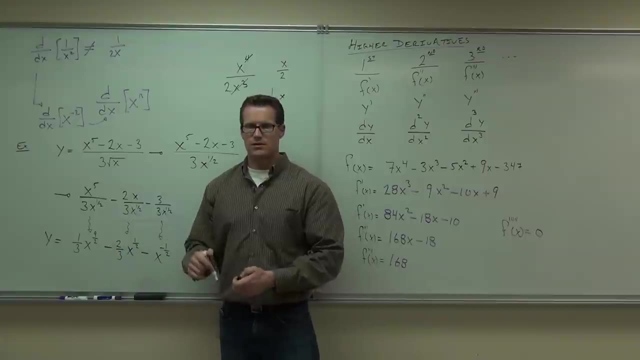 calculus, yet no calculus, yet. this is base, just algebra. now, can you do the calculus? can you take a derivative? why don't you carefully, right now, take me that derivative. got to do that carefully. take a derivative. I'd rather have the go slowly on, by the way, i want. 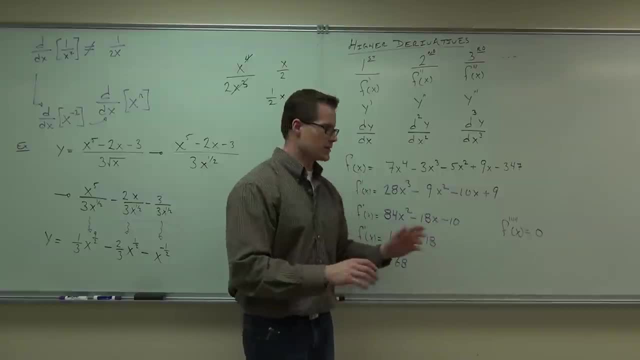 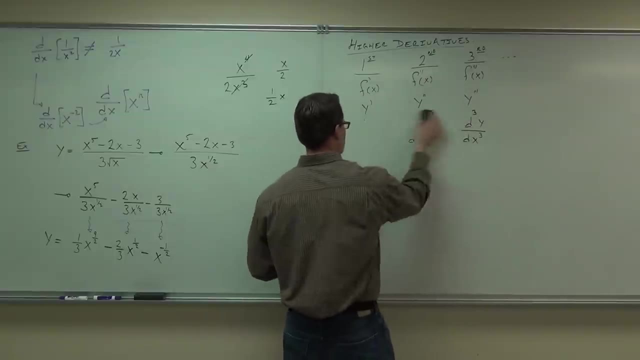 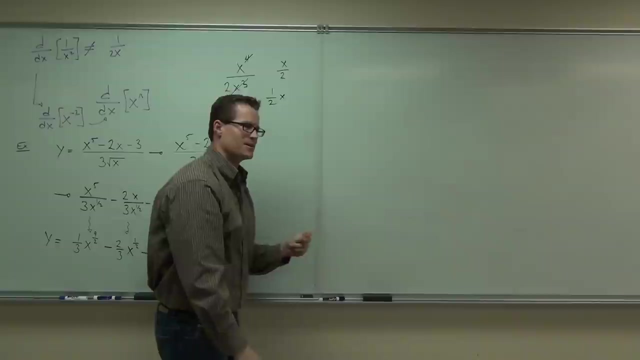 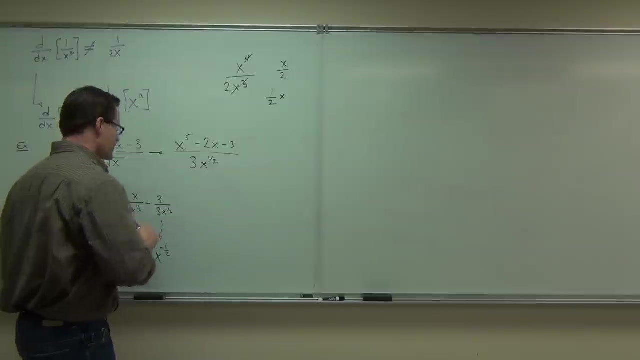 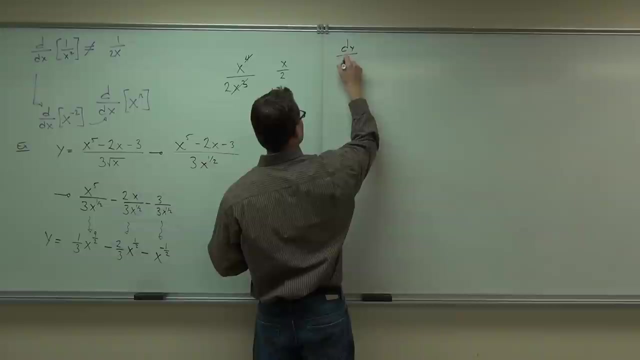 the correct answer rather than the wrong answer quickly. that would be stupid. Was that Lady Gugu, by the way? That lady, Yeah, Is that not right? That was perfect. So dy to the x or y prime if you'd like. 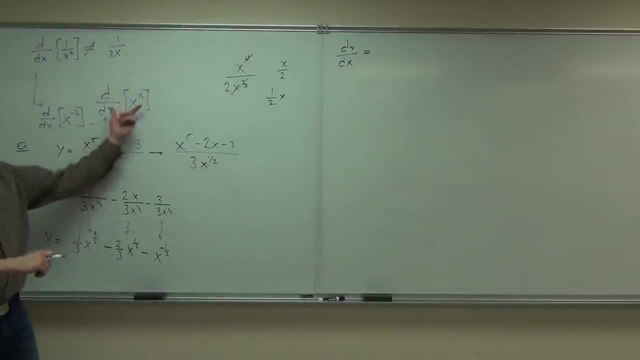 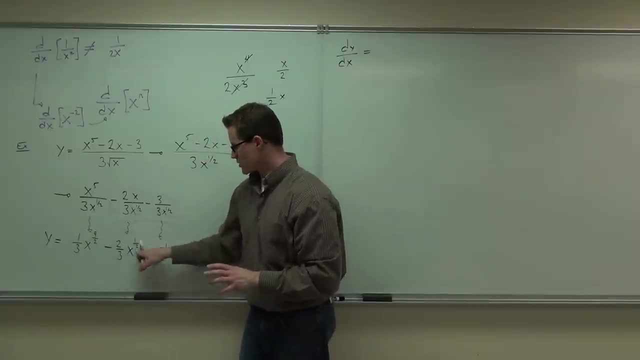 Note how each of these now fits into our format. here The constants: we could pull them out. We're just taking a derivative of x to the 9 halves, derivative of x to the 1 half, derivative of x to the negative 1 half. 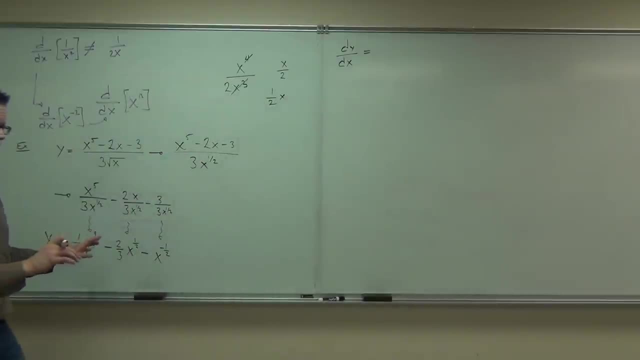 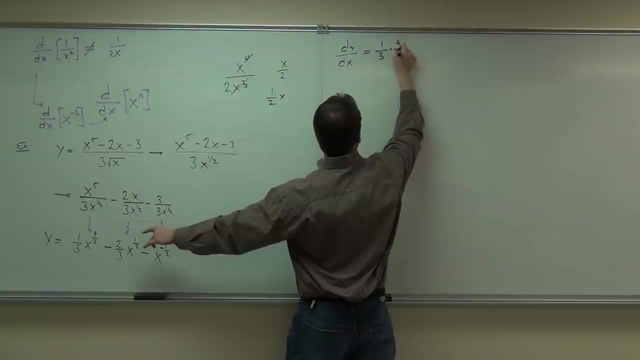 Let's do that piece by piece. I'm going to show you every step. okay, right now, so you see where it's coming from. I'll have the 1, third times the 9 halves. Do you see where the 9 halves is coming from, ladies and gentlemen? 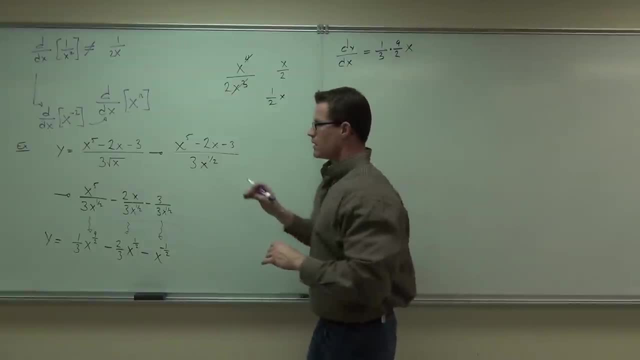 Okay, I'm going to have x to the. I need to do 9 halves minus 1.. That's going to give me 7 halves. Did you get 7 halves as well? Perfect, 7 halves. Get that one. 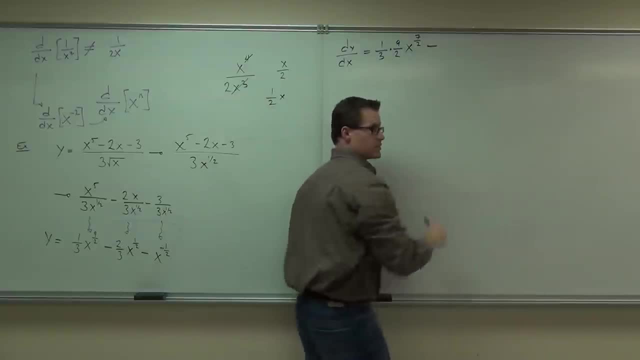 Next up, I'm going to have minus, minus 2 thirds. 2 thirds times what, folks? Okay, 1 half, because that's my exponent that I'm bringing down, So I leave my constant alone. I'm multiplying by my exponent. 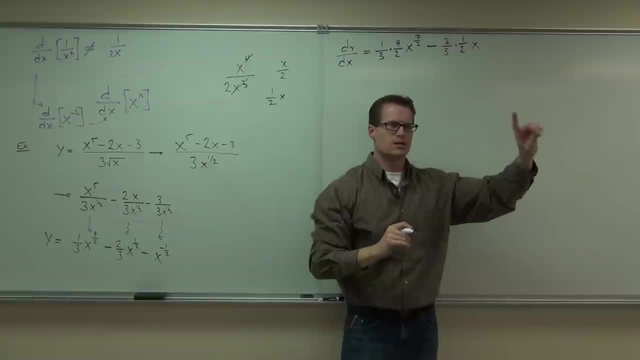 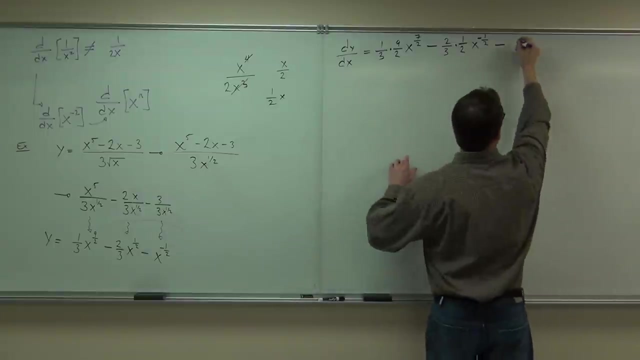 and then I'm going to take x to the 1 half minus 1, gives you what? Lastly, I have minus minus What? now? Negative 1 half times negative 1 half Okay. negative 1 half, Okay, great. 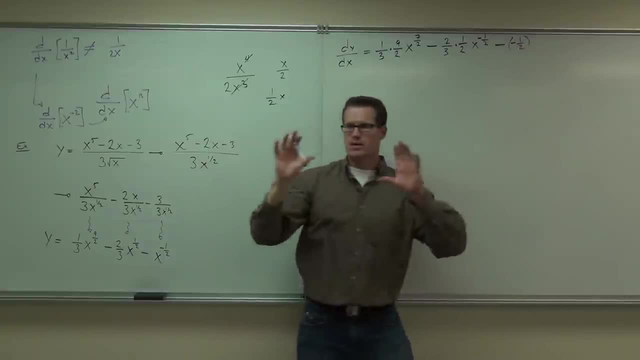 So negative 1 half. I'm going to put that in parentheses, saying hey, I'm a negative, Watch out, I have a negative there. So minus is minus, Negative. that's our negative. x to the Okay, x to the. 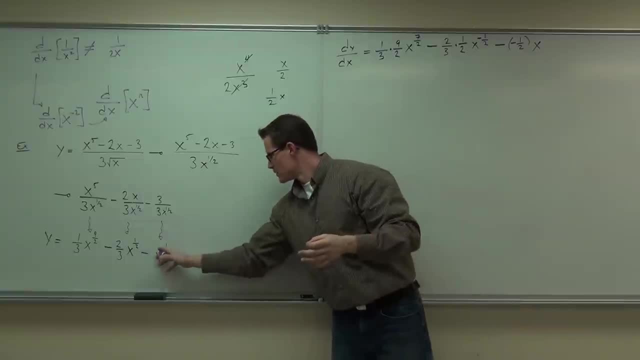 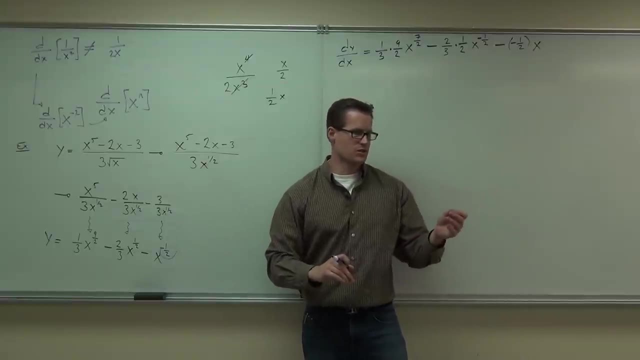 What am I going to get? Negative 3 halves. Negative 3 halves Because I had negative 1 and a half, or negative 3 halves. right, We're using proper fractions here because they're easier to deal with. So negative 1 half minus 1 half. 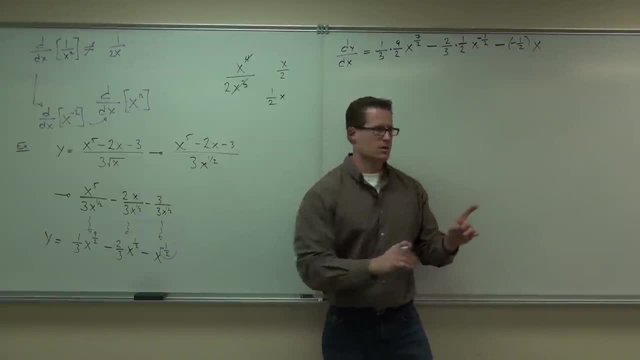 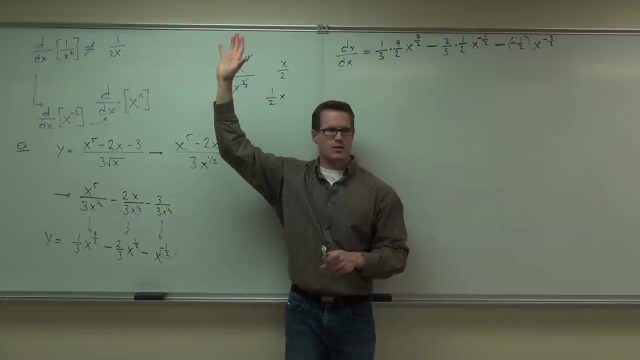 Negative 1 half minus 1 gives you negative 3 halves. You got that one. Yes, Show of hands. how many of you feel okay with getting that far on our problem? Let's make it a little bit prettier. Simplify some fractions. 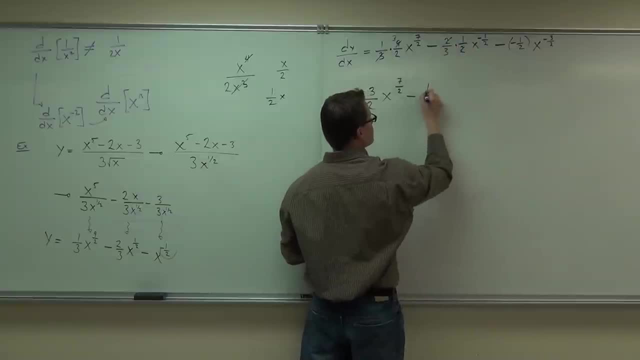 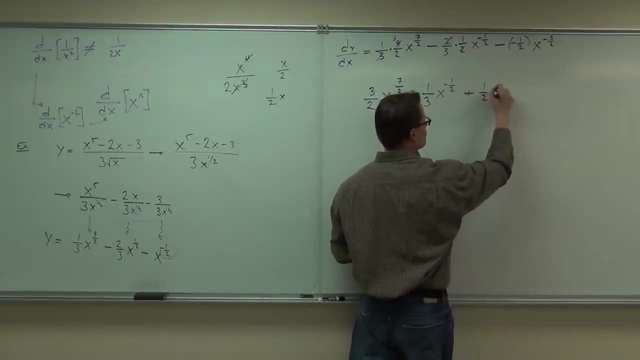 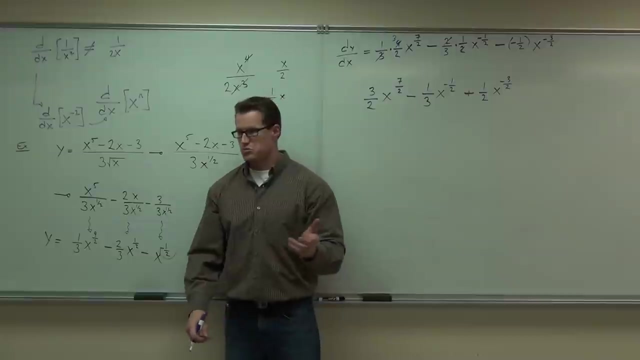 That's 1., That's 2., That's 2.. There's a third one, In the most basic sense, that's your derivative. No problem, What did I just find? What is that that we found? Oh, come on. 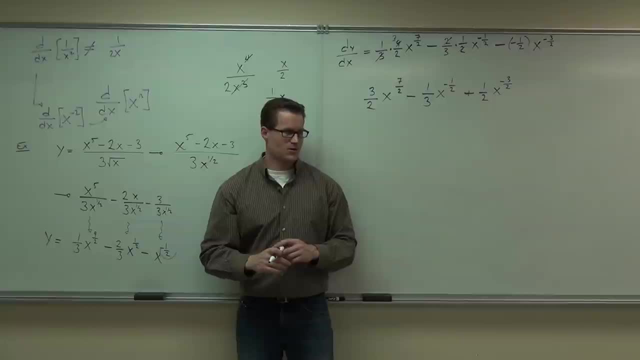 what is it? What's the derivative Slope of a curve, out of this curve, this weird curve at any point, at any point. It's kind of neat that we're able to find that right. We don't even know what that looks like. 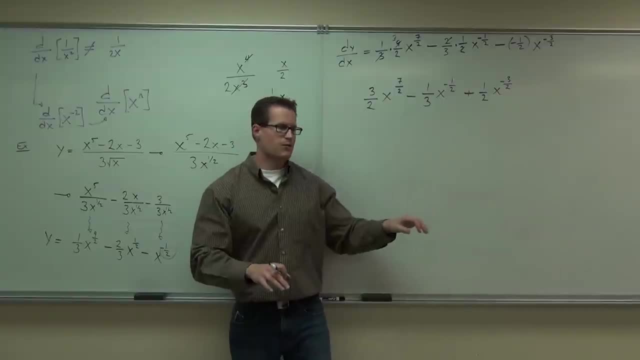 yet we're able to find the slope of that. at any point, We have a function for it. Now, if you do want to make this a little bit nicer looking, you can translate these back into roots if you really so desire. You could do. 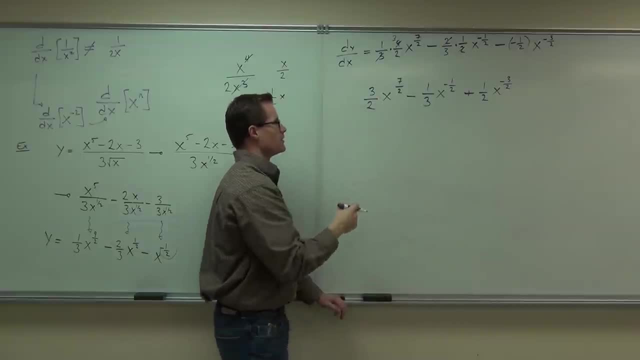 well, I probably wouldn't change that one at all, unless you want to do a square root of x to the seventh. that's what that means. So if you really are forced to do it, here's how you would change this back into roots. 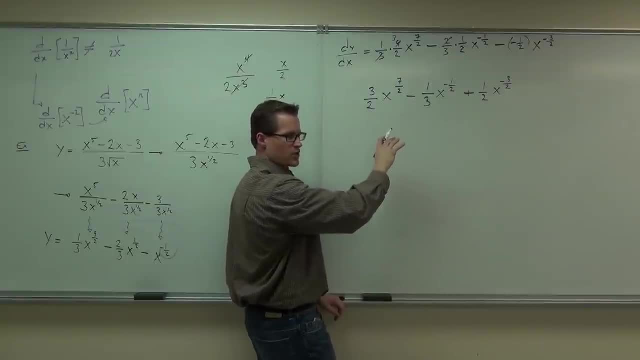 For me, most of the time that's going to be fine, but if you're forced to plug numbers in, you want to see what's actually going on here. So this would be three square root x to the seventh, over two Minus, since that's a negative. 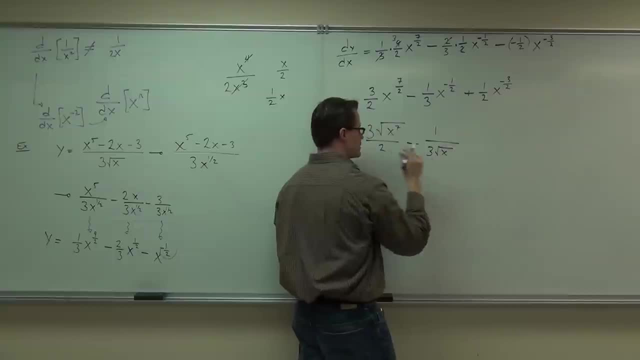 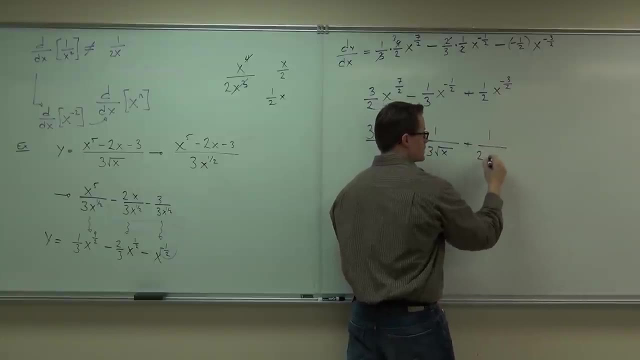 it will be on the denominator of a fraction: three square root of x. Since that's a negative exponent, it will be on the denominator of a fraction along with that: two a square root of x. cubed, That's the way you would write that. 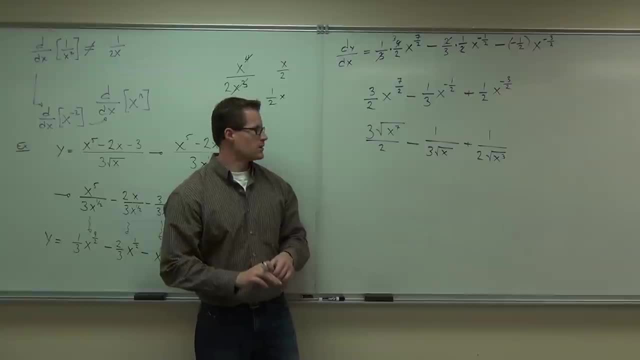 without any negative exponents. That's the way you would write that: without any negative exponents associated with that. Most of the time, we're going to be okay on that. However, typically if they get root form, you want to make it back into root form. 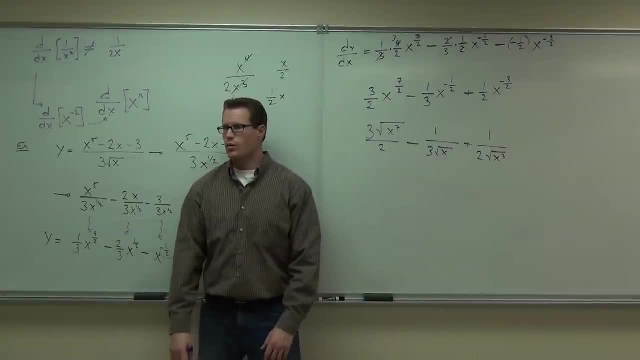 So in that case that would be maybe what you see in the back of your book or some other context. Some people feel okay with our example up here, So can we do this term by term, by term by term? Can we do that?